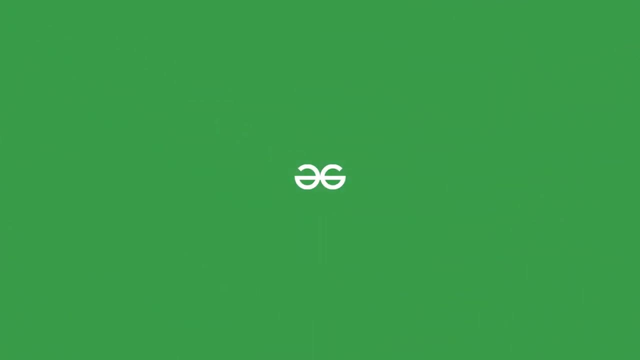 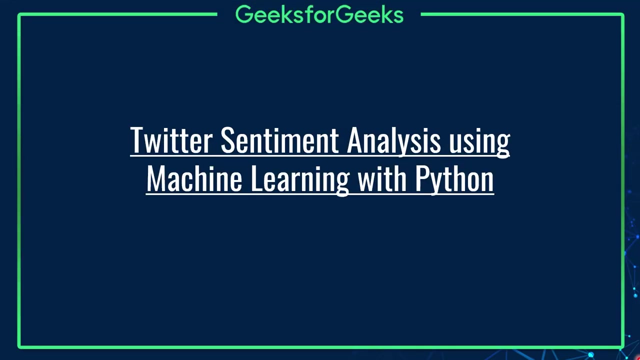 Hello everyone, the machine learning use case that we are going to discuss today is Twitter sentiment analysis using machine learning with python. So in this use case, we will be training our machine learning model with loads of twitter data. So in this case, the twitter data is: 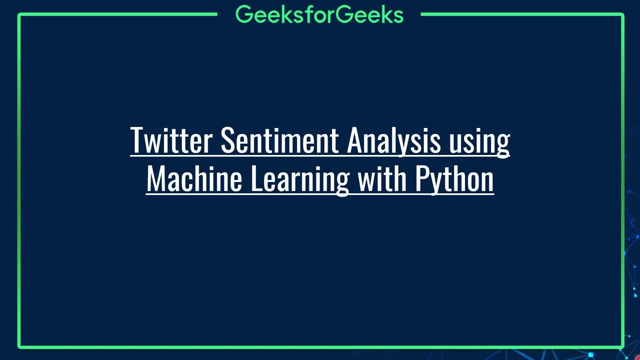 nothing but the tweets that we have, and once we train our ML model, this model can understand whether a tweet is a positive tweet or it is a negative tweet. In other words, it can understand whether a person has tweeted it with some positive intentions or negative intentions. 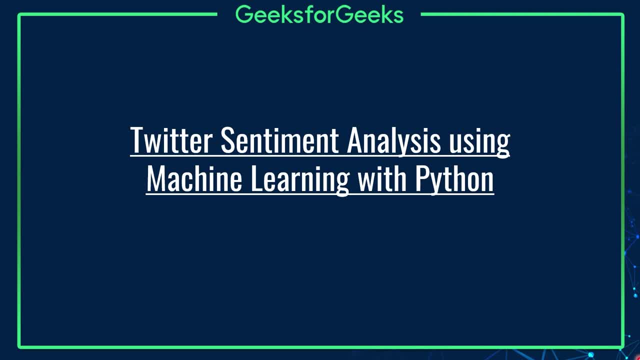 So that will be the agenda for today's video, and let's get started. So, before going into the coding part in python, let's try to understand what is the workflow that we are going to follow for this particular project, and the first thing is data collection. So first we have to collect this tweet. 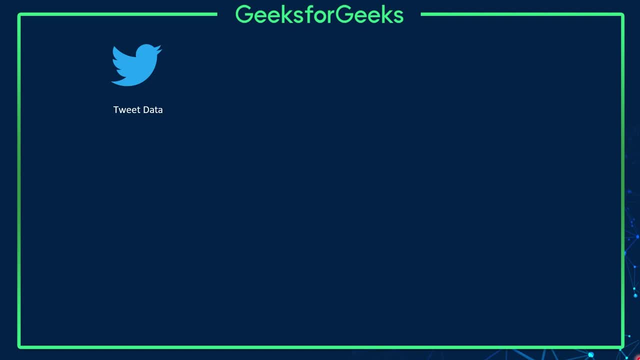 data and once we collect this tweet data, we have to process this. So, as we know that these tweets are nothing but textual data, right, and we cannot feed this textual data directly to our machine learning models. So machine learning models cannot understand this textual data, but they can understand numerical data. So we have to find 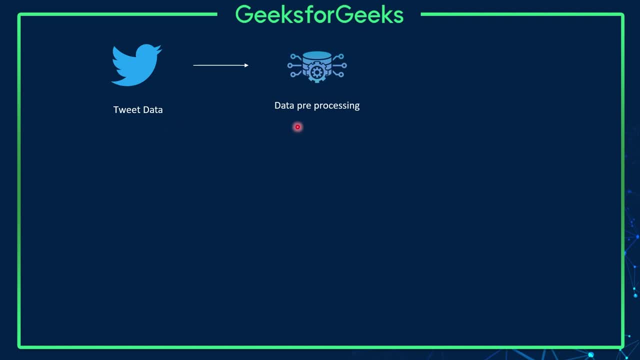 a way in which we can efficiently convert this textual data into numerical data, and that will be done in this data pre-processing part. and once we do this data pre-processing, we will split our data into training data and test data, and this part of the code is called as train test split. 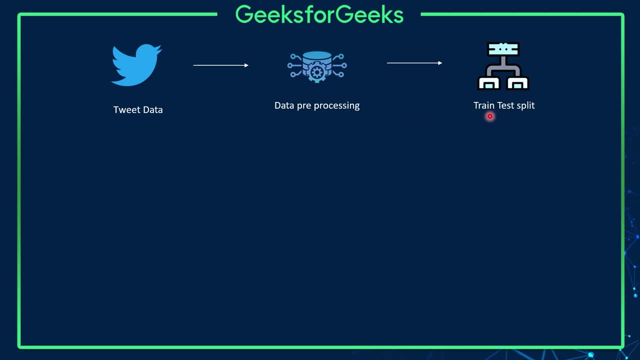 So train test split is a training model that we use to train our machine learning model, and the test data set that we have is used to evaluate our model. Evaluate in the sense we have to find what is the accuracy of the model and how the model is performing and so on. So that is why we are 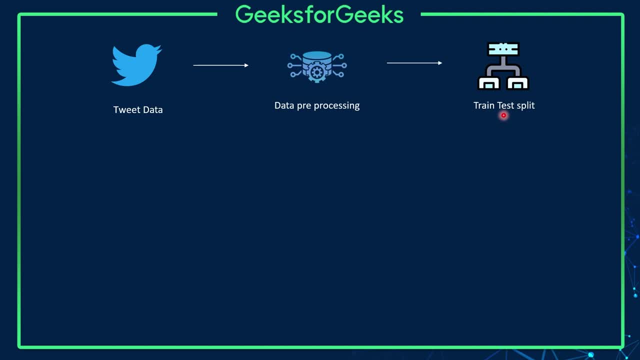 splitting our data into training data and test data, and after this step, we have to feed this training data to our machine learning model and in this case, we will be using a logistic regression model, as this is a classification problem, where we are classifying the tweets to positive tweets or negative tweets. Okay so, once we train our machine learning model, 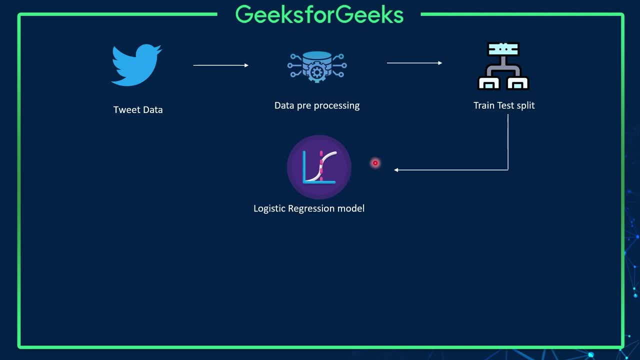 we will evaluate it using this test data. So, after this, we have this trained logistic regression model and once you have this trained model, if you feed a new tweet to this model, it can say whether that tweet is a positive tweet or a negative tweet, which is our final prediction. 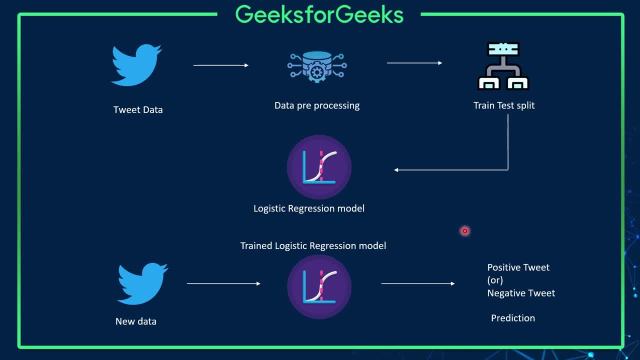 Okay, so this is what we are going to do in python: from this data collection all the way to training this machine learning model and using this trained model in order to do some predictions. Okay so, let us get started with the python part of this video. So I will be doing a. 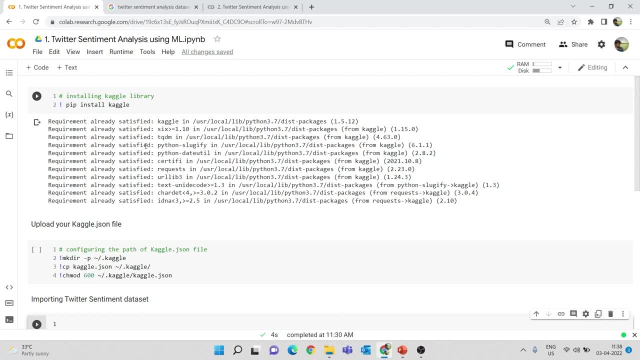 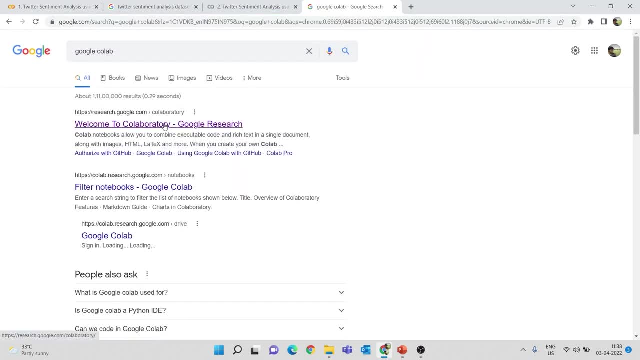 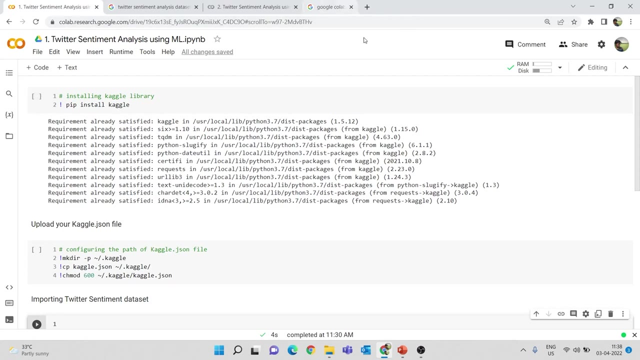 very specific placement and look, you know we are lightest content. many people think about this, But see that between weeks I have 100 thousand. I am trying to build a very large énumeration pace, a warrior course, to test my programming in order to know the month of that month and say correct stage. if that news goes down, what? 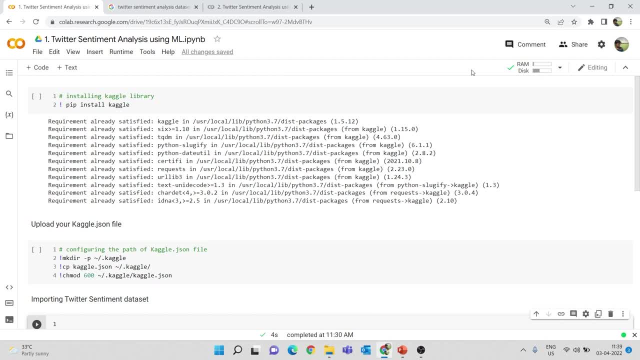 I would call your End. when I open a number, I will be asking you random questions. There is- there will be, an option called disconnect where you can connect your system. okay, so all these are like: uh, these python codes are executed in cloud, in google's backend server, so you don't. 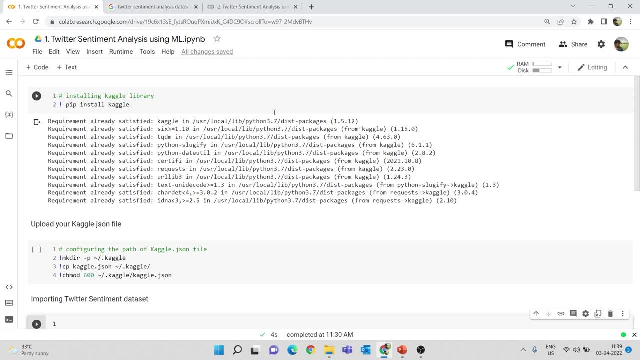 need to install any softwares or anything. so this is like completely free for your- uh, you know, machine learning use cases and data science use cases, so you can actually use google collab itself. you don't need to install any ids or notebooks. okay, so this is where we'll be doing all our 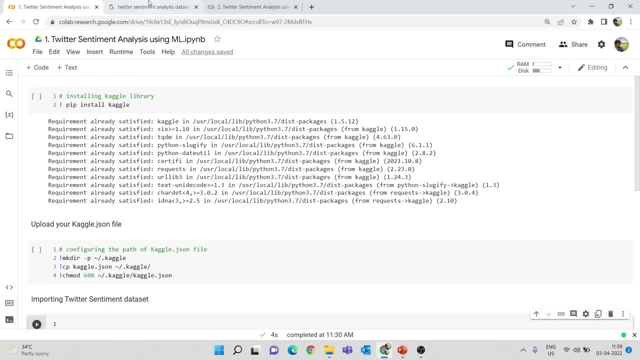 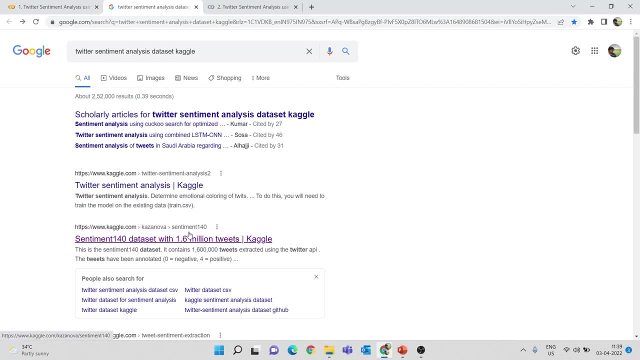 programming. so the next part of this video is to you know do this data collection, so where we are going to get this data. so in kaggle we have this uh sentiment analysis data set, which is you know we are going to use. so go to google and search twitter: sentiment analysis data set, kaggle and. 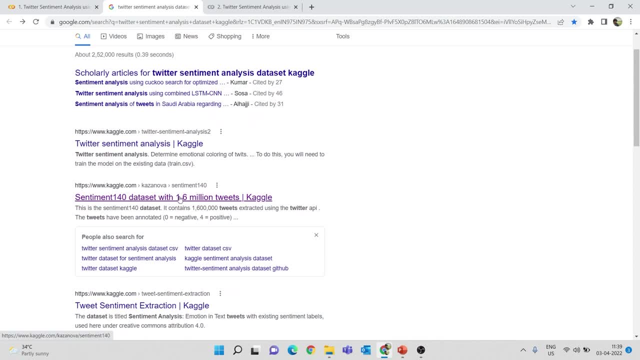 here you will see this uh title called a sentiment: 140 data set with 1.6 million tweets. so this is what we are going to use. so, as you can see, the amount of data set that we have is like it is a very large data set. so it contains like 1.6 million tweets, which is equal to 16 million tweets. 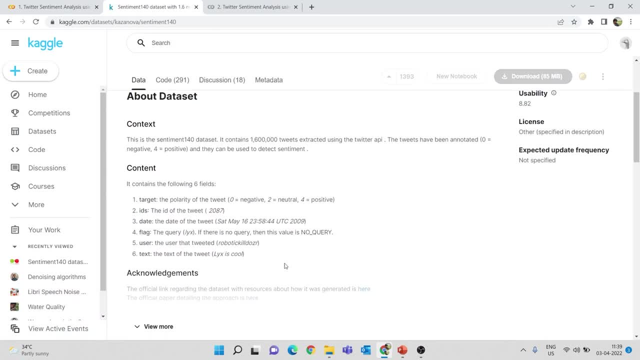 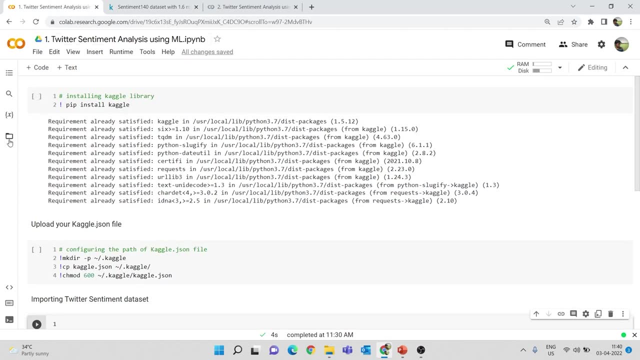 so you can click this one. and this is actually a large data set, so the size of this data set is like 238 mb. so if you want to upload this to this google collab environment, it will take a very long time. so the alternate way is: 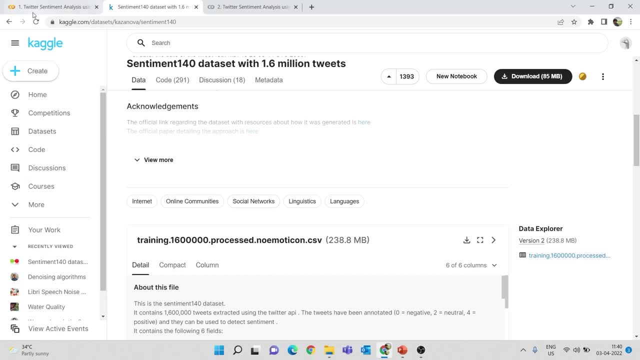 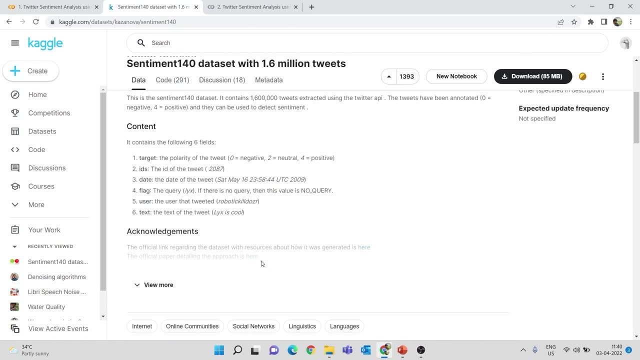 to load this data directly through api from this kaggle environment to the google collab environment, and i'll show you how we can do that. okay, so for this, uh, first thing that you have to do is you have to kind of download the kagglejson file, which is your api token. so in this you can 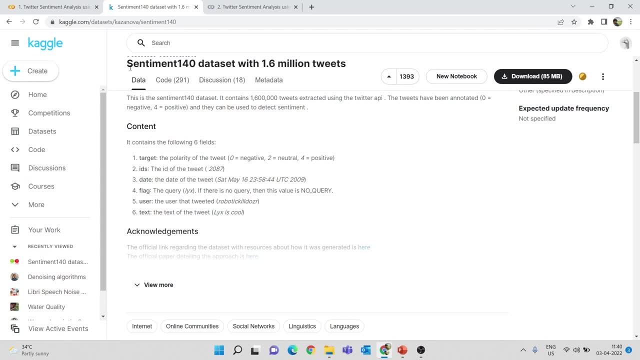 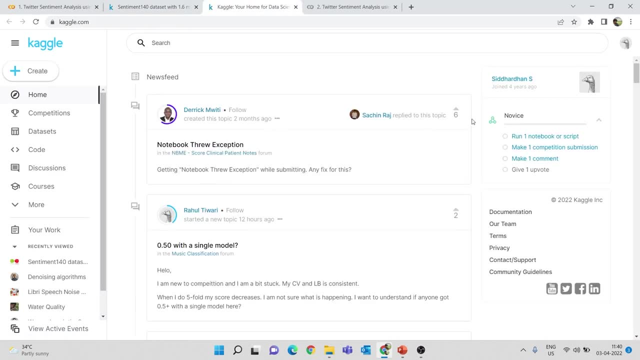 go to the profile icon- okay, so this particular symbol in the top right corner, or you can also go to the kaggle's home page. i hope that you have a kaggle account. if not, you have to sign up for it and also you have to verify your phone number and email address. that is like very important. 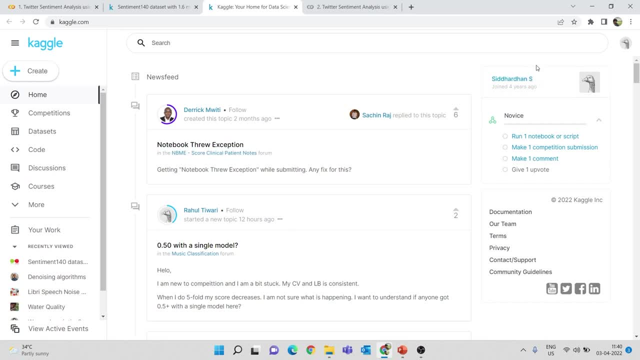 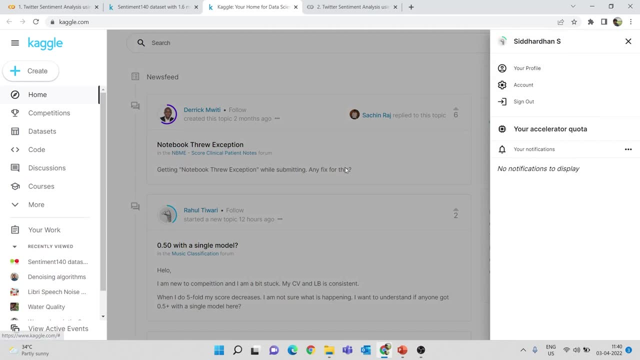 if you don't do that, your uh api won't work. so after, like verifying your phone numbers and email address, you can go to this uh profile icon. if you click this, you will see an option called us account. okay, so in this account just scroll down and here you will find an option called us three. 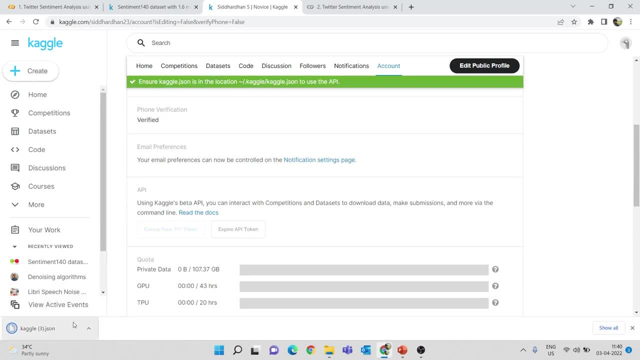 eight new api token. okay, so click this and a file will be downloaded. i have already downloaded this file, so there is a duplicate file that has been downloaded here, so it is basically a kagglejson file which contains your account credentials. okay, so this is the next step that you have to do, then 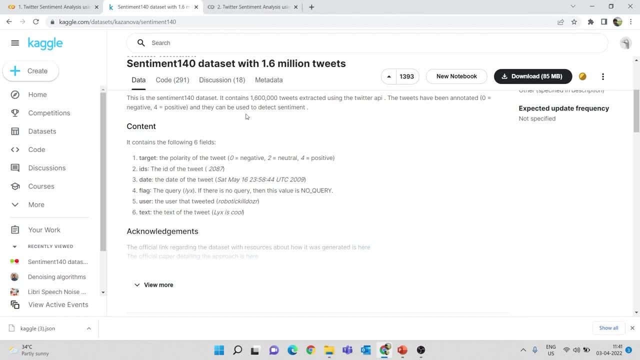 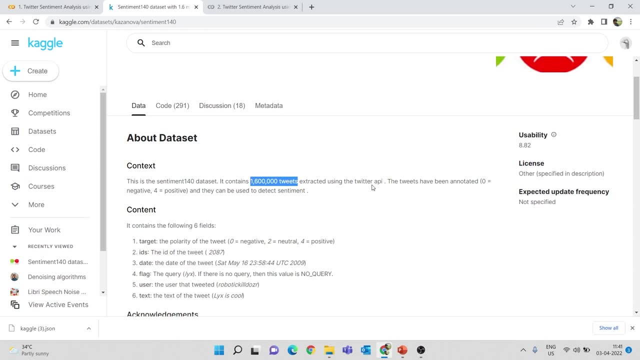 come back to the sentiment 140 data set. okay, so, as you can see, this data set contains like 1.6 million tweets, which is equal to 16 million tweets, and uh. this is extracted through the twitter api and this put this data together and this uh tweets us. two labels: one is zero and the other label is four. 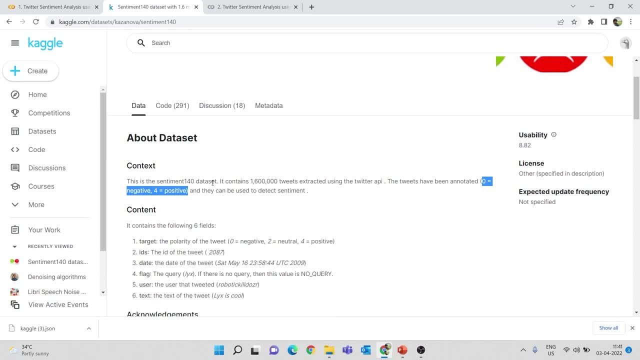 if the label is zero, that means a tweet is a negative tweet, and if the label is four, that means it is a positive tweet. so that is what we are going to classify: whether, uh, the tweet has been made with some positive emotion or it is made with some negative emotion. this is what we are. 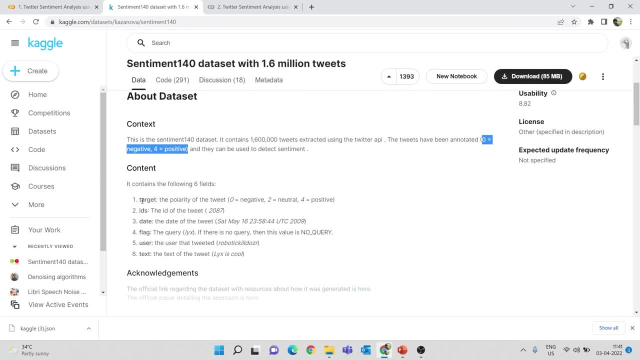 going to classify and these are all the columns that we have. so we have the target, which is the zero or four, and then we have the tweet, id, date, flag, user and finally the text. so the two things are the target column and the text column. so this text column contains the actual content of the 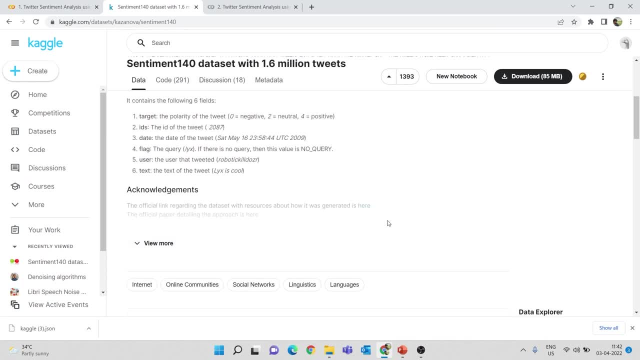 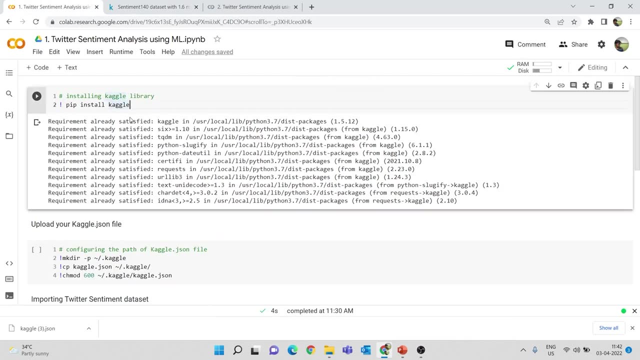 tweet that has been tweeted. so we want these two. so we have to load this data through the api that we have. so i'll show you how you can do this. so first thing is installing this kaggle library. so in google collab this kaggle library will already be pre-installed. so if you want to work in 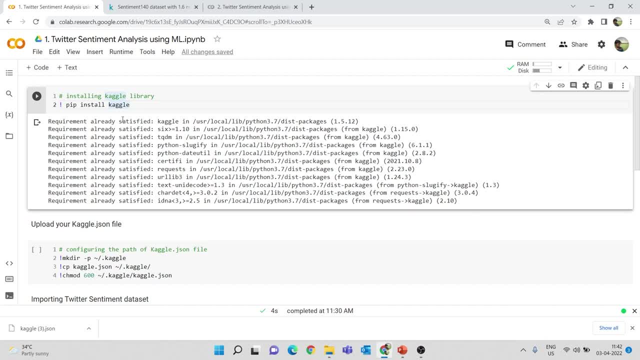 jupyter notebook. you have to install this through this pip install command from anaconda prompt or something like that. okay, so if you are working on google collab, just go to this uh code cell and and write this exclamatory mark: pip install kaggle. okay and uh in order to run this. 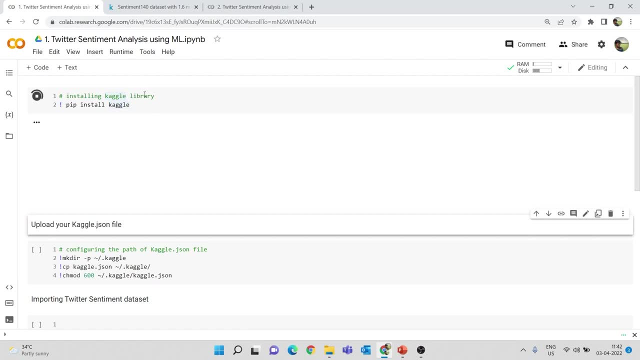 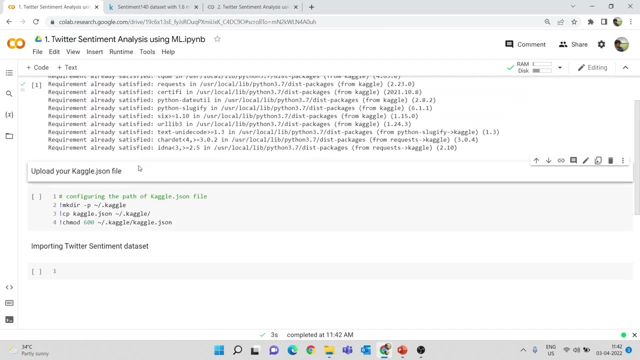 cell. you have to. you know, press shift plus enter, so this will run the current cell and go to the next one. so this won't be available in your new collab environment. it will basically be empty like this. so there will be an empty cell. so here you have to fill this code. the next thing is: 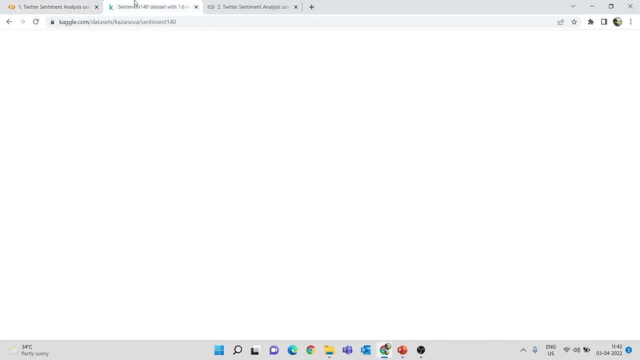 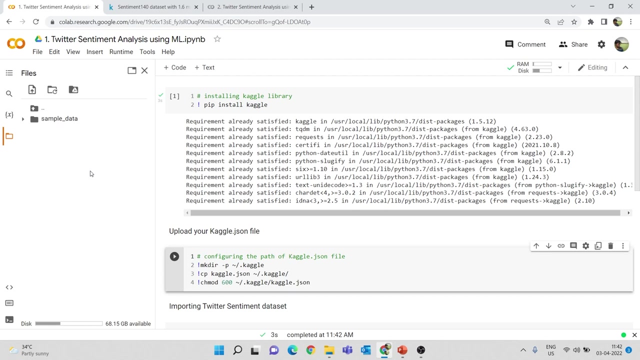 uploading your kagglejson file. so you know that we have downloaded a kagglejson file, right, so we have to upload it here. you can see an option called as files, so i'll click this. so this is directory that we are working on and in this directory we have to upload this kagglejson file. 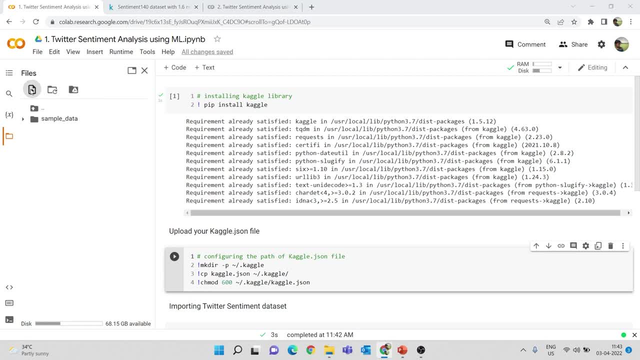 so here you can see this: uh, upload to session storage option. so click this one. and this is the file that i have downloaded, kagglejson. so you have to upload your own kagglejson file here and once this has been downloaded, you have to run this next set. next: 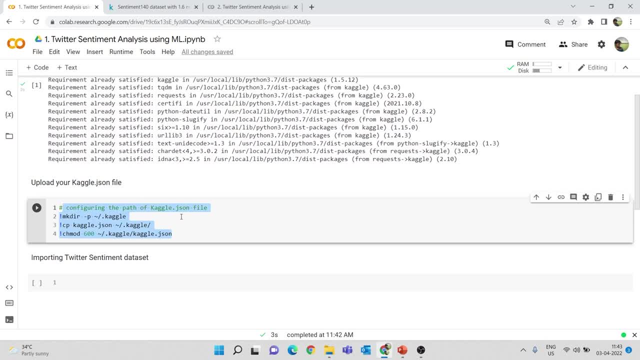 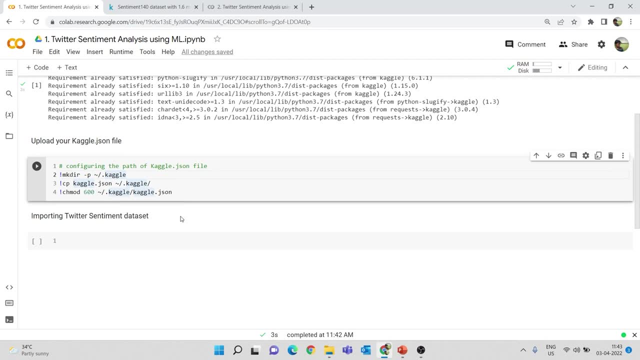 to cell. so this is basically not just to configure the path of the kagglejson file. so this is just to tell where is this json file and how we are going to configure this. so this is the exact code of this collab file. you can just copy this code and you can run this in order to configure this. 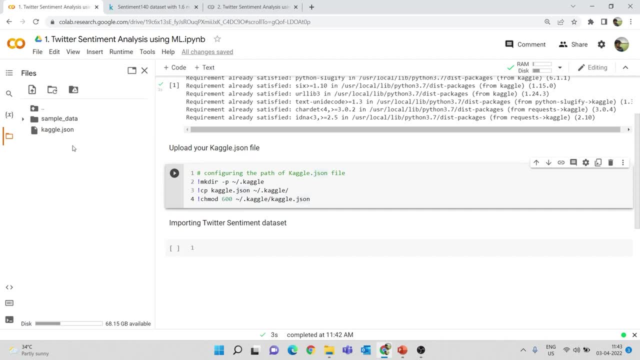 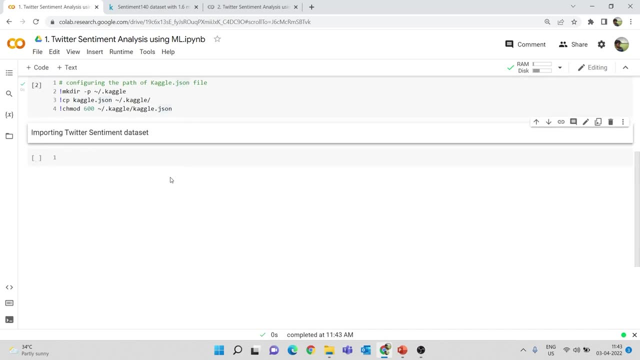 path. so, and the important thing is, you have to do this only after uploading your kagglejson file. so i'll run this cell, and now we are going to import our twitter sentiment data set using api. okay, so the next part of the code is api to fix the data set from kaggle. 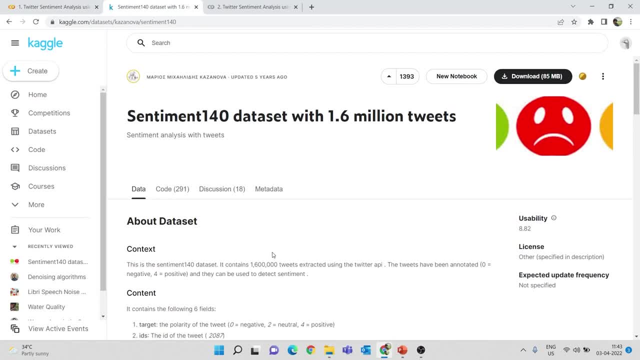 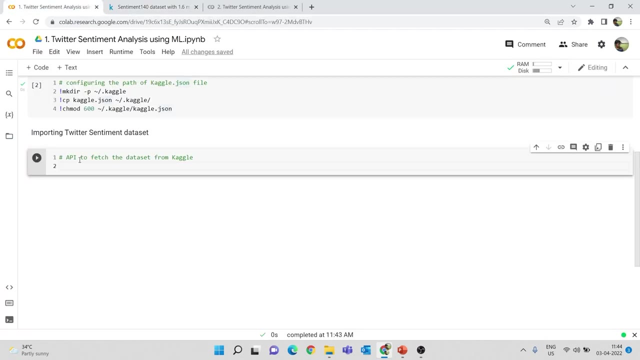 okay, so in order to get this uh api, so you can go to the sentiment 140 data set and here you will see this options symbol. so click this and there will be an option called a copy api command. so click this one so this will copy the api command for this particular data set. come back to your google. 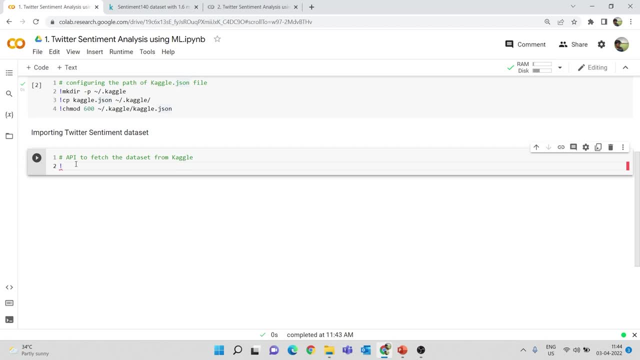 collab environment and you know, just enter an exclamatory mark and paste the api command. so this exclamatory mark is very important. so if you don't include this you will get an error. so we are going to download the sentiment. 140 data set and we are going to download the sentiment. 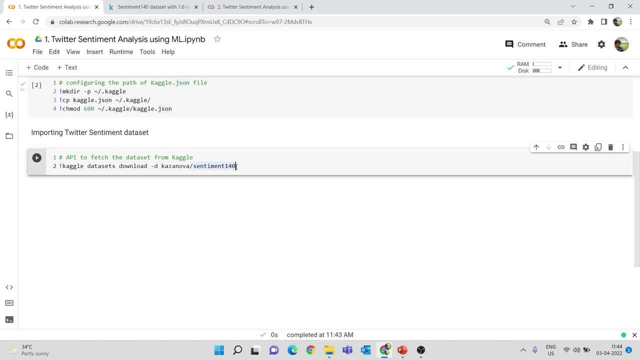 140 data set. so this is the api that we are going to use and just press shift plus enter. okay, so this will download this data set. as you can see, this data set has been uh loaded, you know, very quickly, so it is like an 80 mb compressed file. so if you want to upload this to collab, it will take. 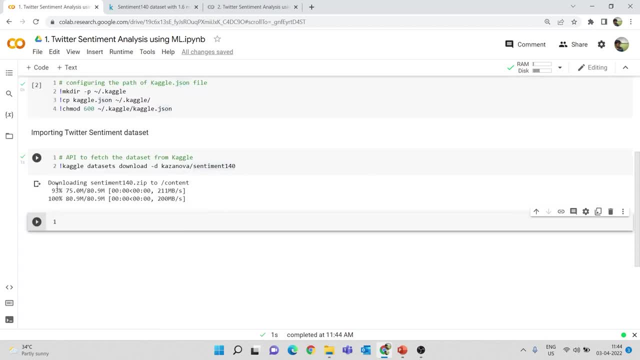 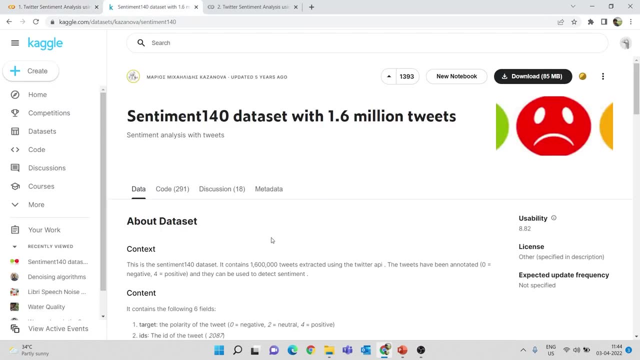 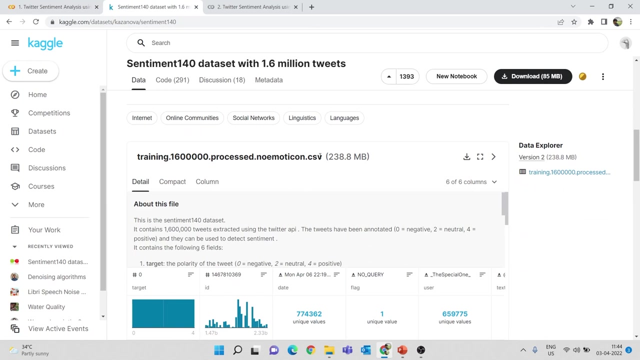 a very long time, so that's why we are using this- uh, you know api method to do this, so this is in a zip file, right? so the next step will be to extract this zip file. the data that we need is in a csv file. as you can see, training: 16 million processed. uh, you know no emotion icon, so this is the data set. 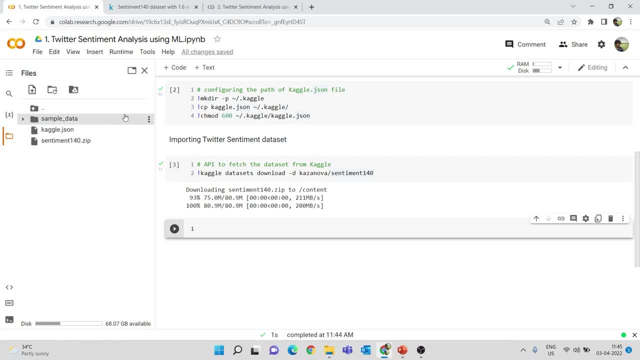 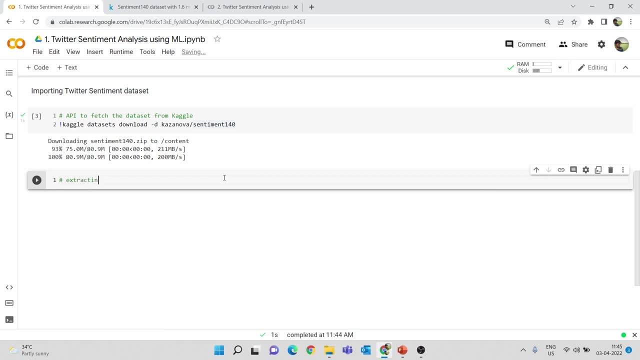 that we need. so we have to extract the zip file that we have. so that will be the next step, so i'll make a comment here- as extracting the compressed file, the compressed data set. okay, so, from zip file. so this zip file is another library that we have in python, so i'm going to use this library. 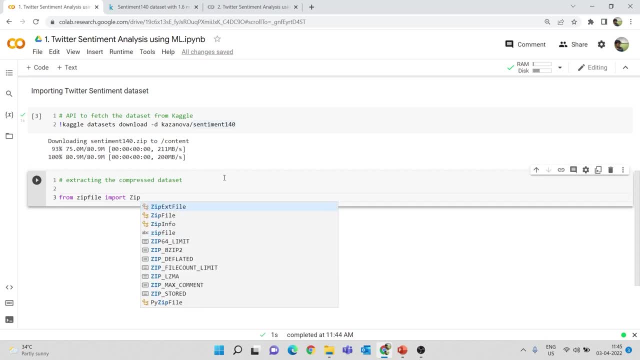 import. so there is a function called as zip file. so here, uh, z and f should be in capital. so this is the library and from that we are importing a specific module and i'm going to specify the path of this data set file, the path of this compressed file. so i'll name this as data set. so this is just. 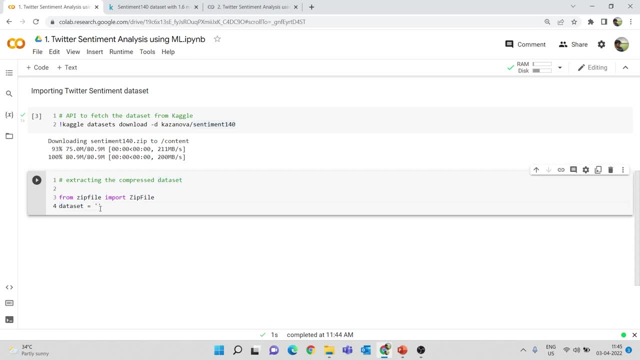 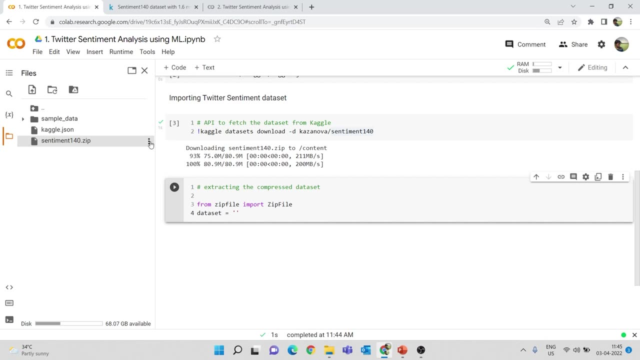 a variable so you can name this anything. so you have to mention quotes here and within this quote you have to paste the path of this file. so in this: so this is the compressed file and you can see this option symbol. so click this one and copy the path. 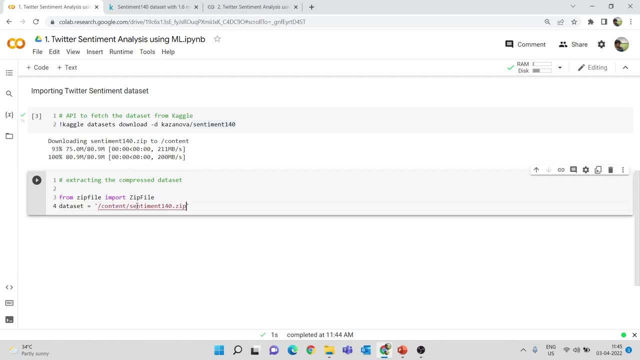 once i have copied this path, i'm going to paste it here. okay, so this is the path of my file, and now i'm going to open this file and extract it, so i'll say with zip file, which is the function that we have imported. so with zip file, here you have to. 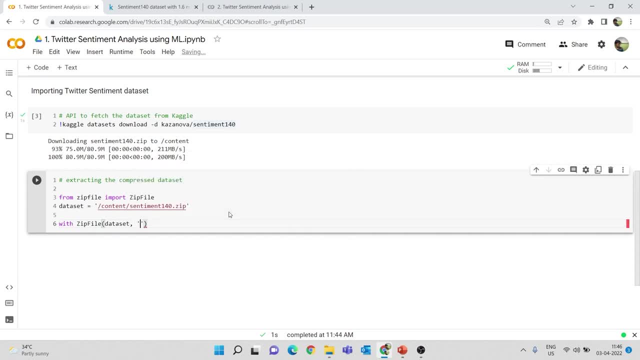 mention the path of the data set, which is data set, comma r. so r stands for read. so we are going to read this compressed file as zip. so, again, this is a variable name. you can use anything. so i'm reading this and i'm, you know, reading it, uh, with the name zip, and i'm going to extract this. so i'm going to. 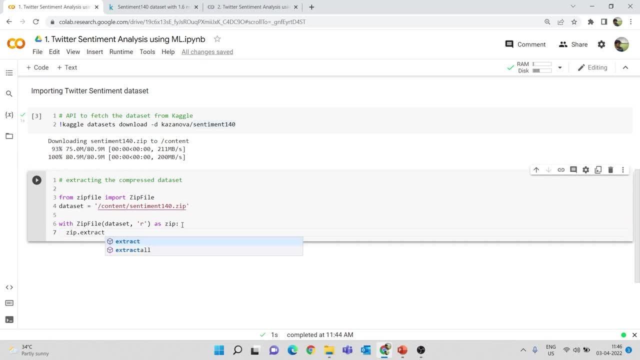 say zipextract, all in parenthesis- and finally, once this is extracted, i'm going to say print, the data set is extracted. okay, so this is the code in order to do this. uh, you know extraction process in python. so we are importing this zip file, uh, library and 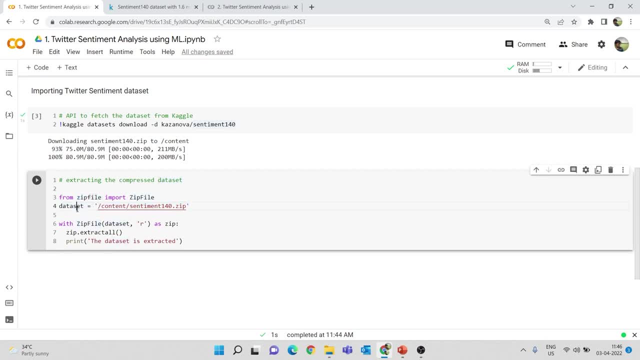 we are specifying the path, so the path of the compressed file that we want to extract, and i'm opening this file. so I am using the zip file function and I am mentioning the path of this file, which is data set, and I am reading this file as zip and then I am mentioning zipextract also. 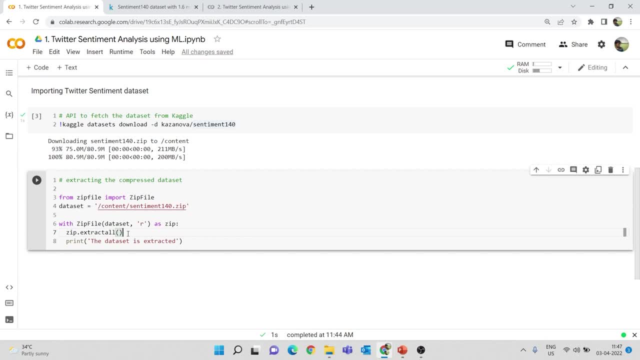 this will extract all the components of this compressed file and it will store it in my parent directory. so I will run this one. so once this extraction has been completed, this line will be printed, which is: the data set is extracted. okay, so now the data set is successfully extracted. 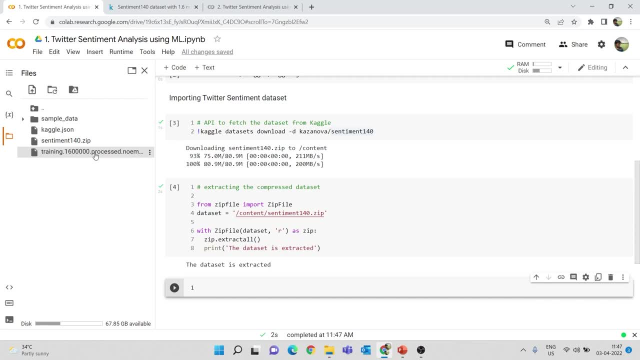 now you can go to this files. as you can see, the data set is extracted. so this is the file, the, which is this training dot 16 million thing, okay, okay, so this is in the form of csv file. you can rename this using this. so you can go to this option. you can rename this file or you can just. 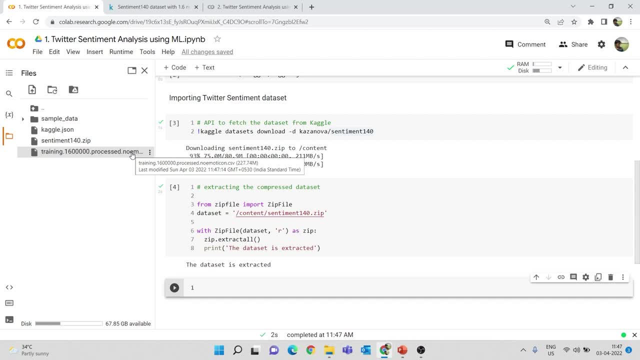 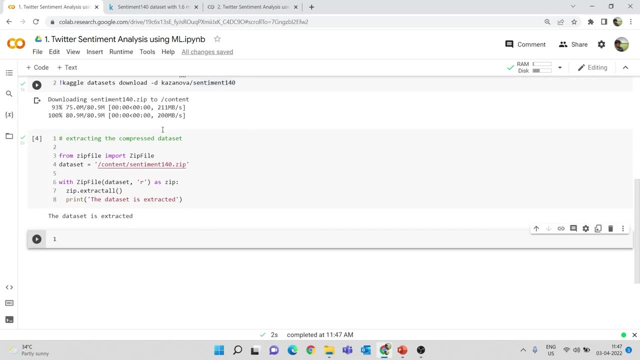 keep it asset, so let me not, you know, change the name of this file and the next part will be to importing. you know the dependencies, so we need, like, several libraries and functions in order to do this sentiment analysis task. so we are going to import that required dependencies and the 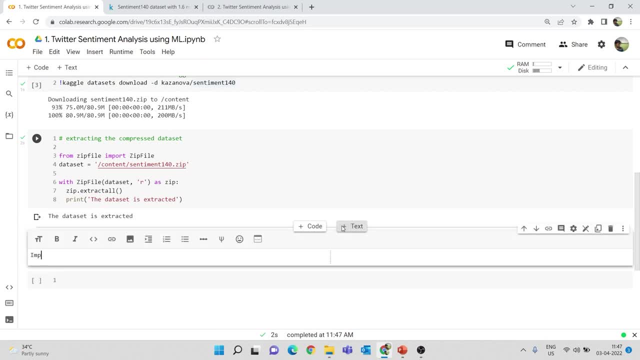 functions for this process. so the next part will be importing the dependencies. okay, so, importing the dependencies, first I am going to import my numpy library, which is a very basic python library, and then I am going to import this pandas library. okay, pandas is used to create data frame. okay, so, as you know, the data set is in. 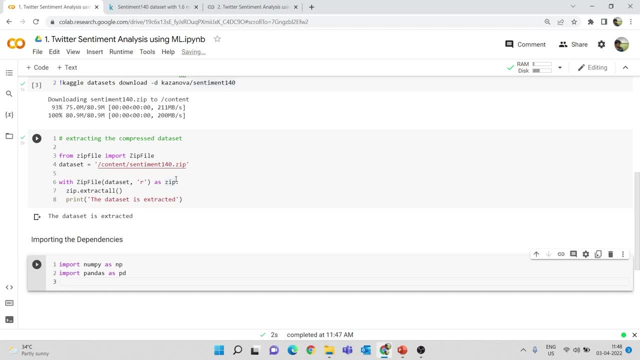 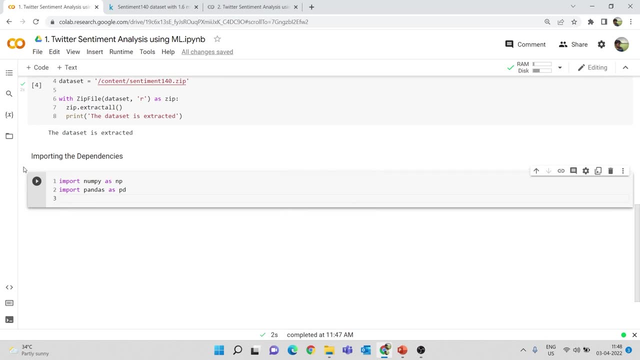 a csv file. so it is not easier to process the data and analyze the data when it is in a csv file. so we will load it to the css file and then we are going to import the css file. so we are going to pandas data frame. so data frames are nothing but structured tables, so we will feed this data to 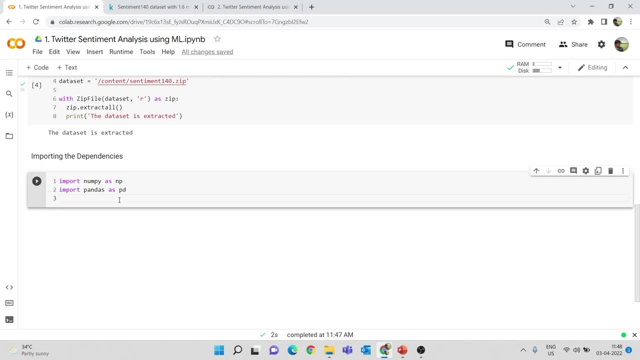 this structured table called as data frame, and we will do all the processing and analysis. so that's why we need this pandas. and then I'm going to import re, so re stands for regular expression. so this is used for us in order to do some pattern matching, search through the data, and so on. 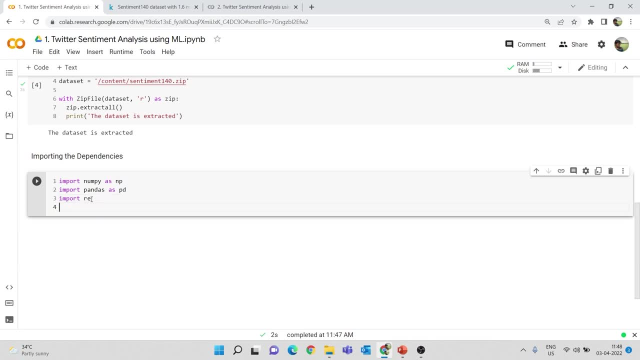 so I'm importing this re so again. so these libraries are already pre-installed in pre-installed in google collapse. if you are working in some ids like spider or quite charm, you have to install it using pip install command. and the next thing that I'm going to import is from nltkcorpus. 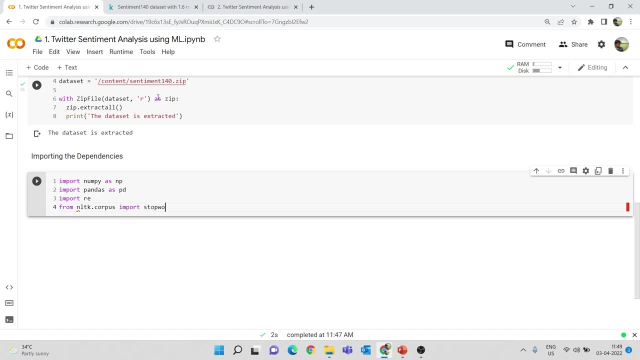 import- stop words. okay, yeah, so nltk stands for natural language toolkit, so natural language processing is something that we do in textual data. okay, so I'm importing this natural language toolkit library, which is nltkcorpus is the module that I'm importing from that? I want this. stop words. 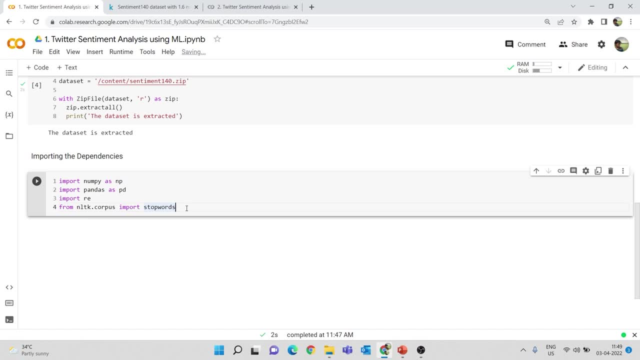 module. so I'll explain you what this stop words means in the upcoming part of the code. so this is the next thing that we need. later I'm going to import from nltk dot stem, dot porter. okay, so, dot porter, I'm going to import porter stemmer. 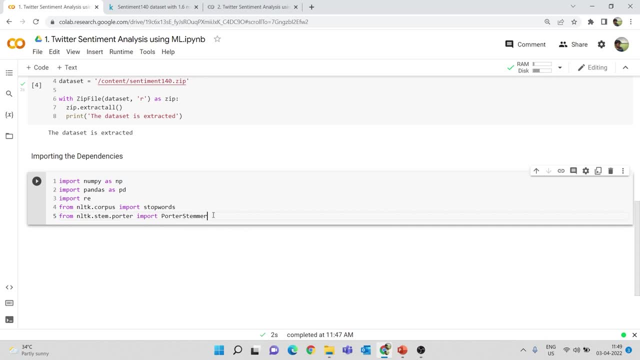 okay, so porter stemmer, so the use of this, uh, a porter stemmer, is. then there is a processing called a stemming that we do, which is, uh, you know, used to, uh, you know, reduce a word to its, to its, you know, kind of root word. so I'll explain you this, uh, in a later part of the code. 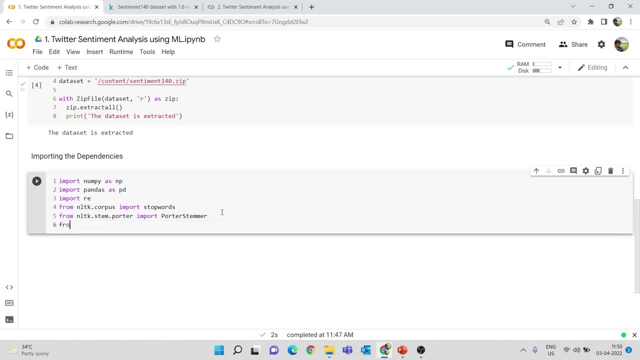 where we will use this porter stemmer. and the next thing that we need is from sklearn. again, sklearn is a very famous and widely used machine learning library, so I'm importing this from sklearnfeature extraction import tf idf. okay, so the purpose of this tf idf vectorizer is that, as I told you earlier, we cannot feed. 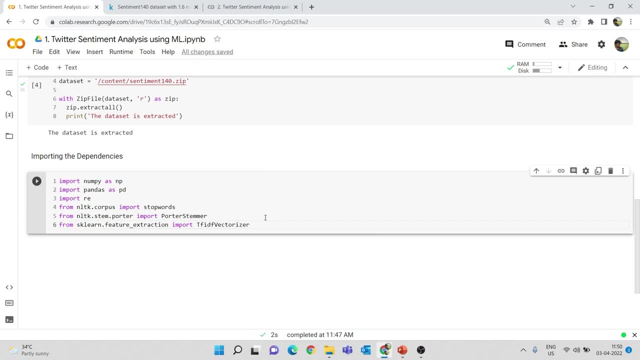 the textual data to our machine learning model. and, uh, you know we have to convert this textual data into numerical data and that is the purpose of, you know, importing this tf idf vectorizer. so just a second. okay, the next thing that I'm going to import is from sklearn dot model selection. 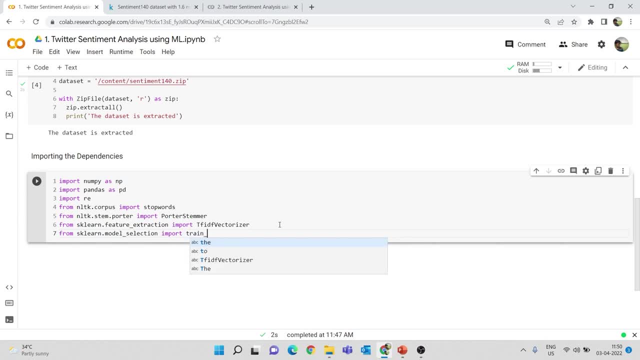 import train test split. so this train test split is a function is used to split our original data into training data and test data, where the training data will be used for training our ml model and test data for evaluating our model. and then I'm going to import my machine learning. 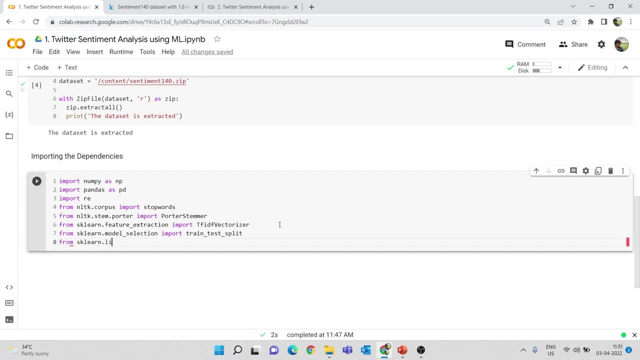 model from sklearn dot linear model. let's import logistic regression. so in this case, I'm going to train this tweet data, or pitta data, with logistic regression. So I am importing this logistic regression with you know, this logistic regression from sklearnlinear model. and finally, I am going to import my accuracy score from sklearnmetrics. 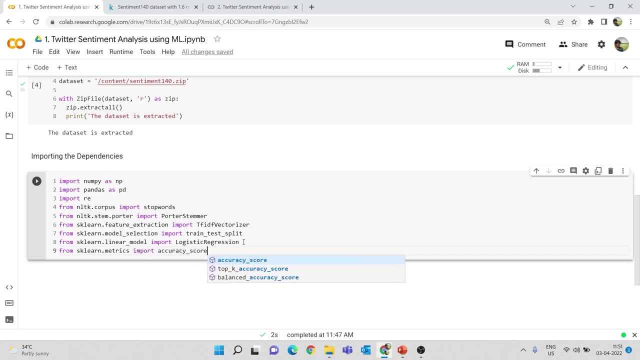 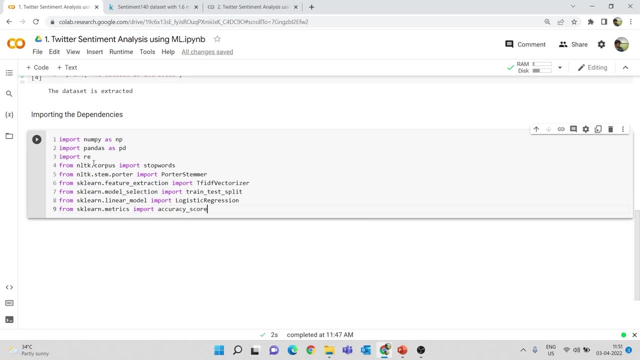 import accuracy score. So these are all the. you know the nine things that I need. So I am importing the numpy library, pandas and regular expression library and later I am importing my stopwatch for test ml tfid vectorizer and then I am importing this train. 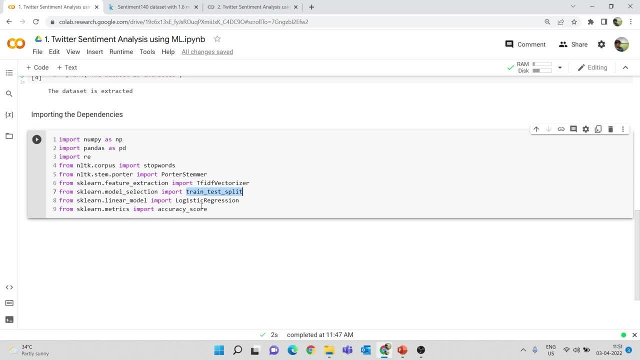 test split, which is used for splitting the data into training data and test data logistic regression for, you know, training my training with this data. So this is the ml model that we are going to use and, finally, we are importing this accuracy score, which will calculate the accuracy and the performance of our machine learning model. 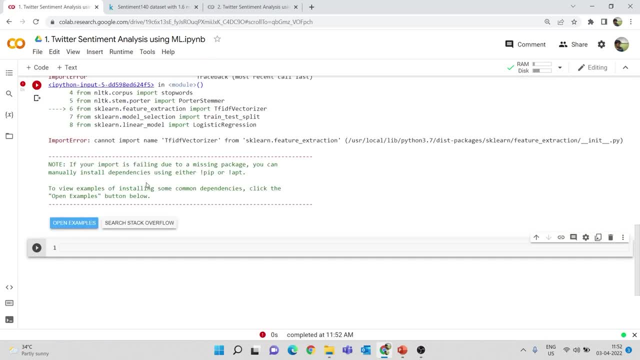 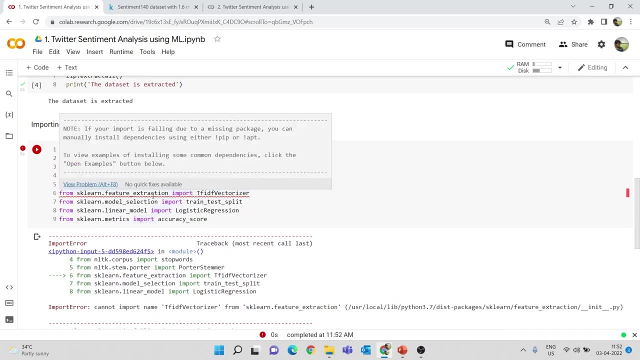 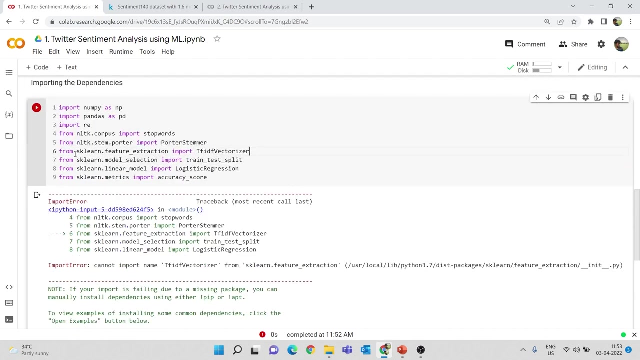 So I will run this one. so this will import all the dependencies that we need. So cannot import name from: ok, so there is some error. let me just check this one. So sklearnidf, tfidf vectorizer- ok, so I should say from sklearnfeatureextractiontxt. 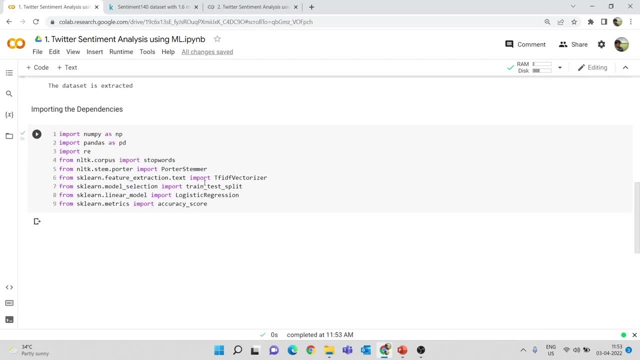 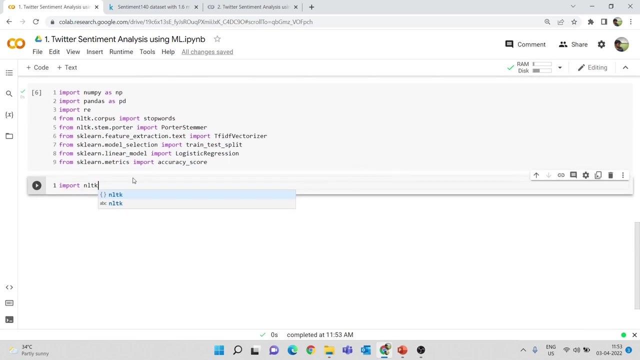 I missed this text one, so I will run this one now. I will not get any errors, as you can see. So these are all the dependencies that we need. so the next thing is downloading this stopwatch. So I am going to say import nltk and from this nltk we have already imported this stopwatch. 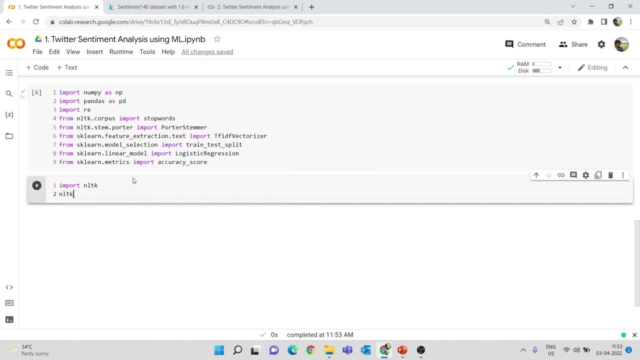 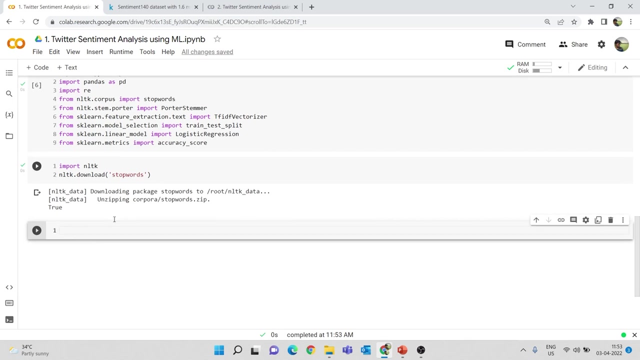 right. So nltk and nltkdownload, and in this parenthesis, in this quotes, I have to say stopwatch. So let us try to understand what does this stopwatch means? so this will you know, download all this stopwatch that we have. So here I am going to print. 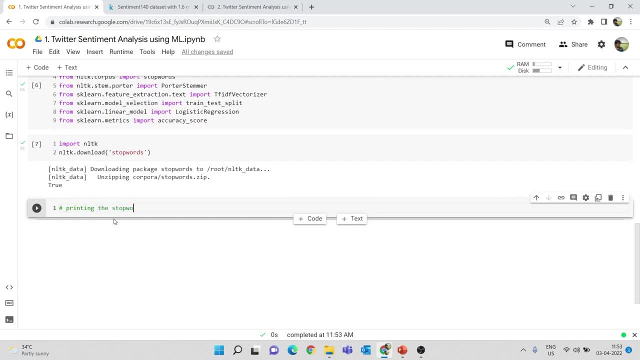 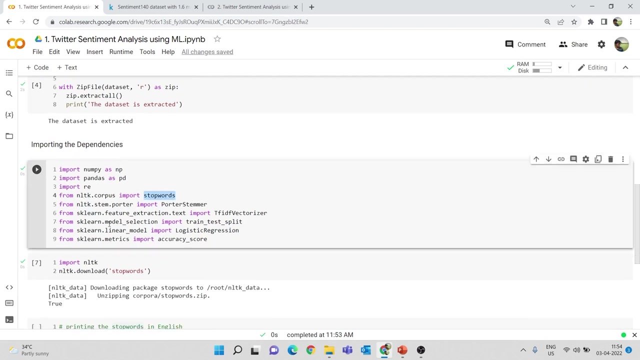 So printing is stopwatch In English. ok, let us say print stopwatchwordsenglish. ok, so this stopwatch is nothing but which we have imported here from this nltkcorpus. So then let us run this one and try to understand what this stopwatch means. so it basically. contains the words like I, me myself, we, our, ours, etc. So let us run this one and try to understand what this stopwatch means. so it basically contains the words like I, me myself, we, our, ours, etc. 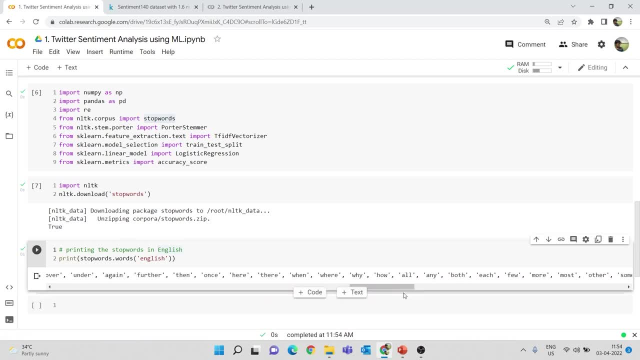 So let us run this one and try to understand what this stopwatch means. so it basically contains the words like I, me, myself, we, our, ours, etc. And you can also, like just you know, scroll through it in order to understand what are. 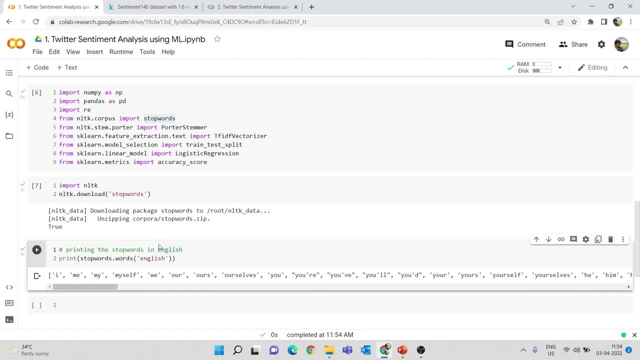 all these words. So stopwatch is something that does not add any meaning to your textual data. so it has some meaning, but it does not have any influential meaning. So if you remove this I from that, it is not required for us. so, like these are words that 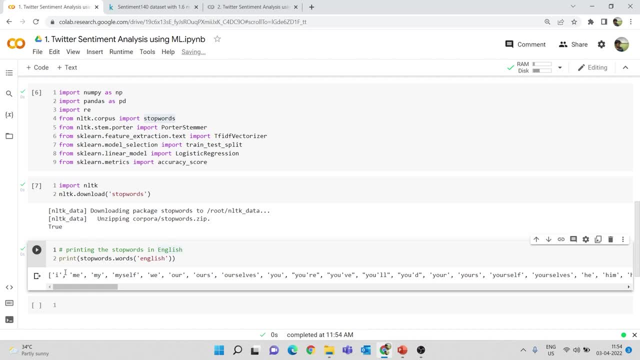 is not required for processing, so the machine learning module does not required for these words, so we have to remove these words from the text that we have. So this does not have that much importance. okay, so that is what I can understand: the stop words. so stop words in any 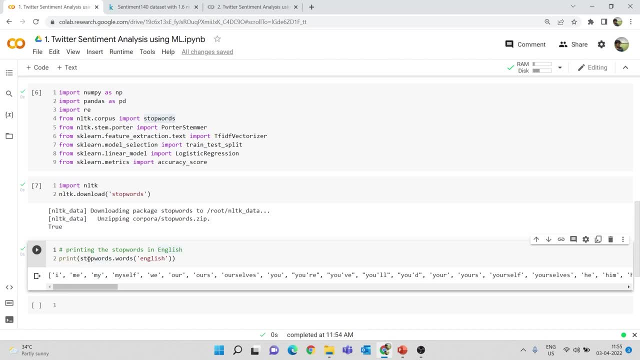 languages of those words. that doesn't add that much importance to that context of this. okay, so of course, I, me and my myself, all these- have some meaning, but it doesn't have that much contextual importance, so we don't need to, you know, include these words from our tweet. so what this actually does is so we will. 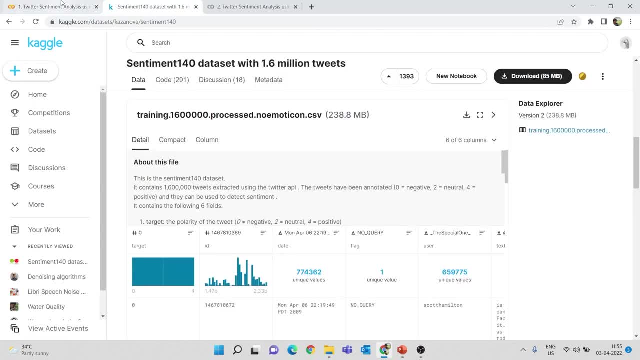 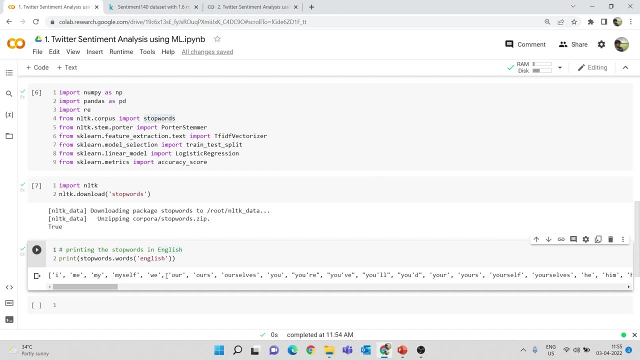 take this stop words and we will remove those from this. 1.6 million tweets, so we have several. you know tweets, data right. so in each tweet we will remove the words, like I mean my myself- 6a, so we will keep only the important words. so 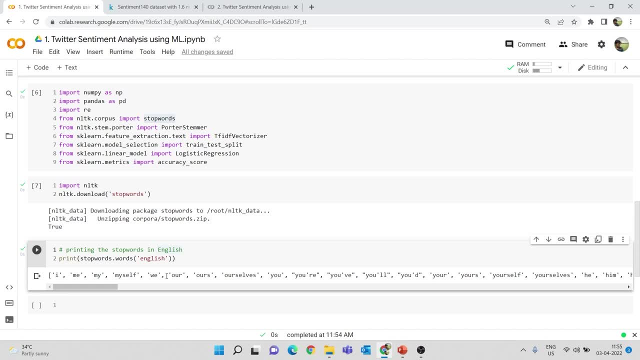 that's why we need this stop words. the reason we are doing here is, as we know, that the data set is very large and we have to do everything possible in order to, you know, reduce the size of the data that we are, in order to reduce the 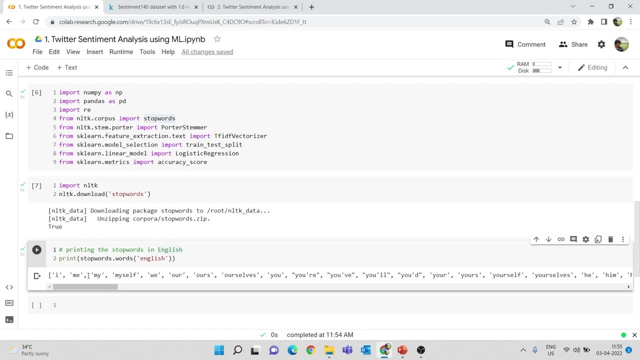 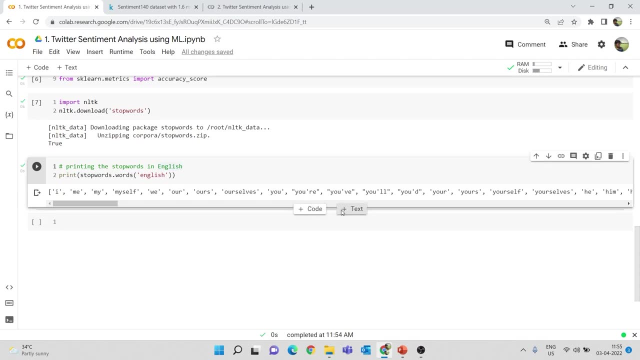 complexity of the data that we are, and one such process is removing the stop words, as it doesn't have that much meaning to it. so that's why we are doing this, and the next thing will be how we are going to process our data set. so this will be: 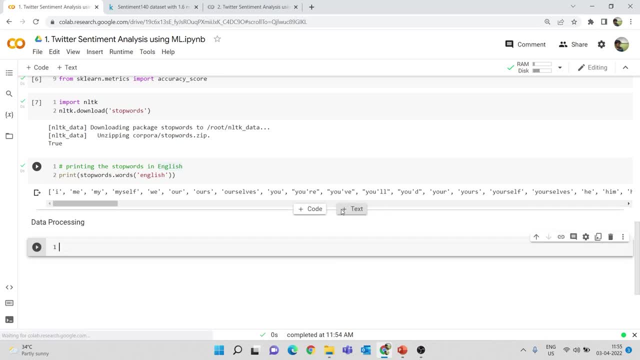 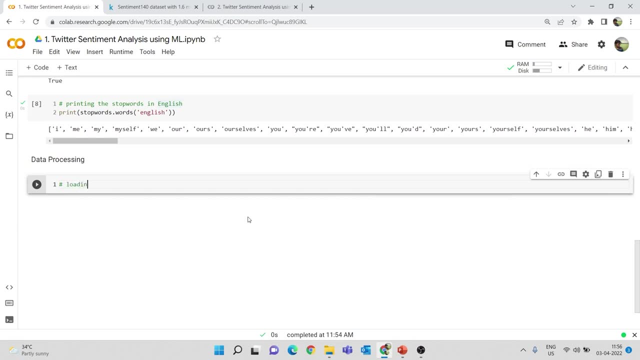 data data processing. Okay so here I'm going to load the data from the CSV file to a pandas data frame. Okay so, loading the data from CSV file to pandas data frame and I'll create the data frame named as Twitter data. Okay so, Twitter data is equal to. I'm going to use 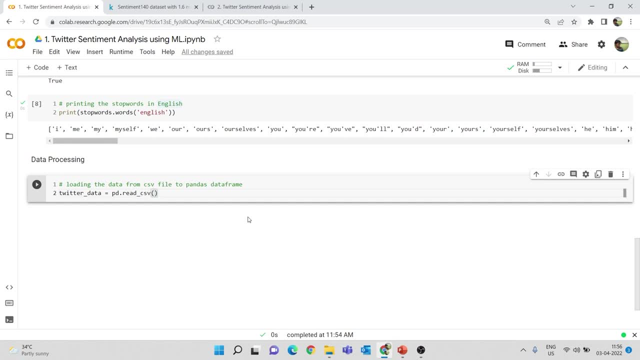 the function PD dot read CSV. So this read CSV function will read the CSV file and load the content to a pandas data frame. So here I have to mention the path of this file. So I'll go to this files and I'll copy. So you have to give this options and you can copy. 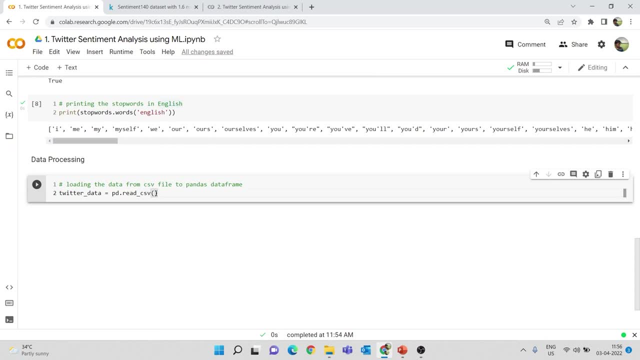 this path of this file and put that path of the file within quotes. So in this parenthesis you have to create opening, close quotes and closing quotes. you can either use single quotes or double quotes And, just you know, put another comma to it. and we have to mention: 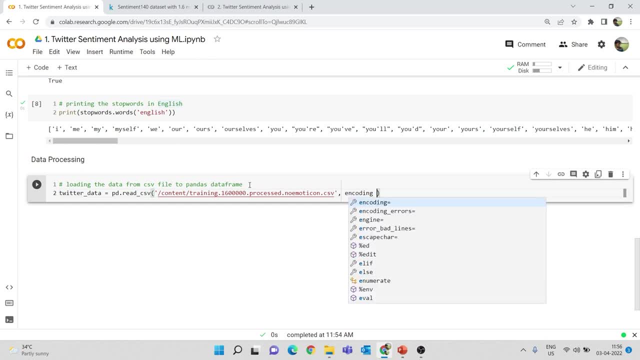 what is this? The encoding here I'm going to say encoding is equal to ISO. So this is like a standard, normal standard that we have, So w8591.. So this is one kind of encoding that we have in this PD dot read CSV. So yes, for w8591.. So I'll run this one. So the parameters that. 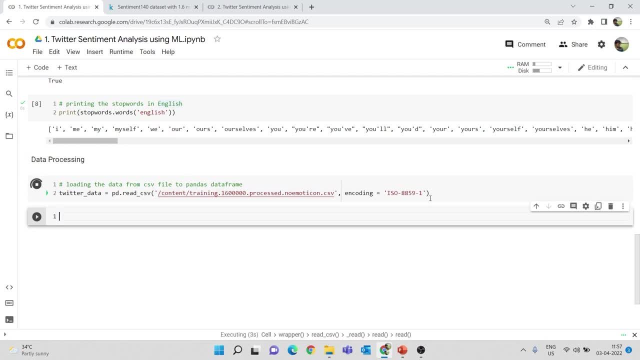 we are passing are the path of the CSV file and what is the encoding method that we have to use. So we have some things And yeah, so now this data from CSV file has been loaded to this data frame and we have named this data frame as Twitter underscore data, And you 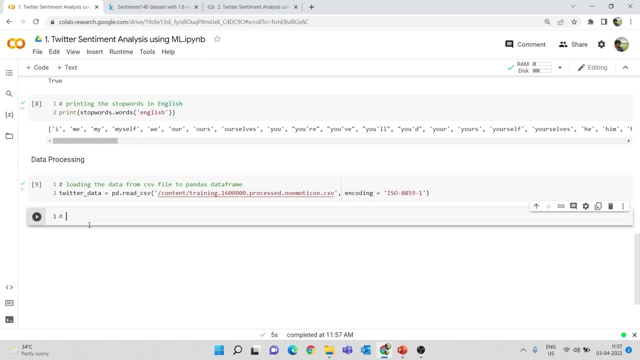 can check the total number of data data points that are there present in this data set. I'm going to say Twitter data. So this is for checking the number of rows and columns. Okay, so rows is nothing but the total number of tweets that you have. Okay, so specific rows. 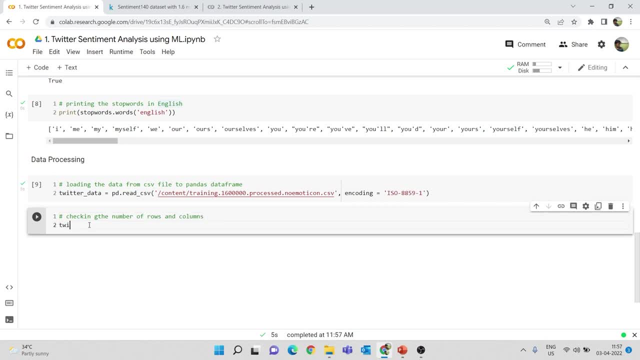 columns. So they are the number of rows and columns. Okay, so rows is nothing but the total number of tweets that you have, So I'll try to do this. So if you see that this is So, I'm going to say Victor, data dot shape. 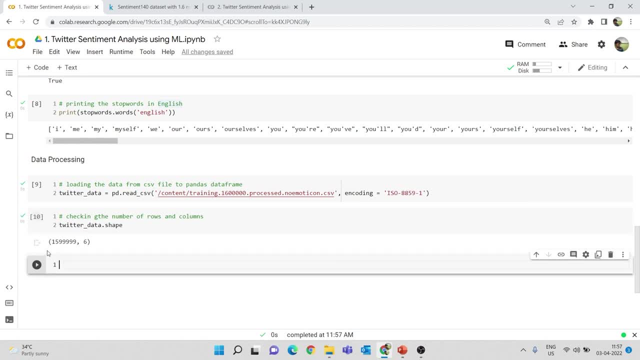 So this will tell me how many rows and columns are there in my data set. So there are like 15, like 999, so this basically means like 16 lakh, because in Python indexing starts from zero. So if there are like 10 numbers are there, so the counting will start from 0, 1, 2, 3 and 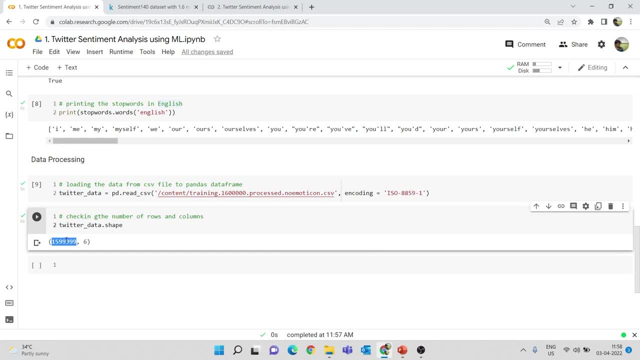 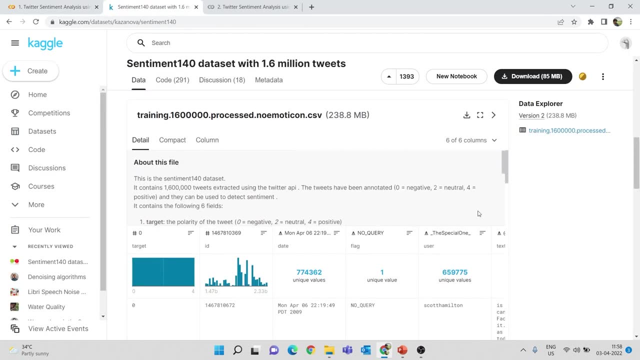 so on. So this basically means there are like 16 lakh tweets, because the first number starts with zero instead of one. So that's why we have this count and there are totally this six columns. So this is six column is nothing but my. you know targets as you can see. so target IDs. 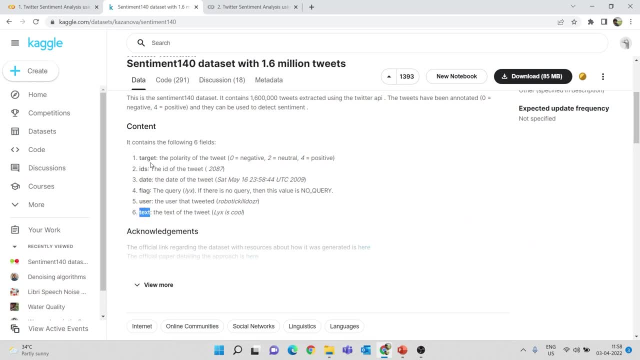 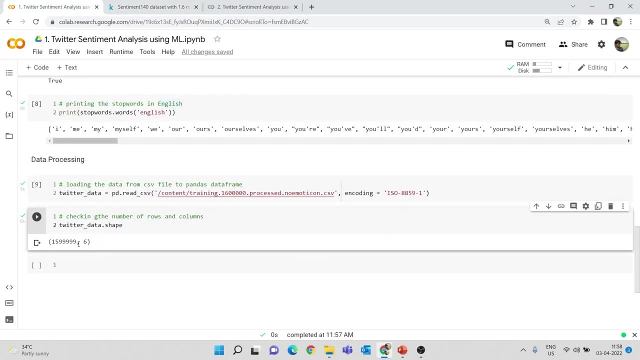 date, plug, user and text. So, apart from like within this, we just need this text and target alone, but let's go into that later. but these are like the six columns that we have, which is mentioned here. So there are like 15 or sorry, 16 lakh tweets and like 16 columns to it, and also you can. 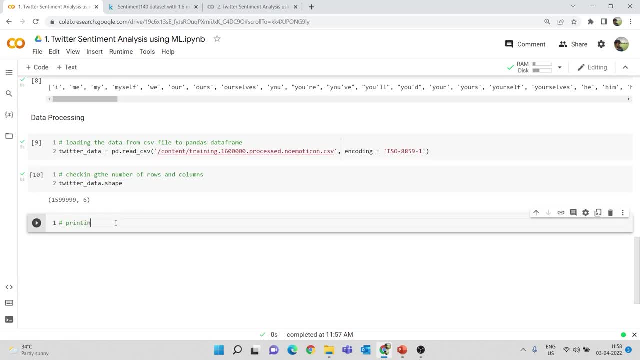 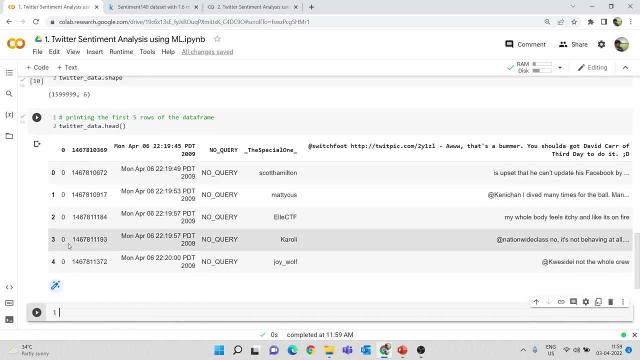 print the first five rows of this data frame. So I am printing the first five rows of this data frame And I am going to say Twitter data dot yet. so this yet function will print me the first five rows. So, as you can see, these are the first five rows. 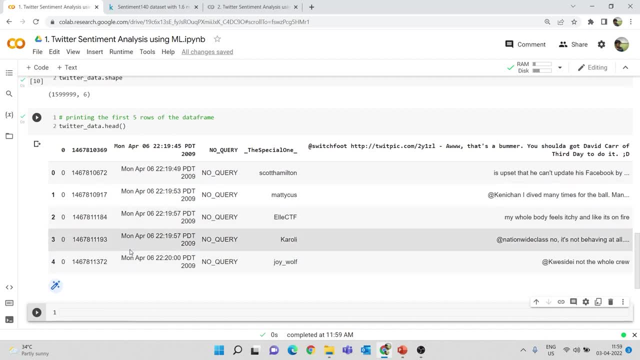 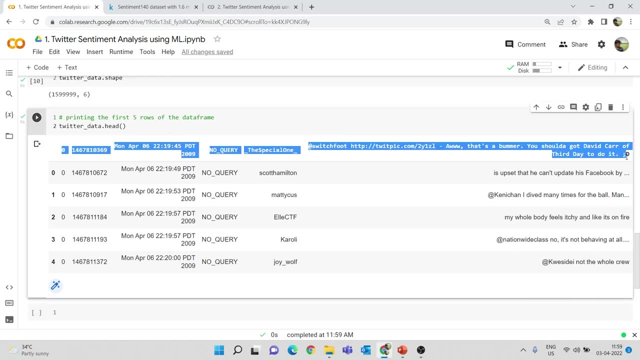 So we have this target ID or date query and so on, but there is like one important thing that we have to note here. So this is actually a data point, but this has been considered as a column name, So this is in bold letters, right? 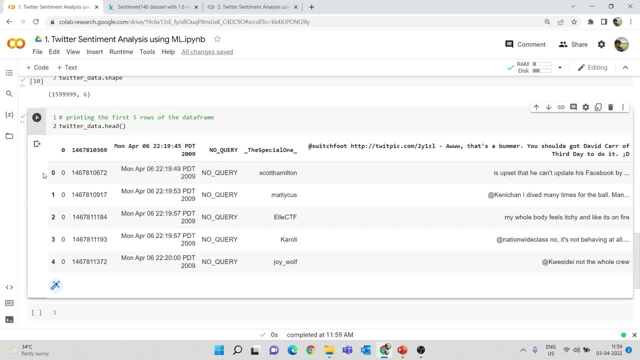 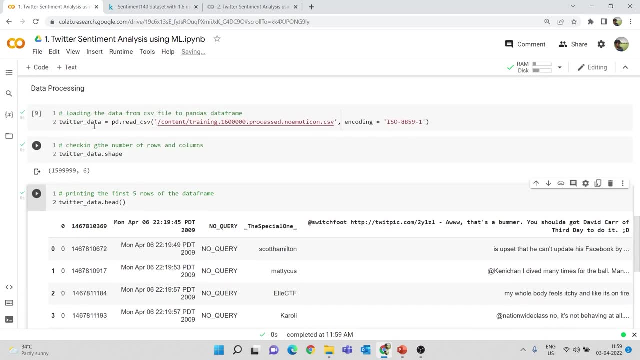 So what this means is, Like, this is the column name and this is my first data point, So this is my first data point which starts with zero. So this column names are not being read by this PD dot read CSV. okay, So when we use this function, so this ID target date flag. 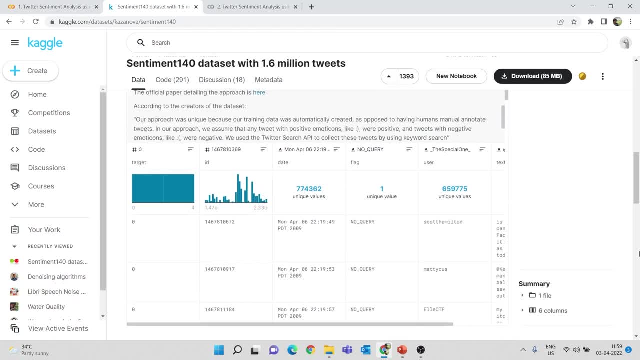 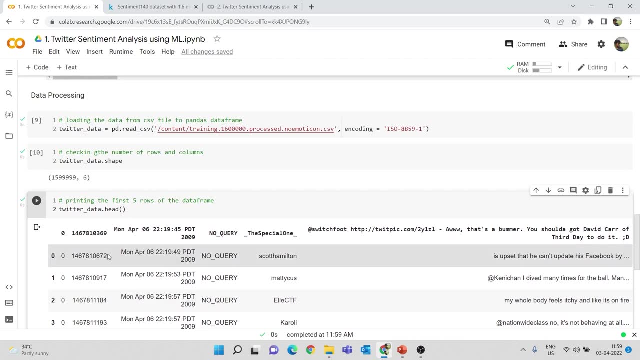 So these are all not read by this PD dot read CSV and the first value is being read as the column name. okay, So if you see here the value is like zero, six, seven, two, right, So this is the value that we have. So we have to tell the PD dot read CSV that you are not reading the column name. 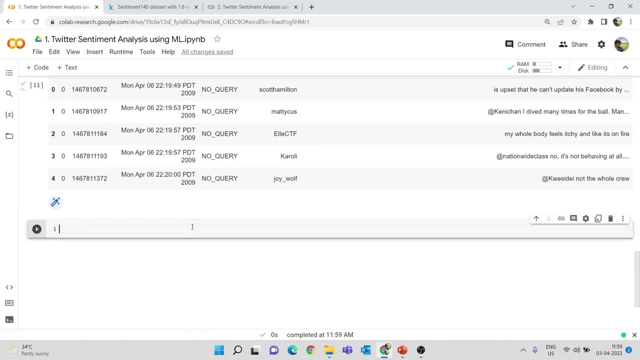 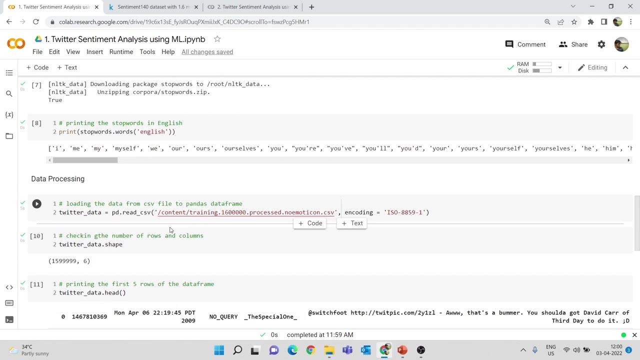 So you have to do that change. Let's try to do that. So I'm going to name the columns, naming the columns and reading the data set again. reading data set again. So I'm going to, you know, do the same task of Twitter data PD dot read CSV. but I'm just 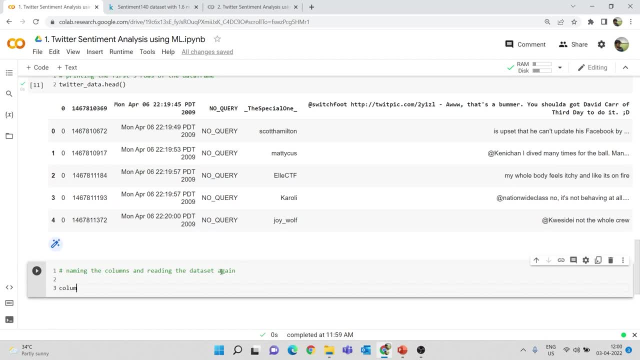 going to add one more thing to it. I'm going to say column names, So column names is equal to. so I'm creating a list. So the first value in this list is target, and then the next item is ID, and then I'm adding this date, and then flag user and finally- let me put this as text- 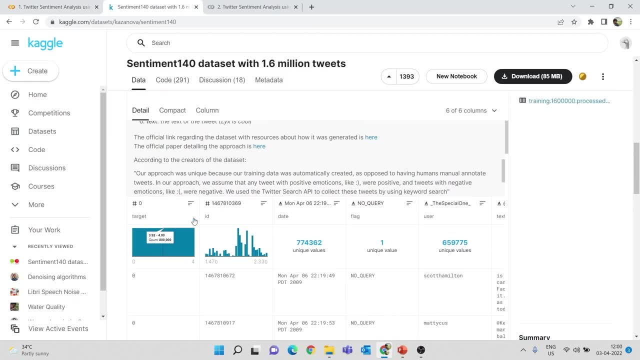 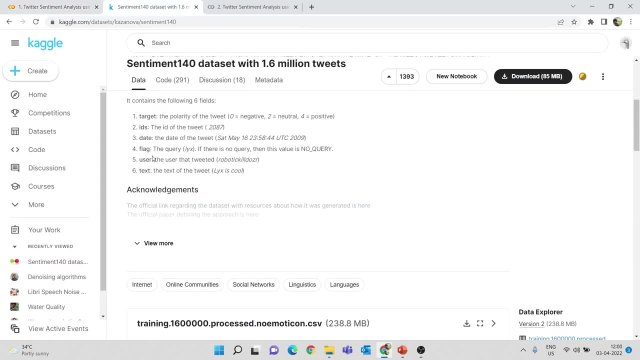 Okay, So where I'm getting all this? This is from this one, So these are the column names that we have. So first is target, So that's why I made like target as the first one, and then we have this: ID is date flag. 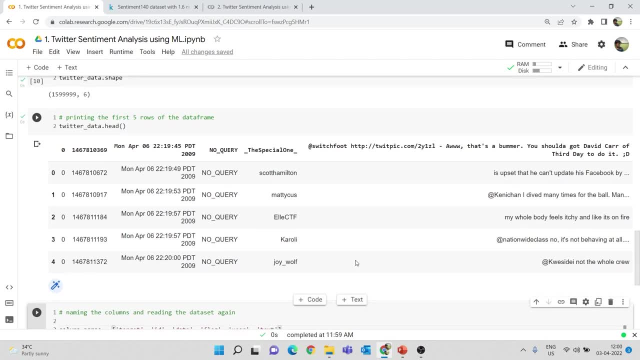 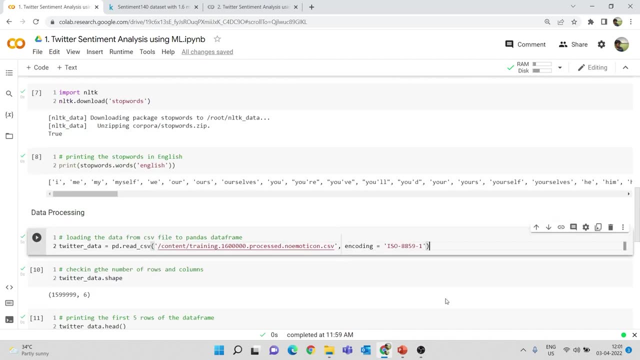 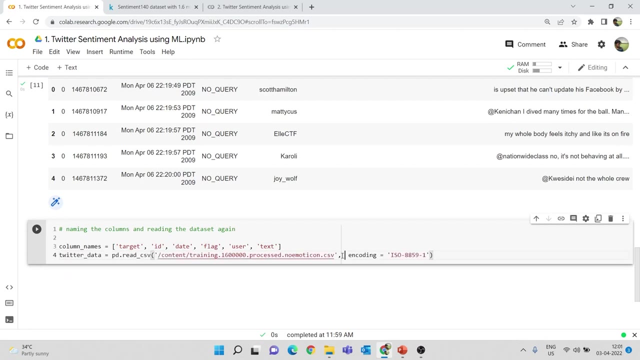 user and text. So I have named all these columns and now I have to read this data set file again. So I'll copy this part of code, this line alone. we copy this and put it here. okay, Now, before this encoding, I'm going to use another parameter, which is names. so names. 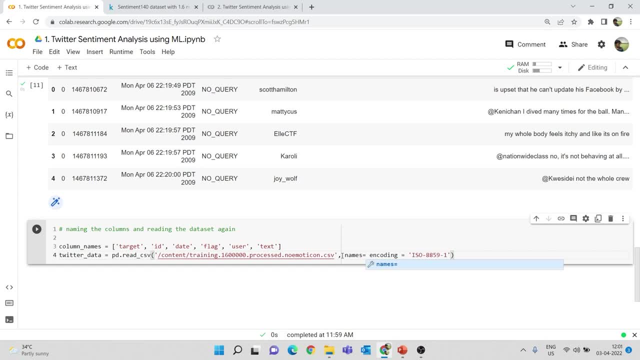 is equal to Column names. So this column name. so you have to, you know, put another comma here. So this column names is nothing but the column names that we have created here. So I'm using this PD dot read CSV. I'm reading the CSV file and this is the name of the columns. 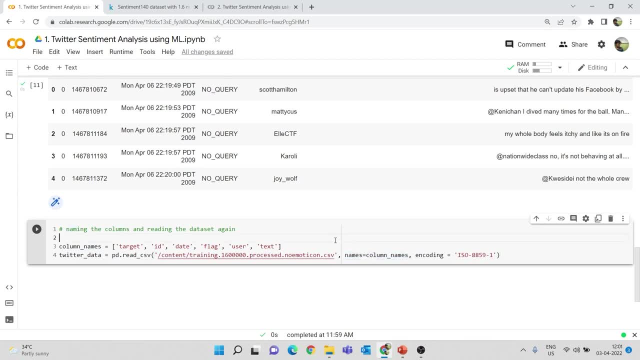 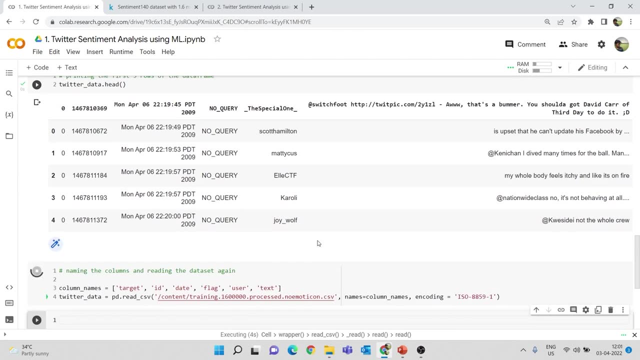 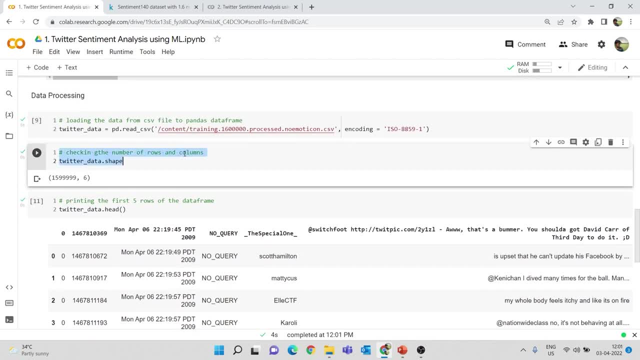 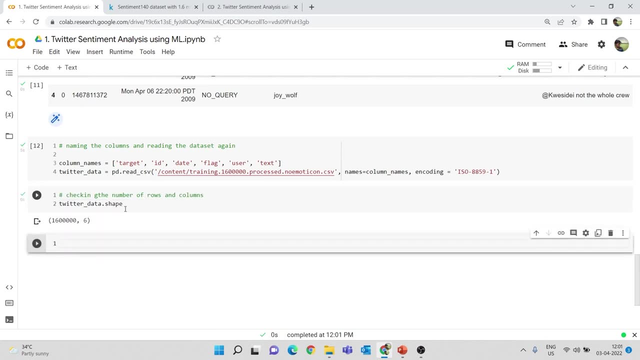 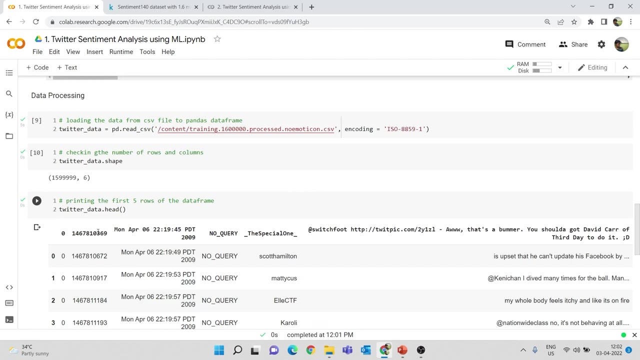 I have my data, Okay, So now I'll copy this one. So now it will, you know. show this as 16 lakh tweets are there, okay, So 16 lakh tweets are there, because previously what happened is like the first tweet has been read as a column name. 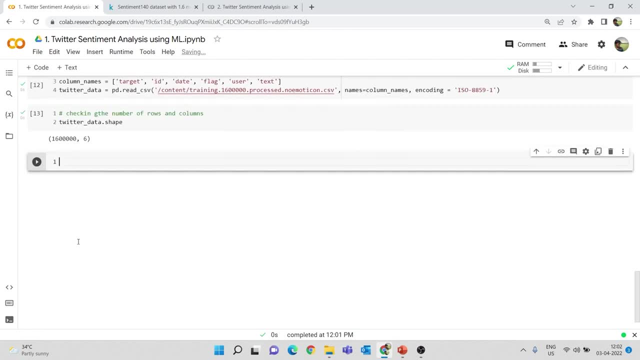 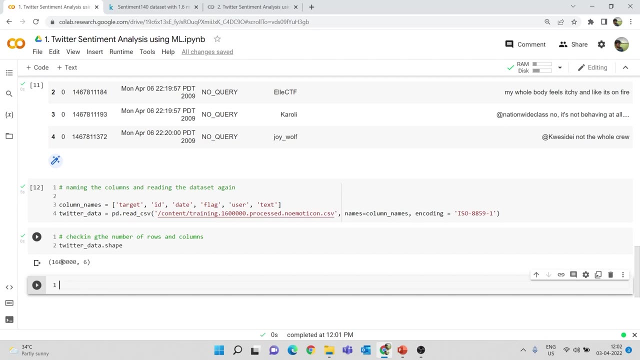 So this is actually the first tweet, but it was like read wrongly, So in this case we can correctly read this: like there are like 16, you know, 16 lakh tweets are there, or 1.6 million tweets are there, and we have like 6 column. 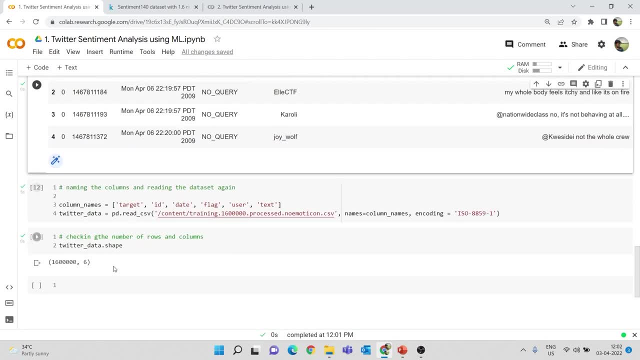 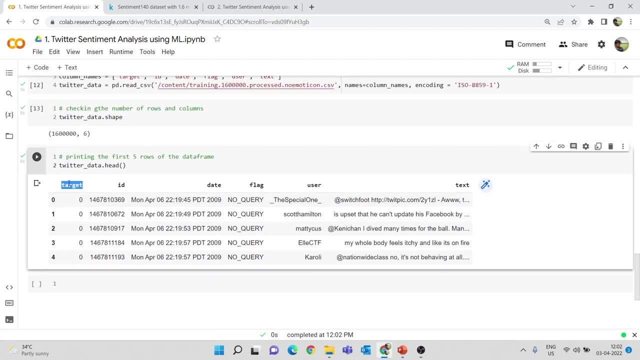 So I'll run this again. So now this will give me a different data frame, which as column names. okay, So, as you can see. So first column that we have is the target column, which contains the value as either 0 or 4.. 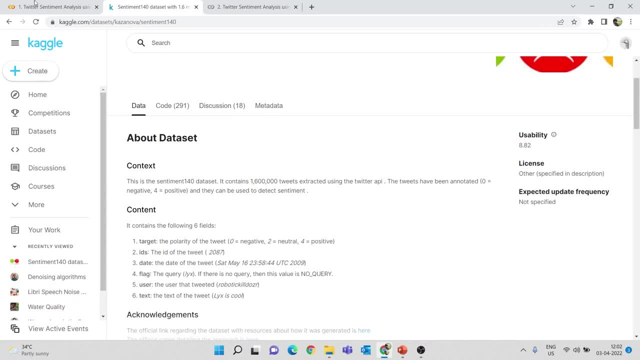 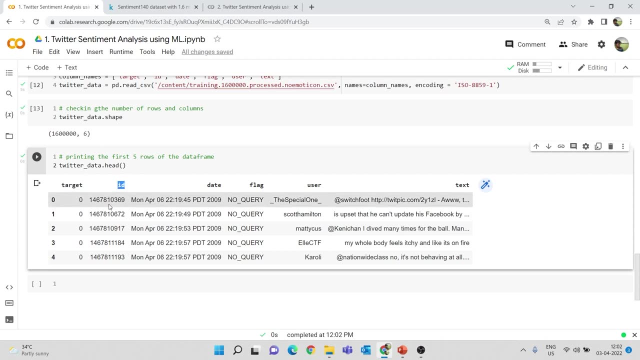 So, as you can see, so 0 means it is a negative tweet and 4 means it is a positive tweet. So this is the labels that we have, so we call this labels as target. and the second column: we have this ID, So ID for each of the tweet and date on which the tweet has been made, flagged whether there 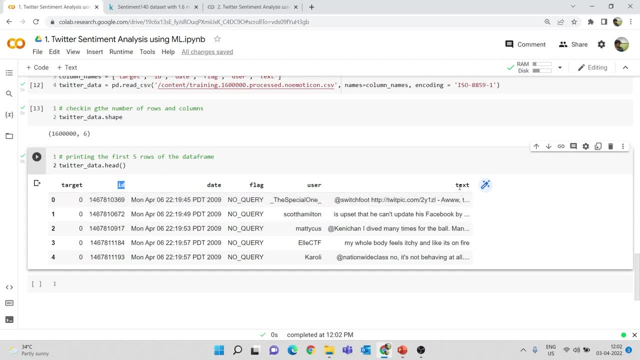 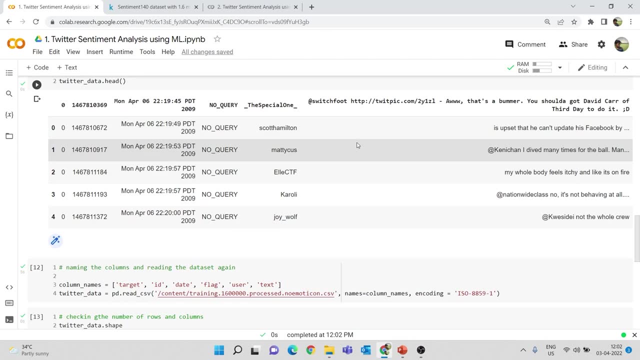 is a query or not. Okay, our name and finally, the text. so this text is nothing but the actual content of the tweet. okay, so we have loaded this data frame. so previously it look kind of look like this without the column name, and that's why we have, you know, included this column name and we have done. 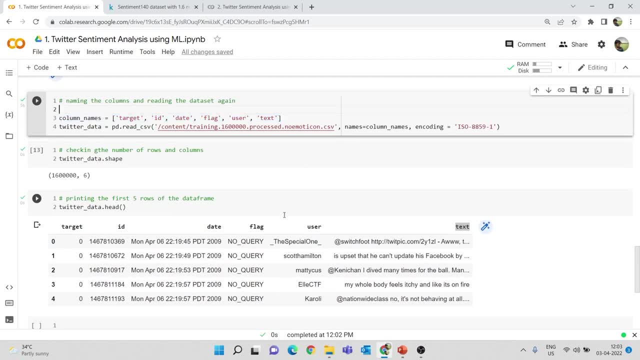 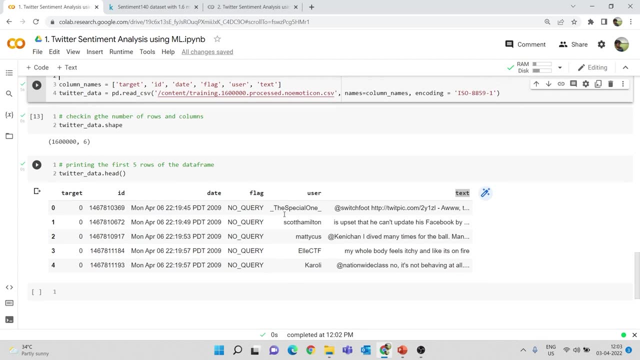 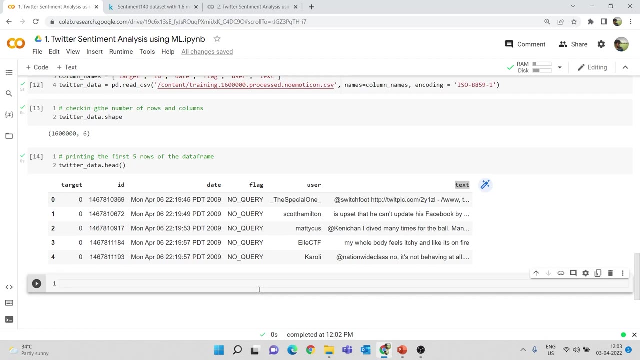 this, okay. so this is how you can load your twitter data from csv file to this data frame, and the next thing that i'll do is i'll check whether there are any missing values. the other important thing that we have to do is, like often when we, you know, deal with the data set in machine learning, a lot of 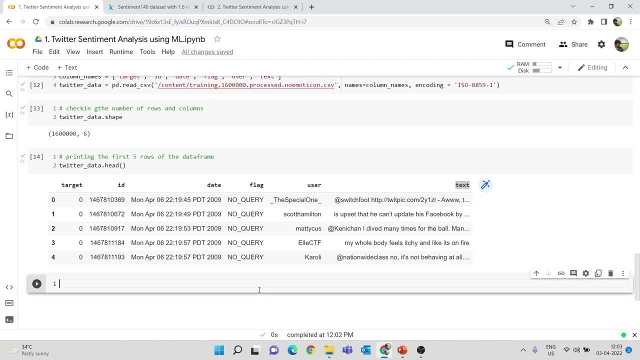 values will be missing. so if values are missing, we have to replace those values with some other values or we have to, you know, drop those values. so in this case, let's see whether any values are missing. so this part will be counting the number of missing values, missing values or text in this. 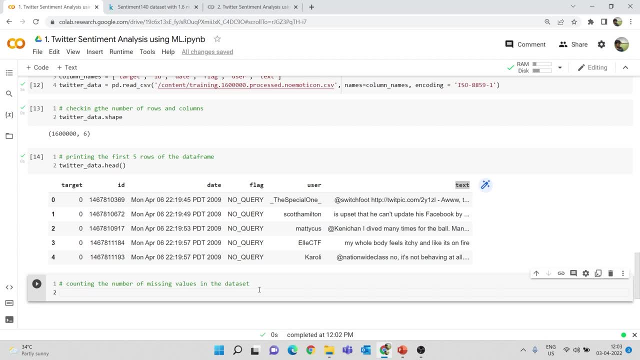 case missing values in the data set. okay, so i mentioned twitter data, which is the data frame name. uh, the data frame which we have created. so twitter data dot is null, so here i have to mention the parenthesis dot sum. so yes, no means. so null means missing values. okay, so i'm checking whether there are any null values using this external. 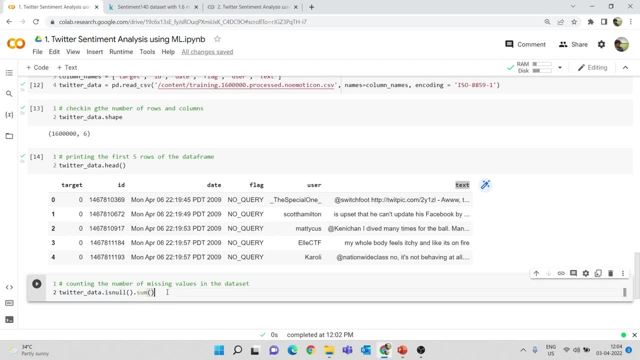 command- so this is null command- is present in pandas and i'm calculating the sum. so this will tell me how many missing values are there in each of the six columns. so we have six column right. so this function, so this code snippet, will tell me how many missing values are there. 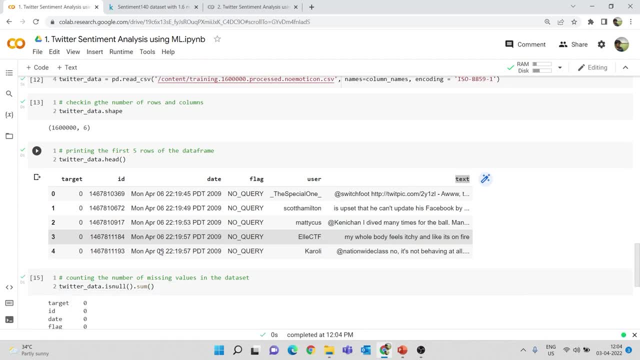 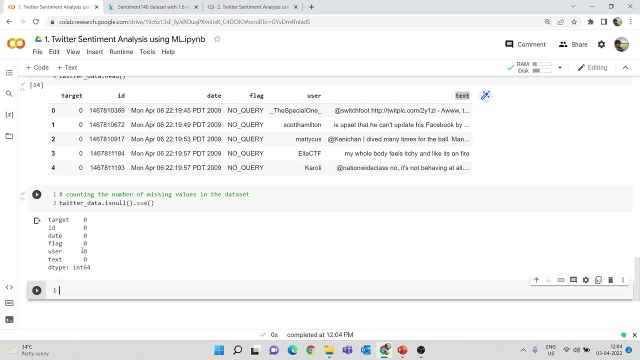 are there in each column, So I'll run this one. As you can see, all the values are zero, which means no values are missing in this case, And that is a fortunate thing, because we don't need to process this data set anymore. So all the values are present and then we. 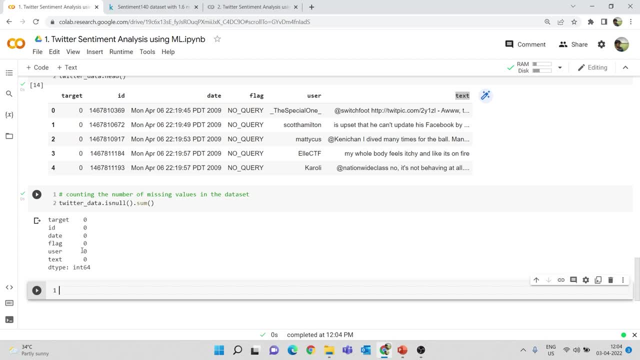 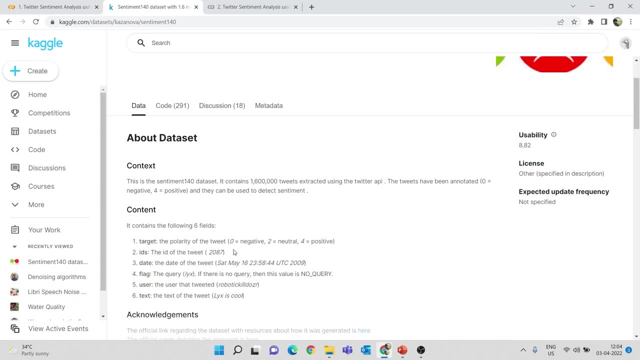 can move on to the other processing part. So now let's try to understand what is the distribution of this target variable. So here it is mentioned. as you know, zero means negative and four means positive. So here they are mentioned as like. there are like three labels. 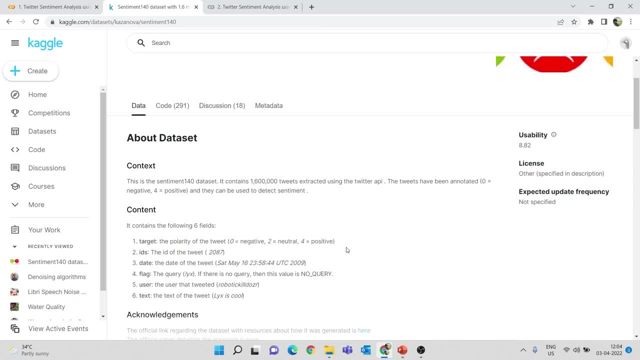 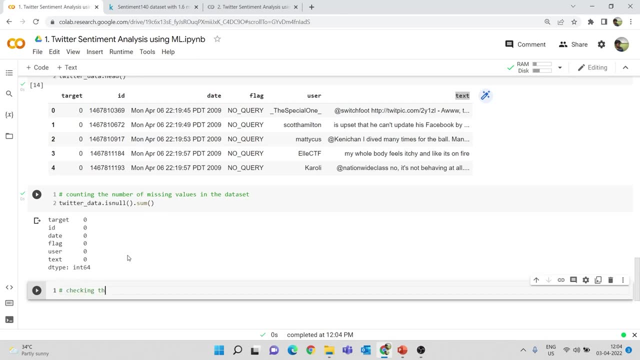 zero as negative. if the value is two, it means neutral, four means positive. let's see how many labels are there. So this will be checking the distribution of target column. So this is basically to check how many positive tweets are there and how many negative tweets are. 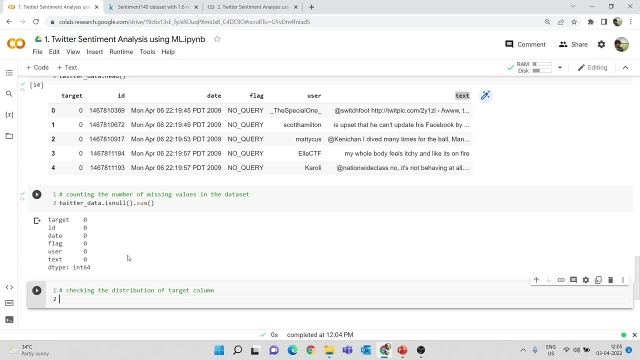 there in our data set. So totally, there are like 1.6 million. So how many you know? positive and negative tweets are distributed in this data set. So for this I have to run this one, So let's run this one. So let's run this one, So let's. implement that. So he forgot about roaming. let's run that one. He forgot what his version is based on, what distribution, so let's see what this is, And then what we're going to do is go into data sets and see what we will see, For today we are going to do is simple. number circuit. So we are just going to do and also mark this code was part. You're paying attention. So here you can enter the früher into with suburif, which is less than zero of course. So again we are going to do another function, to map. This time. I mean this is called target tags. So here we are going to go inside the tag persons first, And that's the current result. So I have here the target to be 2.2 million. So keep on skipping right. so you have toent que it. let's click on the target and you. 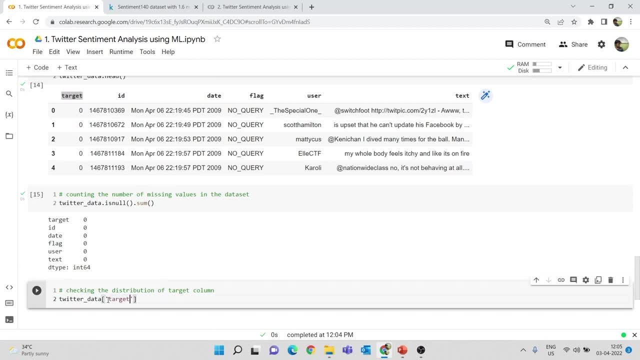 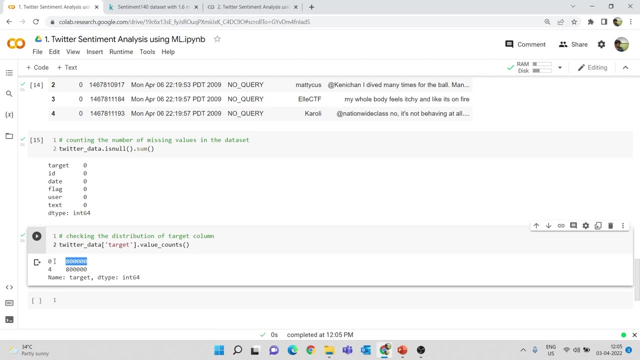 within this parenthesis, i have to mention the column name, which is target and dot. value counts, so this will count: the number of values of zero and four. so value counts. parenthesis, let's run this one. so, as you can see, the number here is eight lakhs, so eight lakhs tweets are there for. 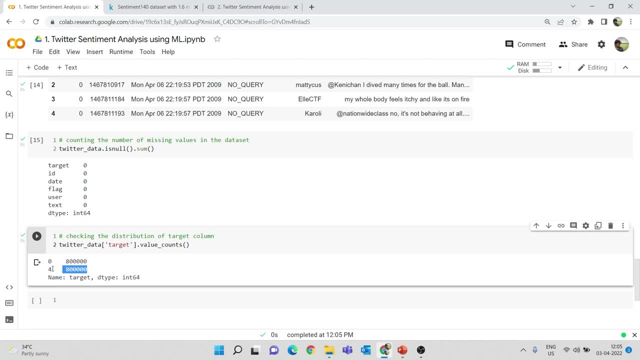 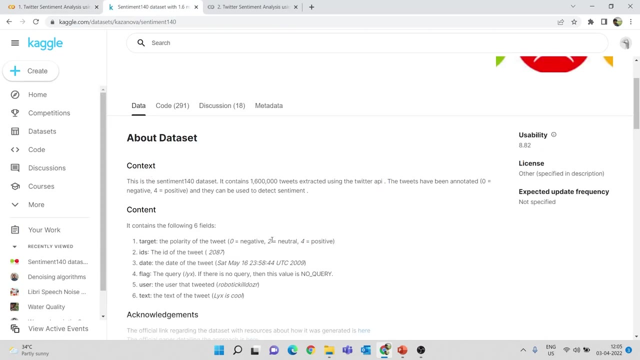 the label zero and eight lakh tweets are there for the label four. so when you add this, you the total value is like 1.6 million. so that is like a very equal distribution of the tweets that we have. and if you go here, so we have like the annotations as zero as negative and four as positive, but in 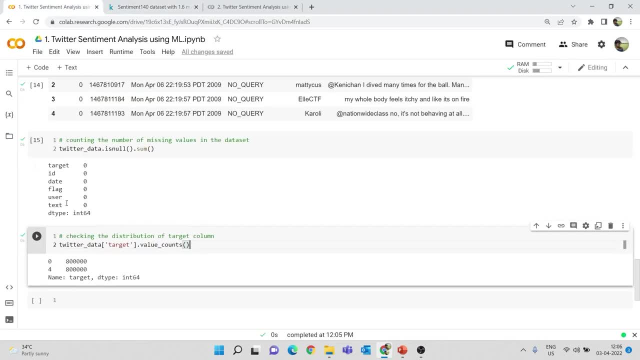 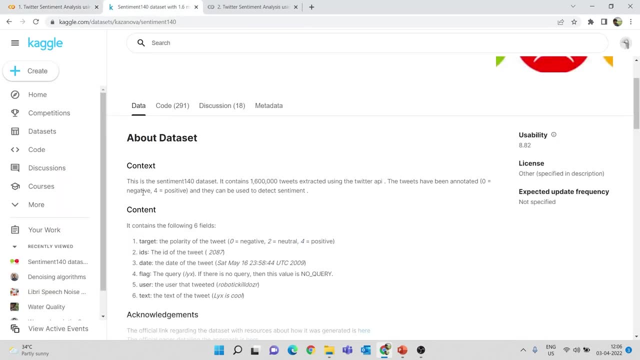 this case, they have given us neutral, but this is an error, because the data set contains like only- uh, you know- two labels: one is zero and four, where if the label is zero, that means the tweet is a negative tweet and if the label is four, then it means the tweet is a positive tweet. so that is. 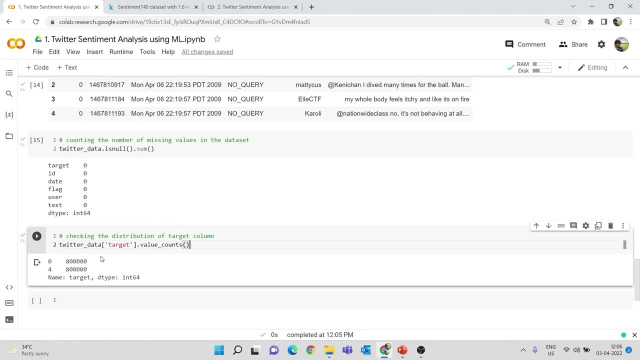 the inference that we can get and the data has been equally distributed. so that reason for performing this operation is that if the distribution is not even, we have to do things like up sampling and down sampling to make this distribution as even. so, if you work with an 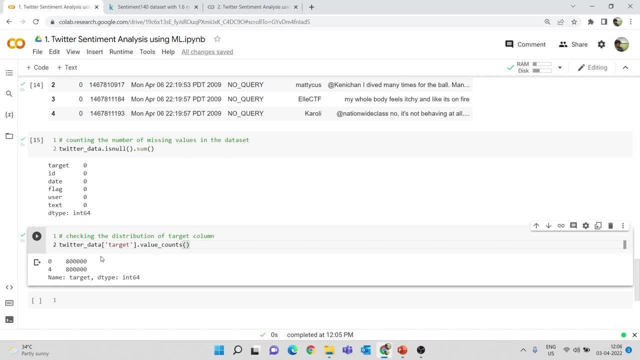 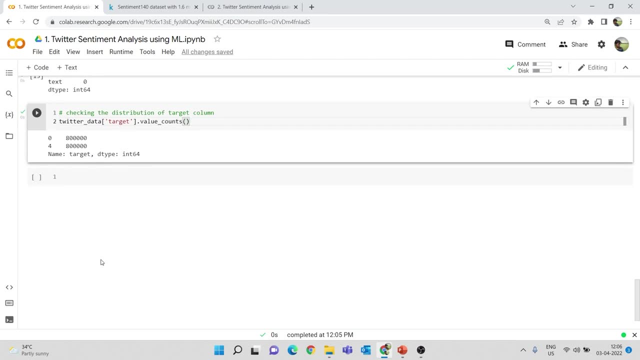 uh, you know, uh, data set that doesn't have even distribution. in that case, your machine learning model won't work properly. so this is a very important step that we have to check. in this case there is an equal distribution, so we don't have to do anything yet. so these are like very 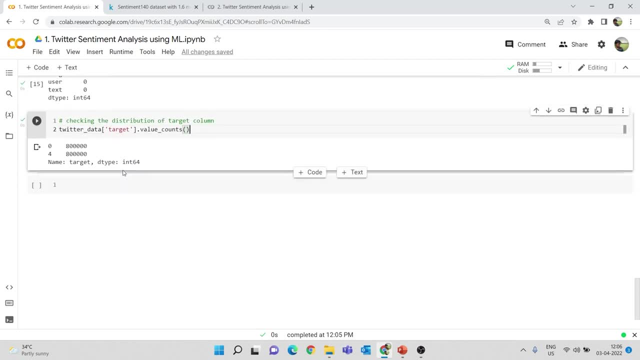 important: checking whether there are any missing values and whether the distribution is even or not. so we have, we will perform these things in you in any machine learning use case that we do. okay, so now what i'm going to do here is: here the label is zero and the label or the other label is four. so i don't like this label, so it is not a good way. 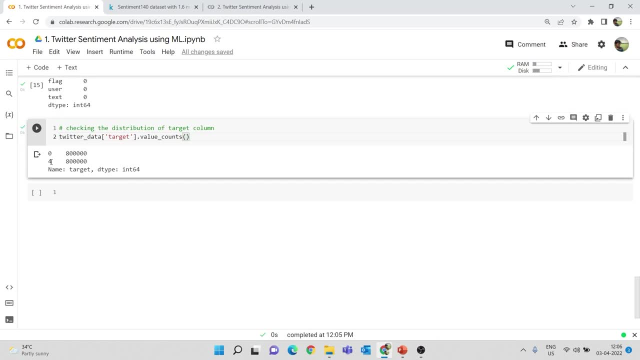 in order to have the labels as zero and four. so what i'm going to do here is i'm going to convert this four to one, okay, so that i will have the labels as zero and one, where zero means a negative tweet and one means a positive tweet. okay, so this part will be. i'll make a text here as: 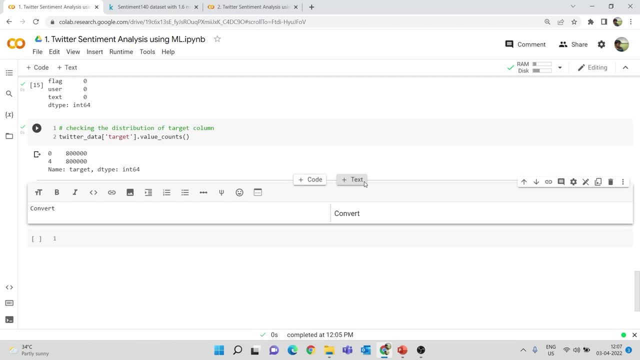 convert the label or the target. convert the target four to one. okay, so four to one, okay. so this is the conversion that we are going to make. so i will mention twitter data. so all these things comes under data preprocessing. so that's why i told you like we. 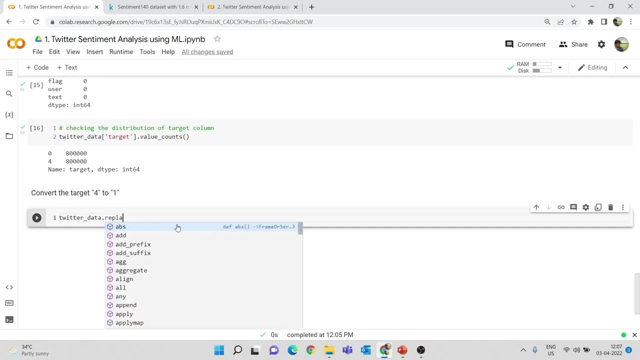 cannot feed the raw data to our ml model, so we have to perform various processing things. so twitter data dot replace. so within this parenthesis we have to mention what we are going to replace. so open a curly bracket and i'm going to say target. target of four colon, one comma in place. 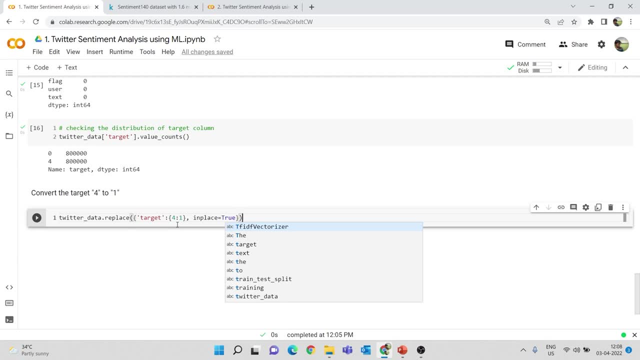 equal to true. okay, so let's try to understand what we are doing here. so, basically, i'm taking this data frame and i'm going to replace certain values. so i'm going to replace the values in this target column. so how i'm going to replace this? i'm going to replace all fours to one, so this: 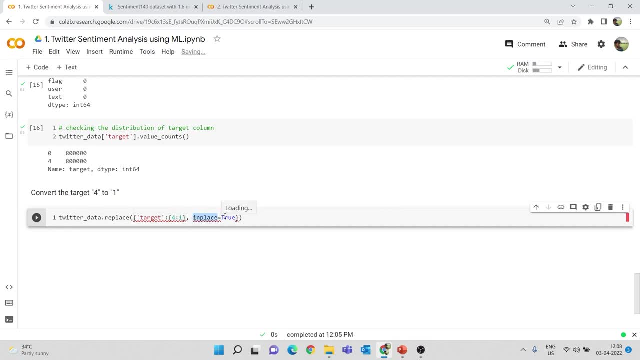 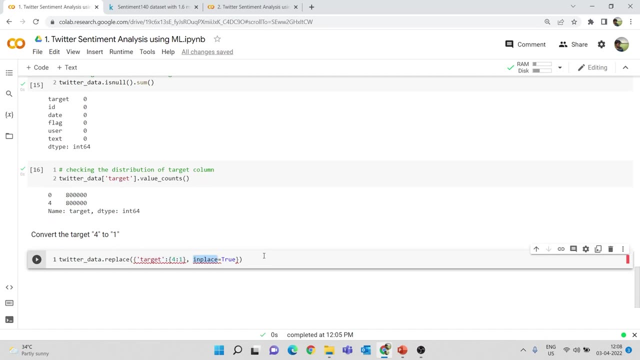 is the conversion that i'm making and i'm mentioning this. in place is equal to true, so in place is equal to true means. so this change has to be stored in my original data frame. so if you don't do this, in place is equal to true. this change of replacing four is two won't be stored. 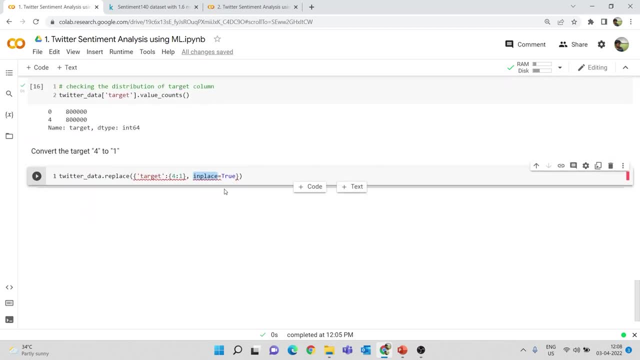 in your original data frame, which is your twitter data. so including this invoice is equal to two is very important, so we are doing this, converting all the values of 4 to 1 within this target column, so I will run this one. okay, so invalid syntax in place is equal to true. 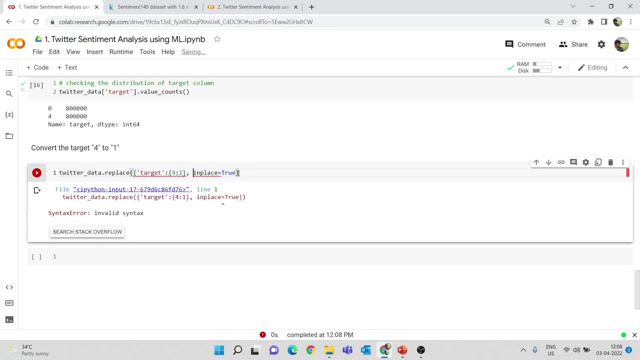 okay, so we have another curly brackets. okay, so we have the opening curly bracket and ending curly bracket here. so this is actually in the form of a dictionary, so this is a python dictionary data type. so I have wrongly included another- you know curly bracket here. so that is why we 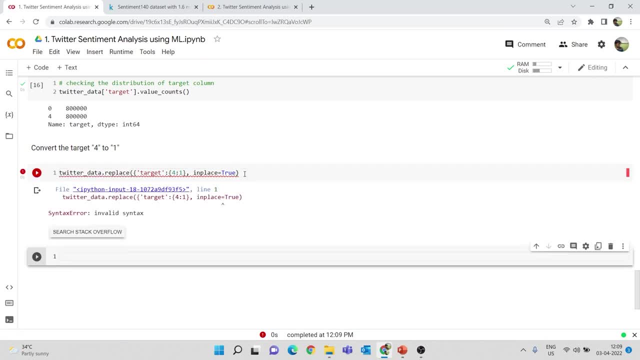 are getting this error, so I will run this cell again. okay, in place is equal to true, so I am getting this error again. let me check the twitter data dot. replace target s2. uh 4 is to 1, okay, okay, okay. so the thing is here: we have one curly bracket and we have another curly bracket here. 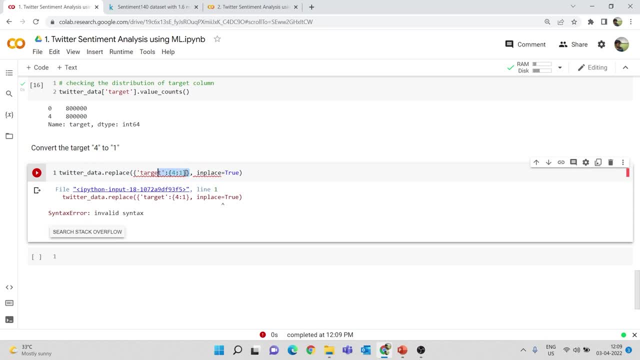 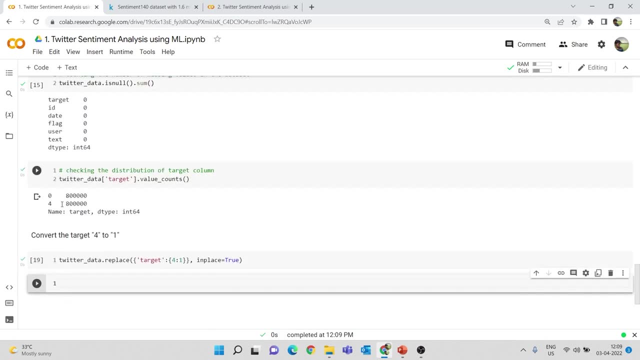 so we have to close the curly bracket here. so this is the error that we add. so let me run this cell again and check whether this is working properly. yeah, so this cell is executed. so previously, as we can see here, the two values that we add in our target column are 0 and 4. now i'll 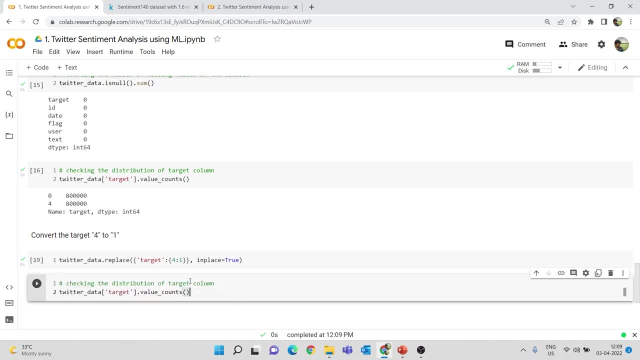 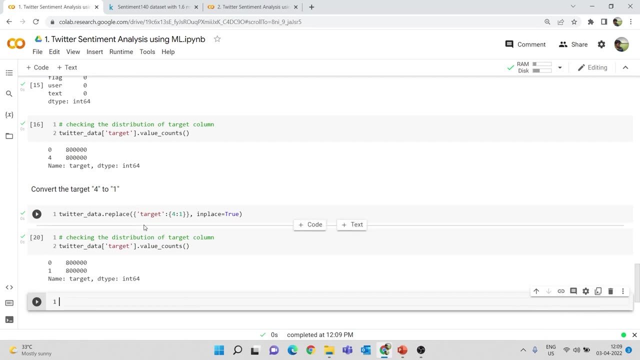 just copy this one and i'll paste it here and i'll run this cell again. so now all this four values has been converted to one. so this is the basic conversion that we are doing. so we have like eight lakhs tweets, or 800 000 tweet, which has a no negative emotion. 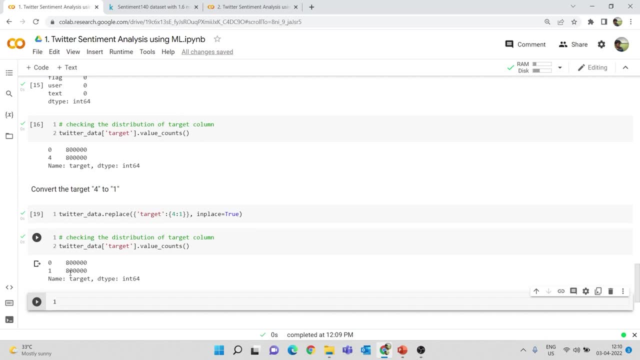 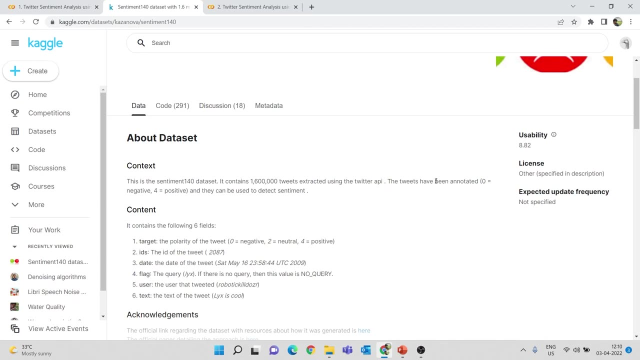 attached to it and 8 lakh tweet, which has you know, positive emotion attached to it. so we have just replaced this, you know, 0, this asset. so we are not doing any change in the label 0. we are just changing this 4 into 1, so it means like, if a target value is 1, that 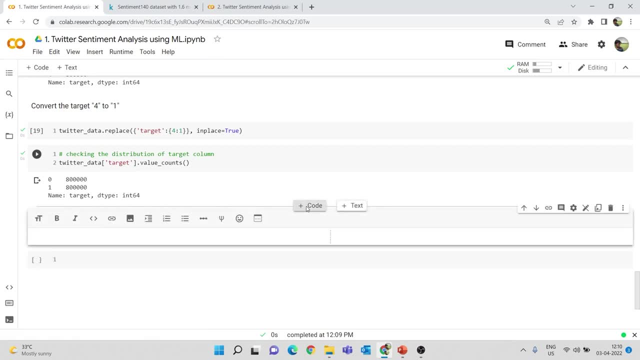 means it is a positive tweet. so i'll make another text here, as 0 means negative tweet, okay, and let's say, if it is 1, that means it is a positive tweet, okay. so this is what the machine learning model is going to understand, whether the tweet is a negative tweet or it. 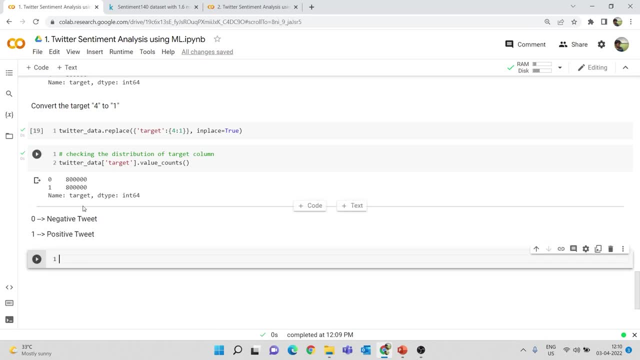 is a positive tweet. so we will be training it with the 1.6 million tweets that we have and then we will, you know, test it for evaluation, and the next thing that we are going to do is called as stemming. okay, so i'll make a text here as stemming. then i'll just make 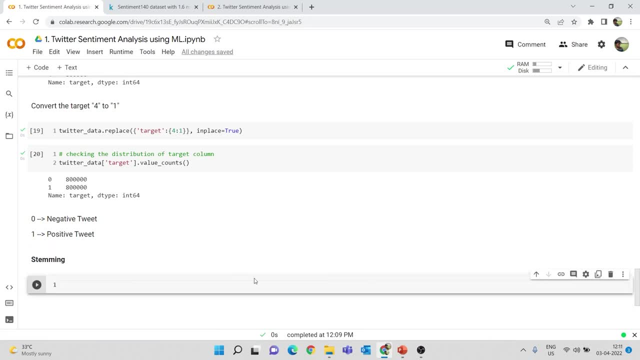 this in bold. so for this purpose only, we have imported the function called a spotter stemmer. so I'll explain you what is meant by the stemming. the stemming is a process that we do in order to reduce a word to its root word. okay, so I'll. 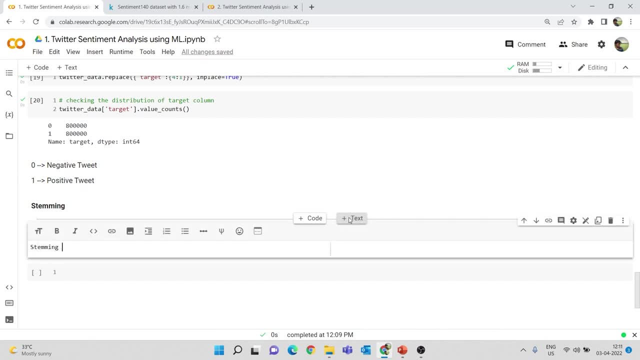 just put that definition here as well. the stemming is the process of reducing a word to its keyword, or let me name this as a root word. so root words are nothing. but let's say there is an example, so I'll just give you an example for this. so let's say that there is. there are like words, like actor and you. 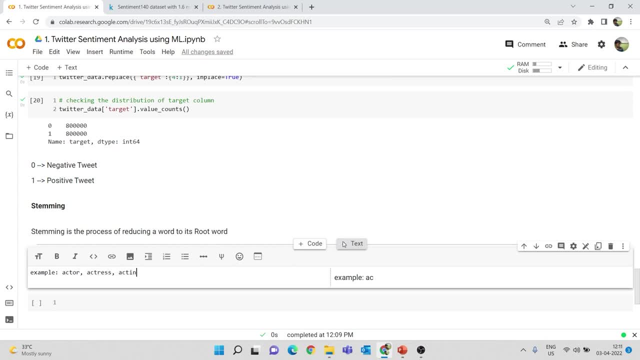 know, let's say actress and acting, so these are like words that are similar meaning, right? so we kind of take all these words and change those all this to those keywords, or what we call as root word, called as act- so I shouldn't use the term keyword, so we have to say root word. so the root word for actor, actress and 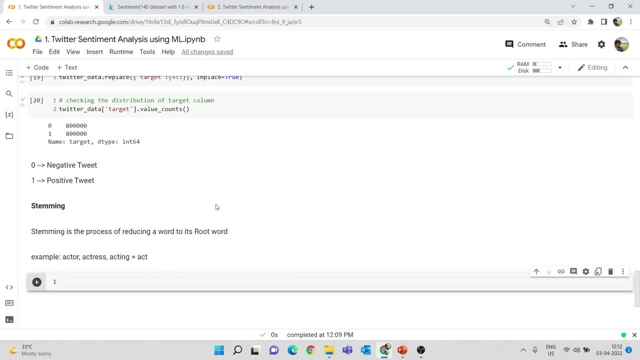 acting. all these things are act. so the reason we are doing this is, as we know, that the data set is very huge and we have to do some processing in order to reduce the- you know- dimensions and the complexity of the data. so we are taking all the words and then we are reducing the these words to its root word, so that 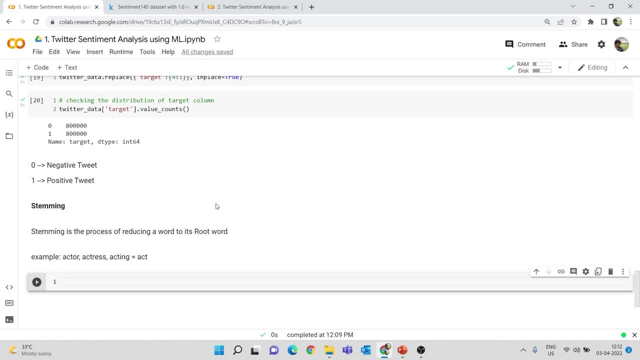 it is easier for our machine learning model in order to go through the data and understand whether the tweet is a positive tweet or not a negative tweet. so this is a very important part, you know, in this sentiment analysis where we are taking each word of this tweet. so there are like 1.6 million tweets, right? so we are taking each 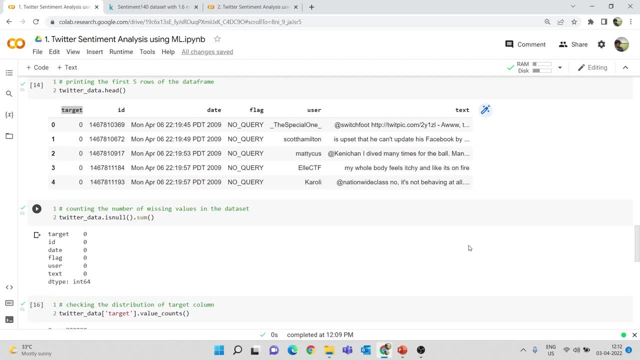 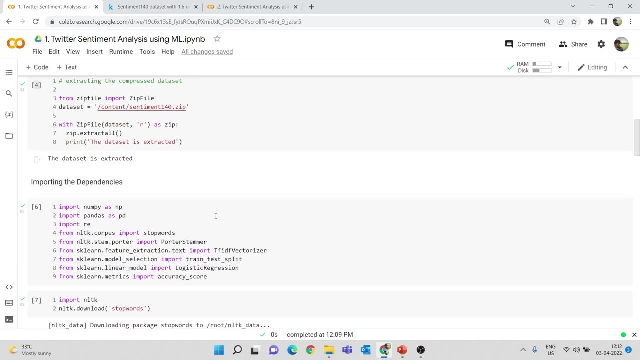 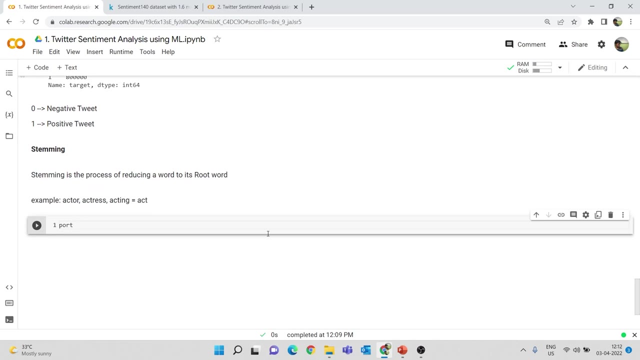 word from each tweet, and then we are, you know, kind of reducing it to its root word. so that is what we are doing here, and for this I am going to use the potter stemmer function that we have created. so potter stemmer. so I will create a variable as pot stem. so this is where we are. 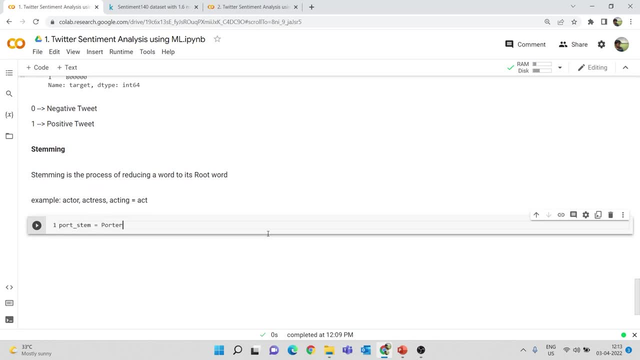 going to load the instance of this potter stemmer function that we have imported, so potter stemmer in parenthesis. so this will load the instance of this potter stemmer module, or the function which I imported to this variable, called as pot stem. so I will run this one, and now I am going to create. 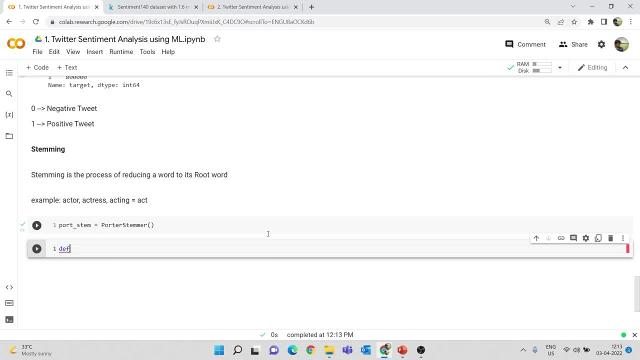 a function. so we know that in python we use this term, def, which stands for define, and this is used to create some function. so I am creating this function, called as stemming, and I am going to say content, right, okay, so content. and so when I call the stemming function, I want this: 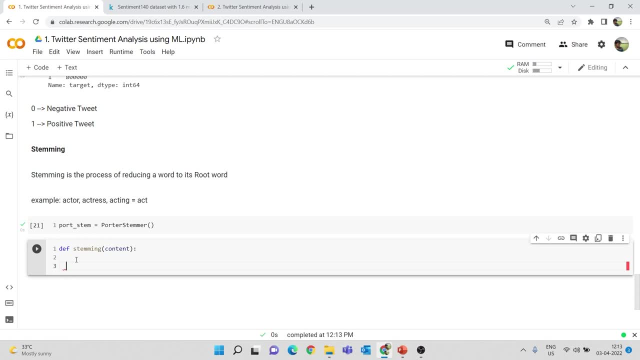 you know, process to be completed, which is like reducing the word to its key, to its root word. so I will create a variable called as stemmed content. stemmed content is equal to resub. so this resub is nothing. but so we have already imported our regular expression expression library. so the short form for regular expression is resub. so from this, 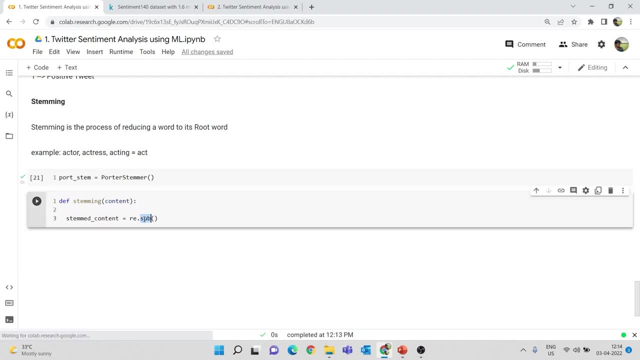 regular expression library. i'm importing this uh sub, the sub module. i'll explain you what uh, this particular sub function does. let me just complete this one. so i have to mention codes, i have to mention a list with opening square bracket and closing square brackets. i have to say 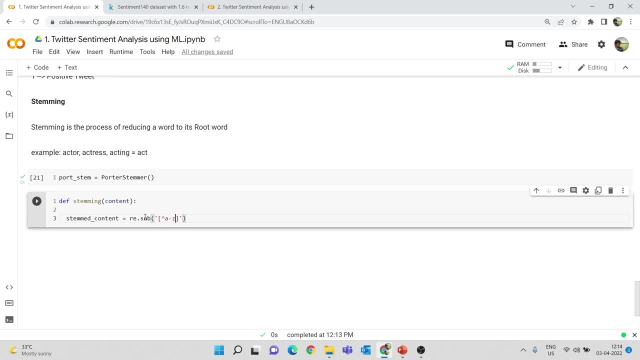 uh, upper arrow head. a to z capital. a to capital. is it later? i have to say this: codes: there has to be a space, later has to be this content. so i'll explain you what we are doing here. i'll just, i'll just complete this particular function. i'm going to call this stemmed content. 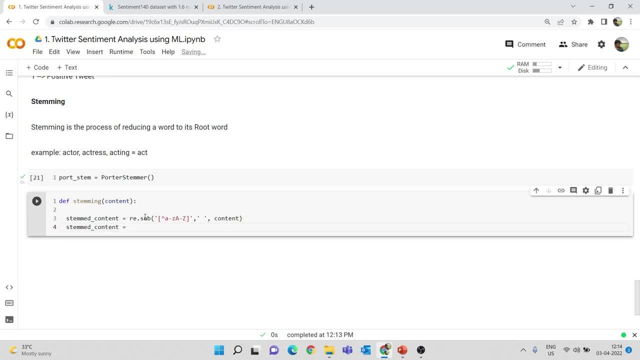 again, stemmed content is equal to. i'll copy this one: dot lower. okay, so lower in the sense we are converting all the uh uppercase letters to lowercase letters because we don't need this. uh, you know, uh, we don't need a letter to be uppercase in order to do this processing if it is in lowercase. 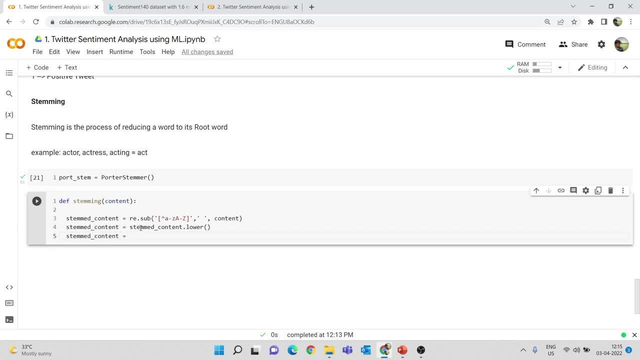 it is sufficient for us. that is why we are converting that and i'm going to say: stemmed content, dot split. so once we do this stemming operation, we have to split all those words into like. so we will split all these words and we will store it in a list. 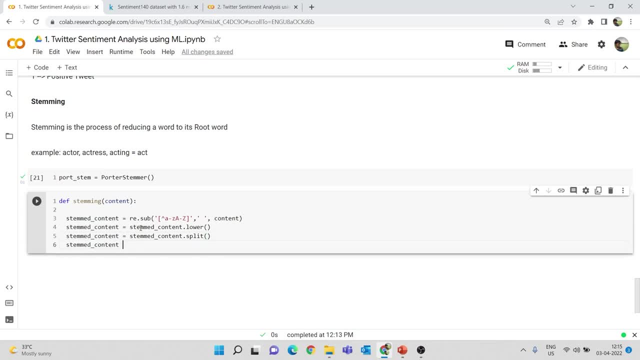 so i will explain you in detail about this later. and the stemmed content is equal to. so this is where we are going to use the port stem function that we have: stem dot, stem word for word in stemmed content, if not word in stop words. so this may look. 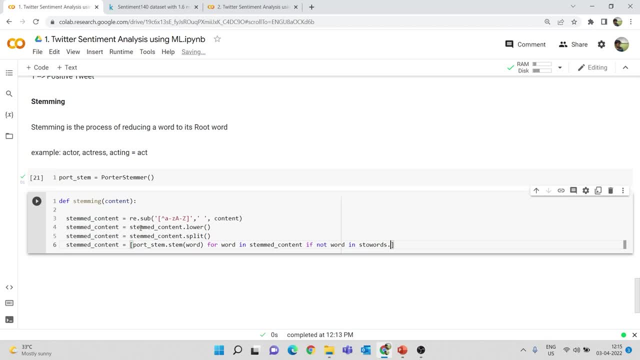 a bit complex, but this is actually very simple. i'll explain you in a moment. contentwords, english. okay is like one more step, which is: stem the content is equal to space, dot, join, stem content and finally, we can, you know, return this stem the content. okay, okay. so when i call this, uh, stemming function, i want all these processing to take place. 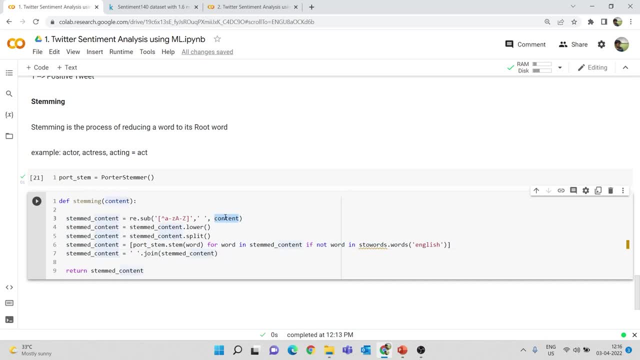 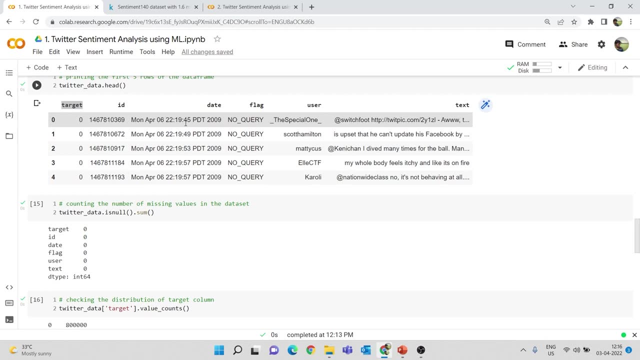 okay. so what we are doing here is so content is nothing. but so in this content, within this function, we are going to pass this text column. so text column contain all the tweets, right, so we are going to pass these tweets because we do not need any other you know column, so we just need this target column and this text column. 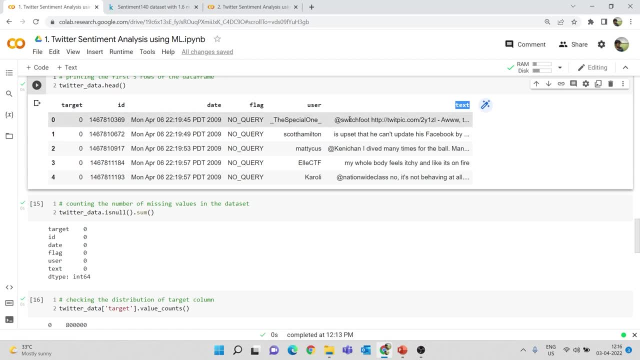 which is basically the tweet, so we do not need anything else. and I am going to process all these texts because, like this target is already in the form of numerical value, right, either 0 or 1, so the machine learning model can understand it, but it cannot understand this text. so before converting: 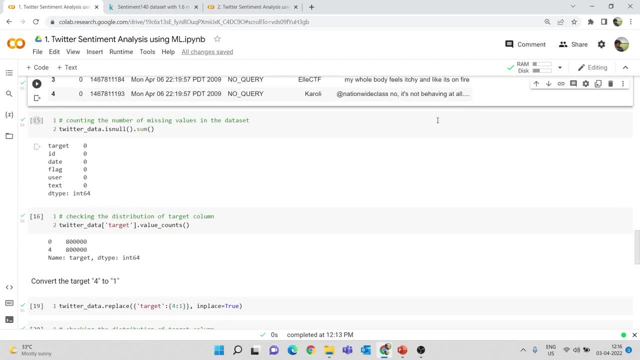 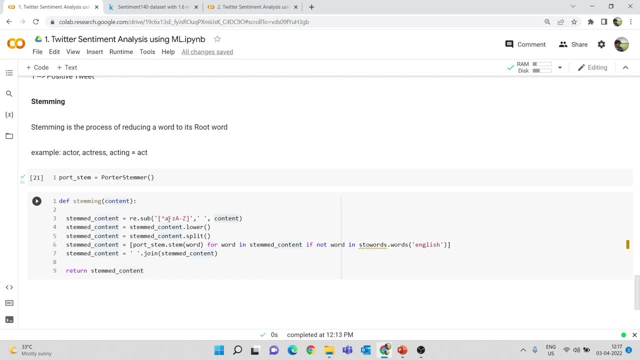 this textual data into numerical data, we have to do some more processing, and that processing is called a stemming, which is to reduce a word to its keyword. so before doing that, we are doing some, you know, some you know like few other steps here. so I am taking like the content. so here the content. 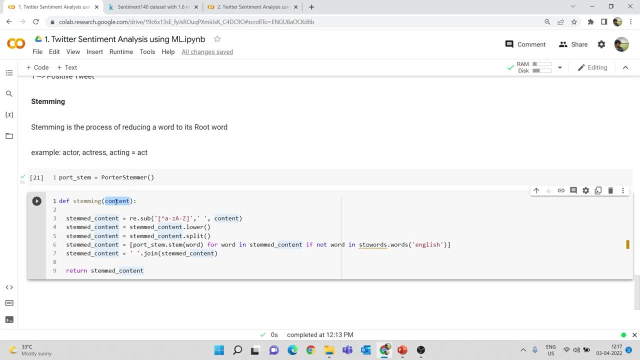 is nothing but each tweet that we have in a data frame. so all this 1.6 million tweets will be processed individually. so first thing we are doing here is resub of a to z and capital, a to z and content. so we are taking this content and I am going to process this text column and I am going 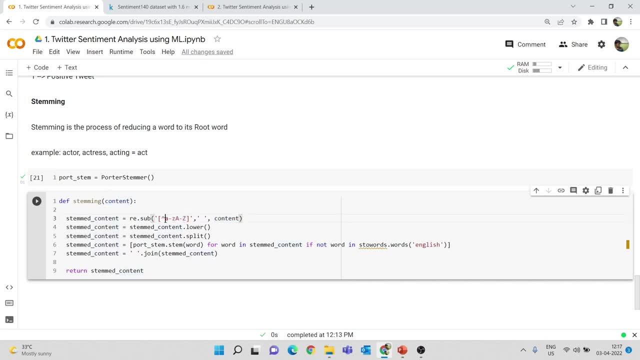 to remove all the things. that is not alphabet. so when I say a to z, so lowercase a to lowercase z, that means like all the alphabets, like lowercase a to lowercase z, all the alphabets. and this capital a to capital z means all the you know uppercase letters. so, and this means this upper arrow it. 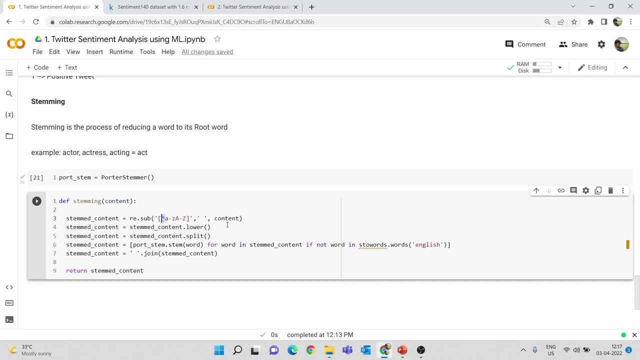 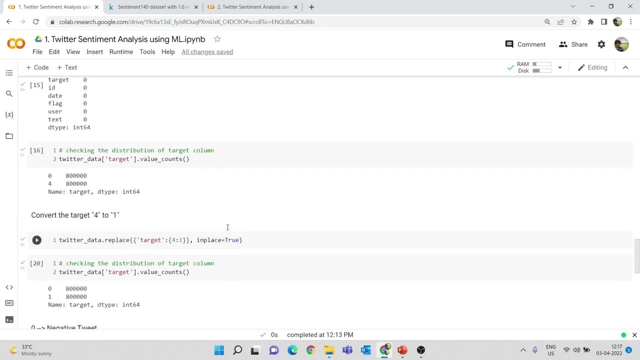 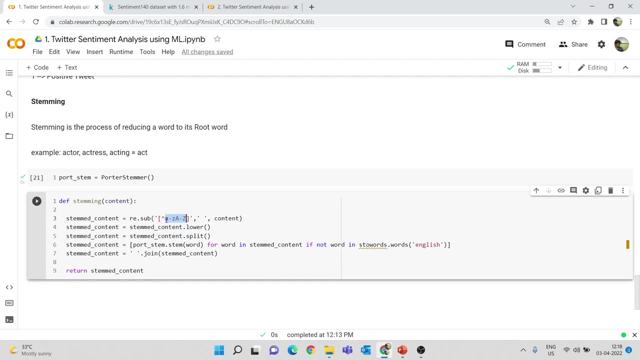 means I am going to remove those words. so upper arrow it. you can just press shift plus six in order to get this arrow it, as you might know already. so I am going to take each of this tweets and I am going to remove if it is not this, if it doesn't belong to this list. so this is: 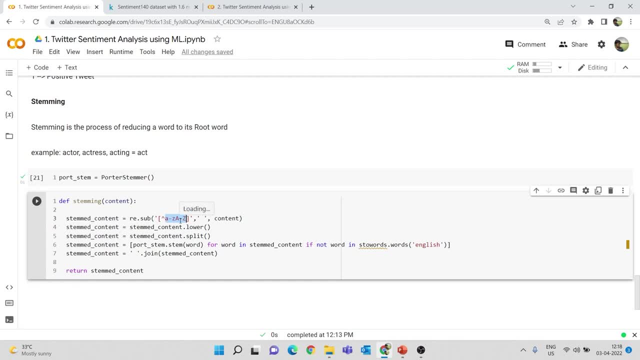 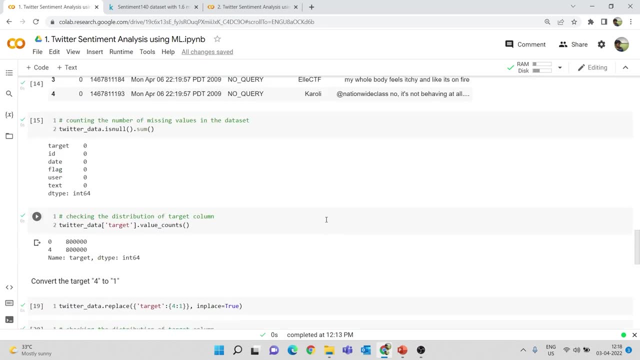 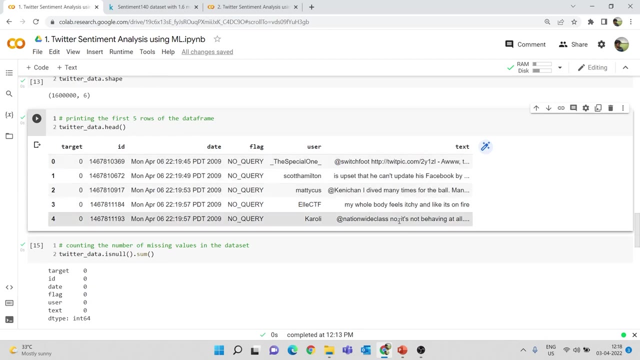 nothing but small a to small z, and this is like capital a or uppercase a to uppercase z. if a word or a letter doesn't belong to this one, I am going to remove it. okay, so if you see this one, we have this at symbol, right, so this will be removed and we have this. number two is there, and some. 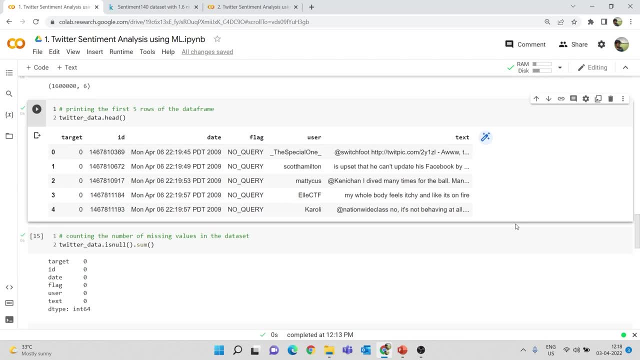 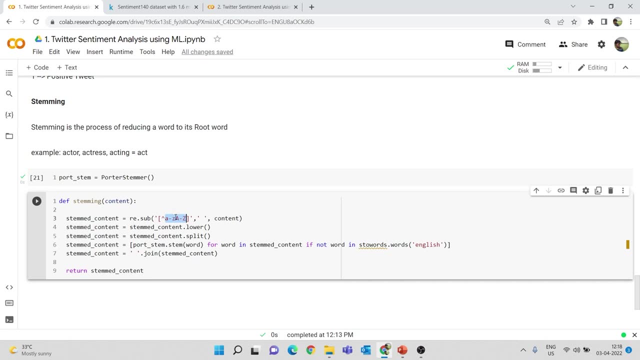 punctuations are there, so we are going to remove all the things. that is not a letter, so that is here. so this is the list that we are considering. so we are just matching some patterns. so the pattern that we are matching here are letters, so alphabets, english alphabets. so when I say this: 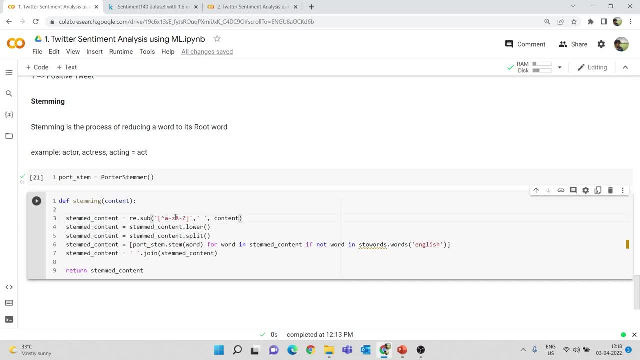 upper arrow it. that means I wanted to remove everything that is not a to z, or this capital a to capital z. so that's what I am doing here. so once you pass this content, so each tweet will be processed each time this function runs and we, kind of like you know, remove all the things except for. 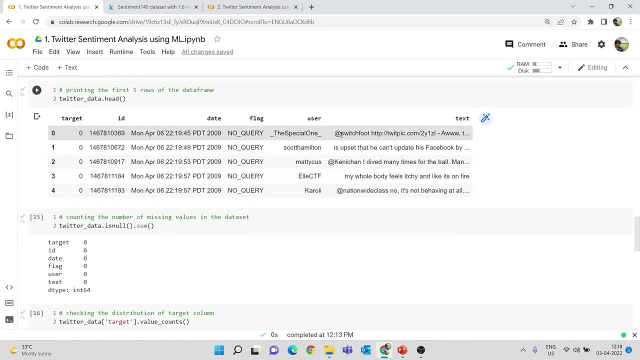 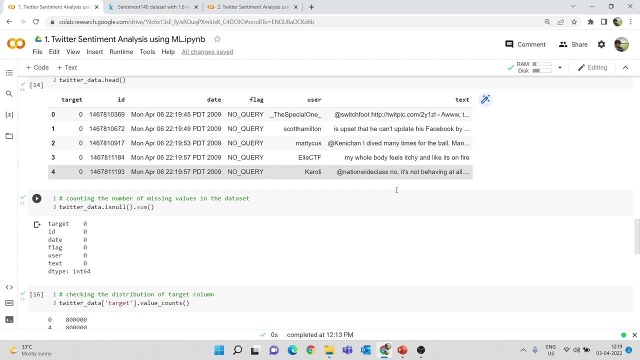 this. so if it is, it is at symbol, or if it is like any other special characters, or it is two, or if it is a punctuation. we kind of remove all those things, because we don't need all these things in order to understand whether a tweet is a positive tweet or a negative tweet. so that's the reason. so that is. 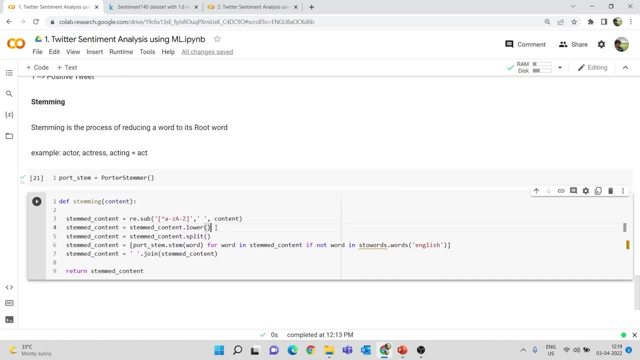 the first step. after that, we are converting all the letter to lowercase letters because we don't want the uppercase letter. so if we you know, it doesn't add any meaning to the context of the tweet. so a letter being like a capital letter, or in other words an uppercase letter or a lowercase. 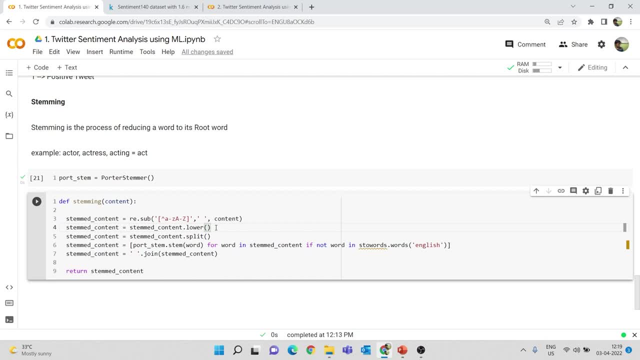 letter doesn't influence the context of that particular tweet. so we are going to convert all the letters to lowercase letters and once we do that, we are going to split all the words from this tweet and we are going to load that into a list. so that's what we are doing here. so I'm going 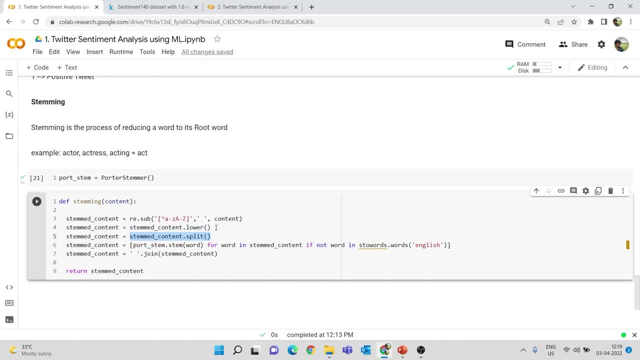 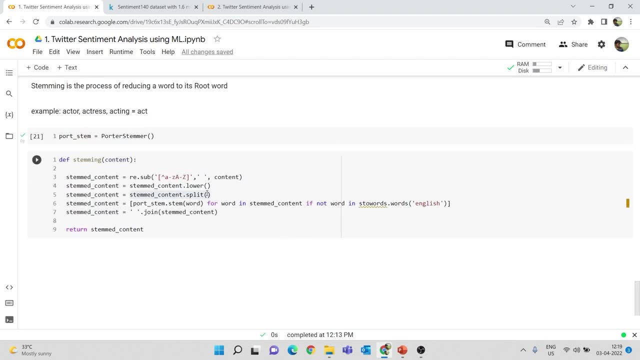 to split all, all the words in a tweet and I'm going to put that in a list. so if you consider this one, so the first word will be in in the list and the second one will be in the list, and so on. so that's what we are doing here in this dot split uh function, and after that we are using this pot stem. 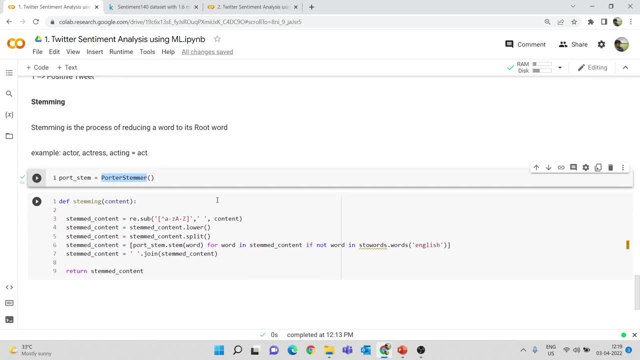 of this pot stem is to reduce a word to its root word so that we can save some space. you can, we can make this processing easier. so here, what I'm doing here is pot stem, dot stem of word for word in stem content. so stem to content is nothing, but so this is where we are storing all this processed content. 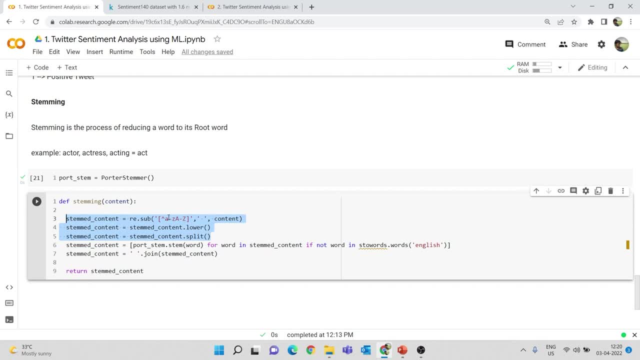 so first, we are like removing all the special characters, numbers and punctuations and all those- uh, you know, content that we need has been stored in this template content. so this template content will contain only letters and words, so it doesn't contain any numbers or special characters. after, 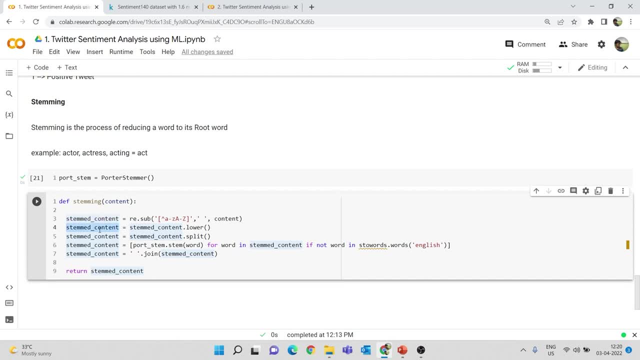 that we are converting uh into lowercase letters and that will again be stored in the stem content and then we are splitting it to a list. so once we do that, we are taking each word in the stem the content and we are checking if that word is present in the stop words. so it should be stop words, as we 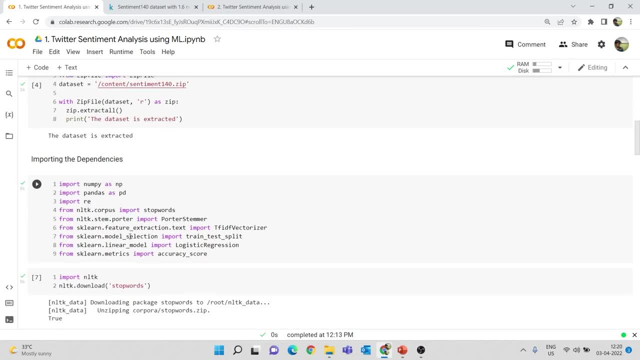 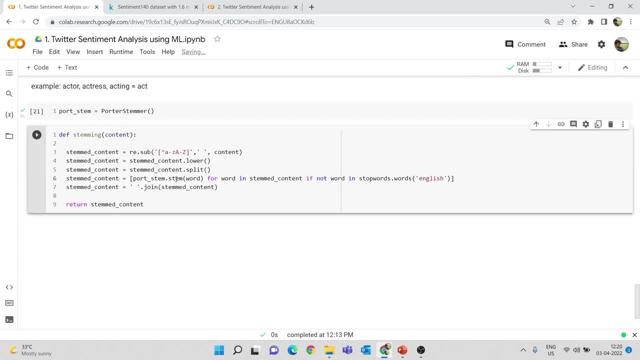 know that stop words are, uh, nothing but the words that we don't need. that doesn't add that much meaning to the context of that week. so these are the stop words. so when I say pot stem, dot, stem of T word, so what words I'm going to? uh, you know, do the stemming operation is for word in stem content. 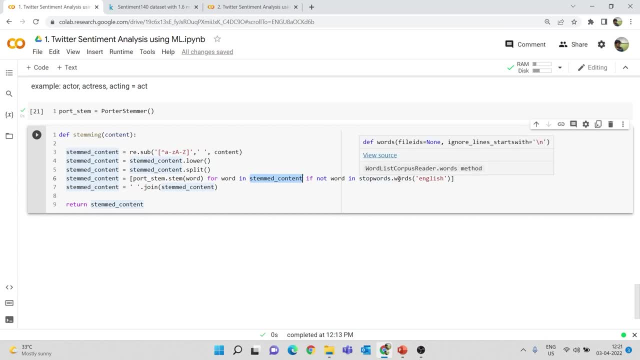 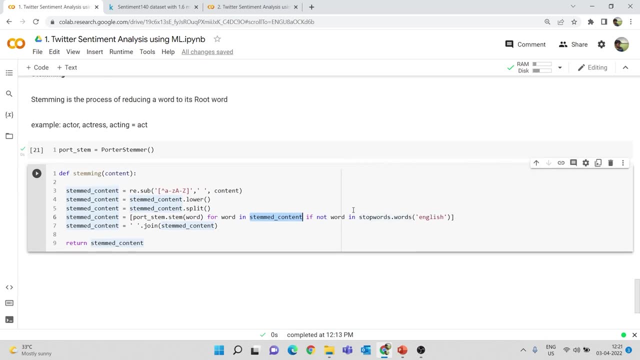 if not word in stop words, dot English. so if a word doesn't belong to the stem words, and then in that case I'm going to process the stem content, because it's like there is no meaning in performing this uh stemming operation and uh for the stoppers, because we don't need those stop words, so that 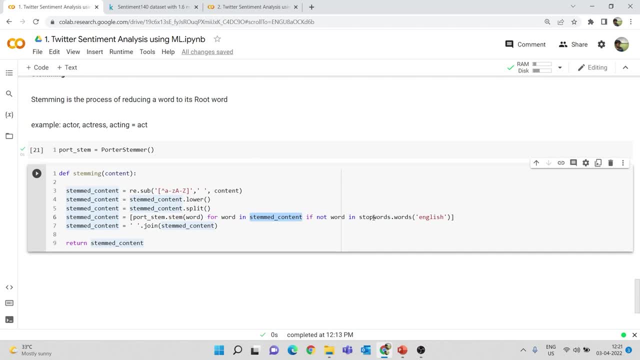 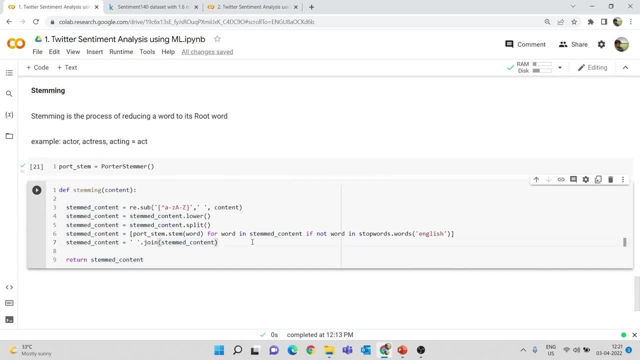 is the reason. so if, if a particular word is not in the stop words- stop words are nothing but this- I me, my myself. so in that case, perform the stemming operation. okay, so if the word is present in the stop words, in that case I won't do the stemming, I will just basically ignore those words and I will just join all those things. so this: 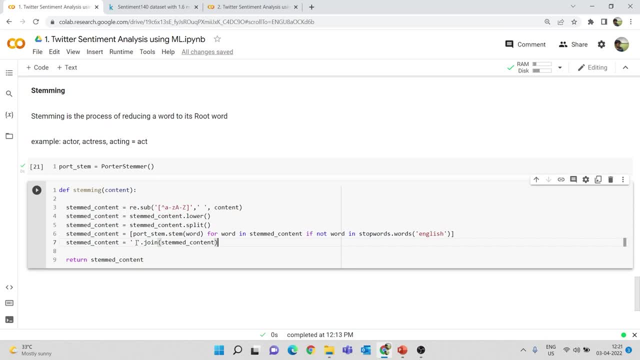 is like again joining all the tweets together. so let's say that, uh, first tweet is there and there are like 10 words in a in that particular tweet. after you know, doing all this processing, we will combine this tweet together. so in this step we are splitting each word and the stemming operation is. 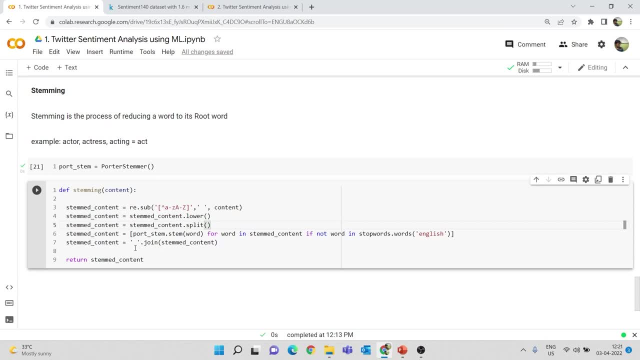 done. we will join all the words in a particular tweet. so let's say that there are like uh, you know, as I've told you, words in a tweet, so in that tweet, when this uh function run, we will remove all the punctuations and special characters in that first tweet and then later we will- uh, you know, kind of replace. 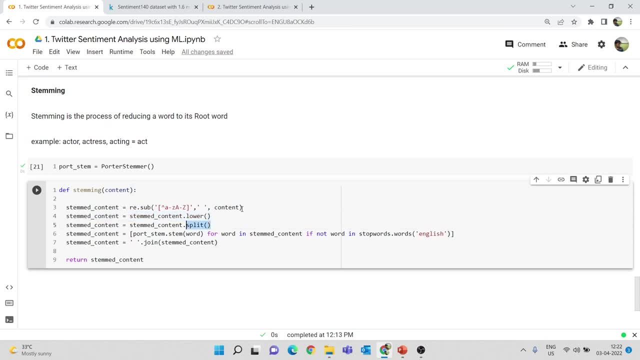 all the uppercase letters to lowercase letter. later we will split all the words into a list so that we which contain 10 words will now be converted to a list and that list will contain 10 individual words from that list. after that we will check whether that uh words present in the tweet. 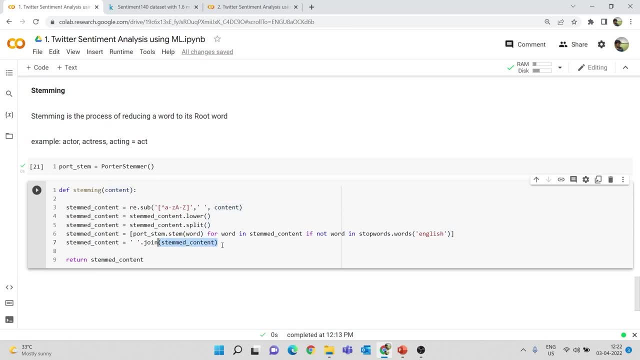 we will perform the stemming operation and we will join this- uh, you know- words- back so that we know that it is one particular tweet. so this is the process that we do: first we will check for special characters, numbers or punctuation, later we will convert it to lowercase letter, then we will split. 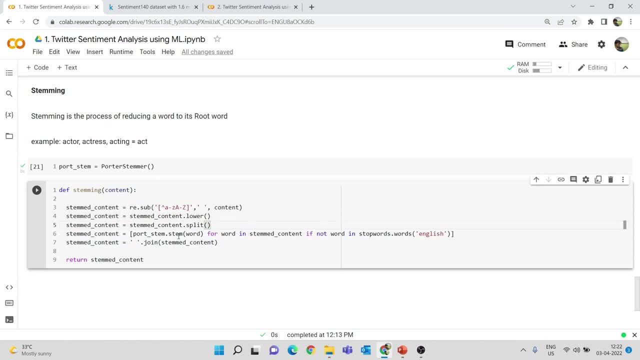 each word individually, and then we will perform this stemming operation individually to this words. so, once this has been done, uh, each tweet will be joined. so I'm not telling that all 1.6 million tweets will be joined, so I'm not telling that. so, when you are performing this, uh, individual words in. 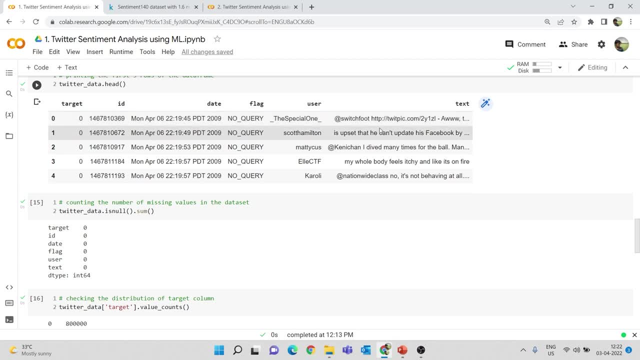 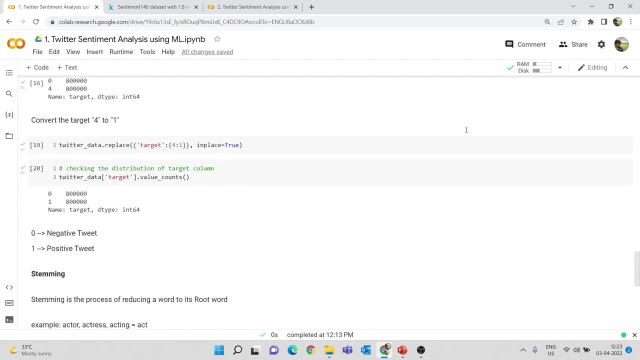 each tweet will be splitted. so, after all this processing, we will join this tweet and, uh, second time, we will do all this processing in the second tweet and once all this processing has been done, we will join all the words in the second tweet. so that's what happens here, and this process is what 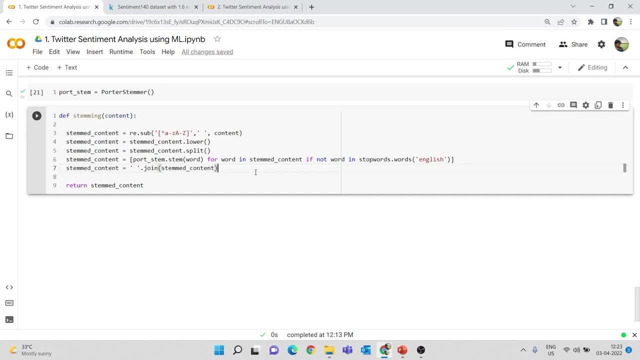 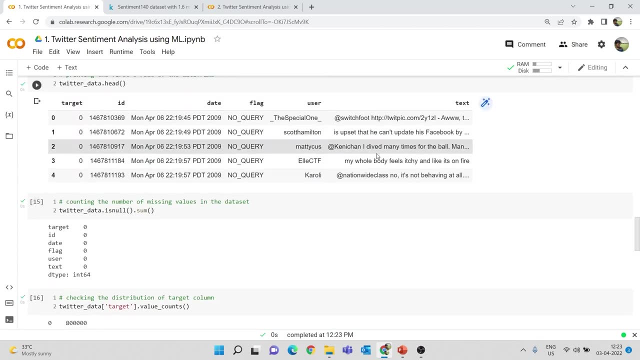 we call the stemming, okay, so I hope you understand this one. so this is the most important part of this code, so I'll run this function. now we have to- uh, you know, apply this function to the text data that we have. so this step is just, like you know, building the template for our stemming function. now we have 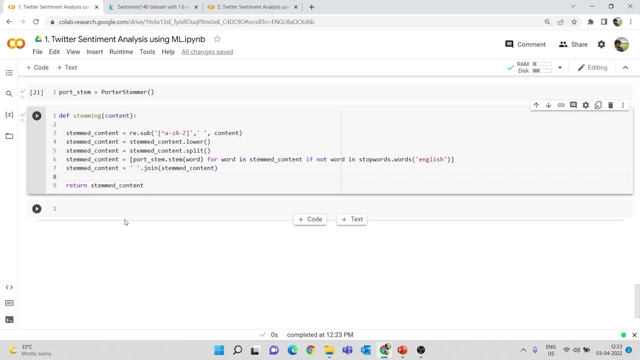 to apply this function to the data that we have. so I'm going to say Twitter data and within this I'm going to create another column. so if you want to create another column, you have to mention the data frame name. in this case it is Twitter data and within the square bracket. 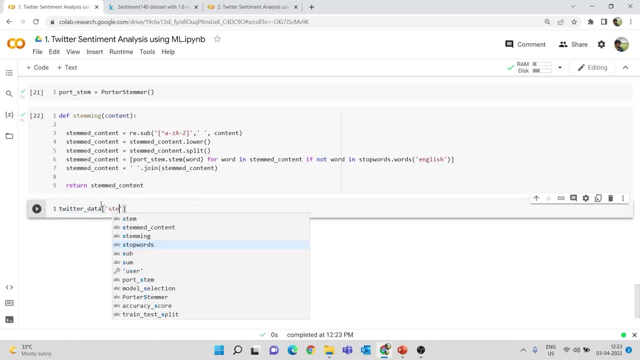 in the parenthesis, you have to name the column, so I'm going to name this as stemmed content- stemmed content. so this is the new column that I'm going to create. so the data to this new column is nothing but the stemmed content of the tweet. so Twitter data. 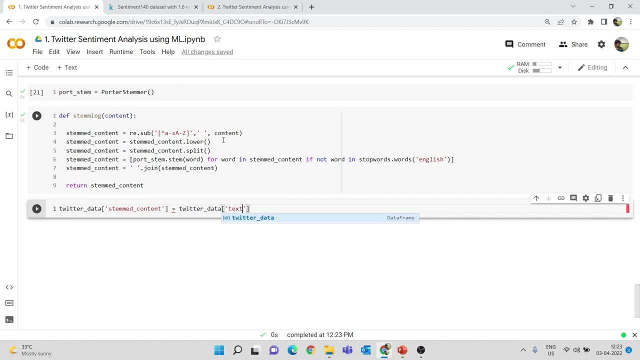 Twitter data of text. so text is nothing but the tweets that we have. I'm going to say: dot apply stemming, okay, okay, so this is the step. so we are calling this with Twitter data stemmed contents. I'm creating a new column and for this new column the data is stemmed content. so I'm taking this Twitter data. 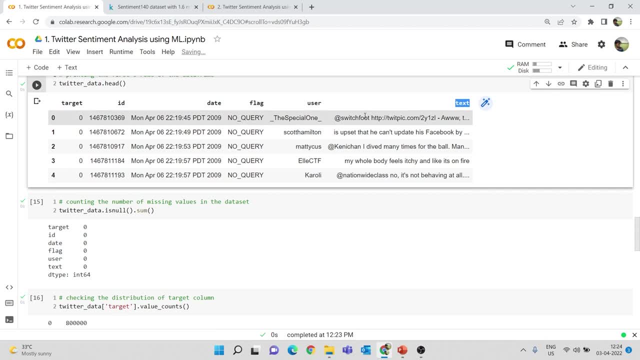 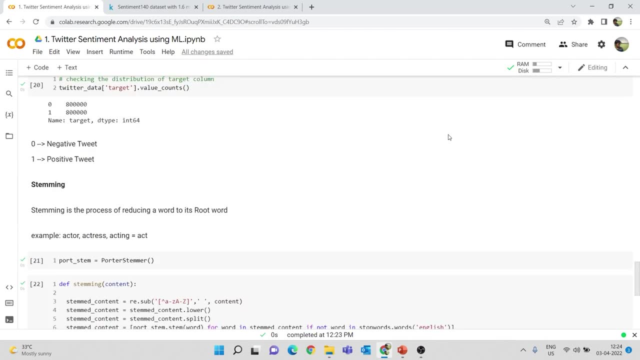 dot texture. so this is nothing but this column alone, text column alone which represent my tweet. so i'm taking this values alone, because we don't need any other uh details. okay, so i'm taking this text and here i am applying: right, so here it should be like: 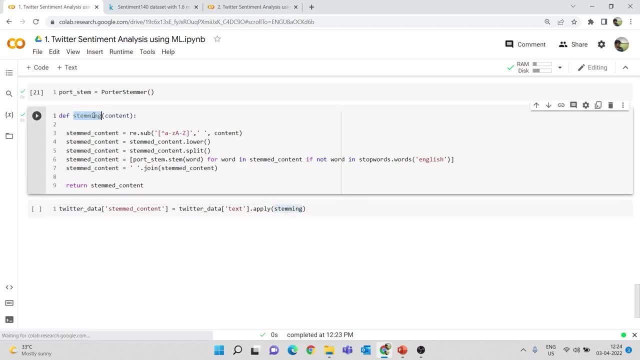 dot, i'm applying stemming. stemming is nothing but the function that we have created here, right? so that's what we are doing here. so when you run this one, all these operations that we have mentioned here will be performed on all the tweets that is present in our data frame. okay, 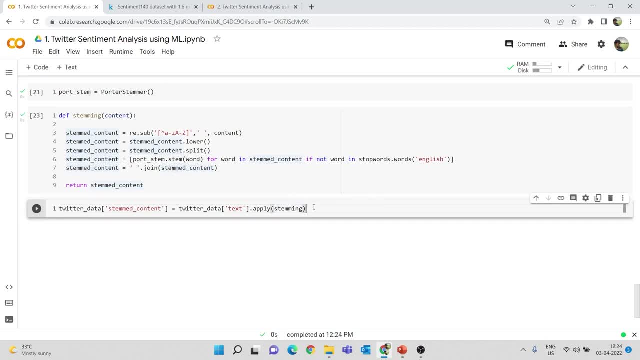 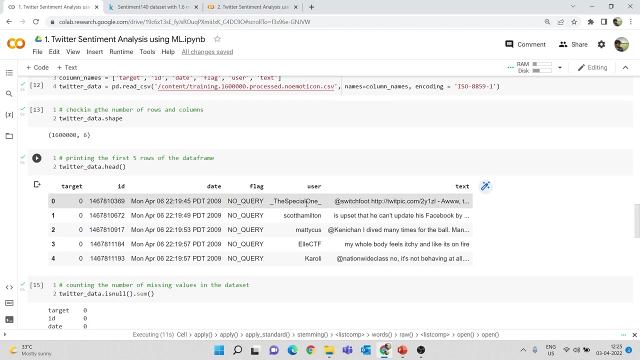 so we have successfully run this function and now we have to run this stemming operation. when you run this, this operation will be performed on each individual tweets. right? and here's the catch: this stemming operation will take a very huge time in order to complete, because the reason is, as we have like 1.6 million tweets, which is equal to like 16 lakh tweets, right? 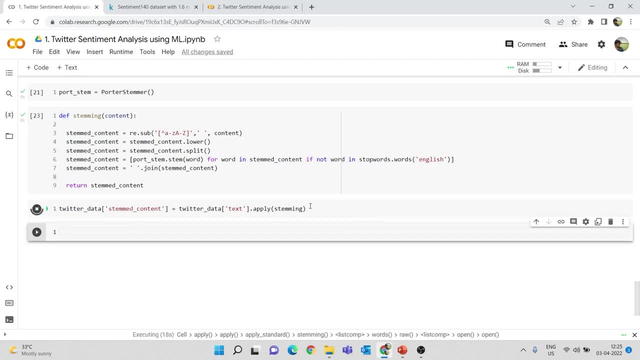 so it will take a very. you know it takes a lot of time and, uh, i checked that it took about like 15 minutes in order to complete this tweet. not 15, it took like 15 minutes for this. so i mentioned this 15 minutes to complete this execution. 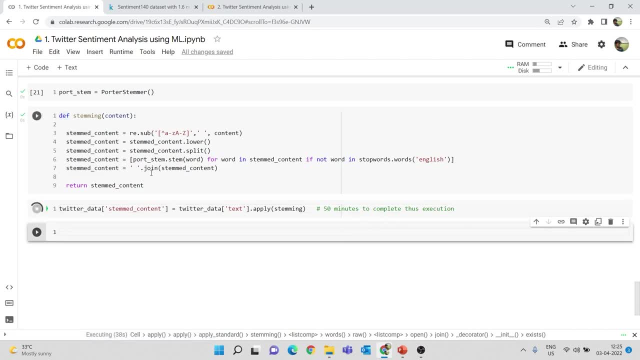 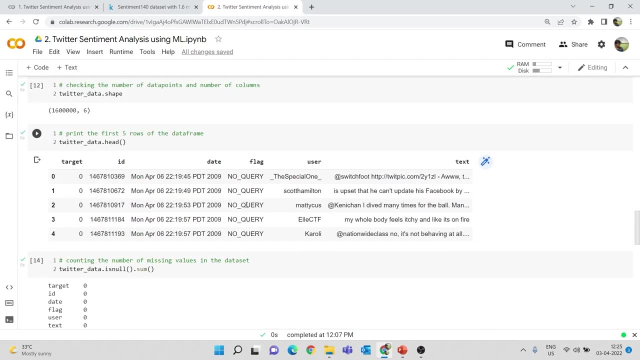 okay, so you have to wait for this. so you have to wait like 15 minutes in order to complete this step of stemming. so i've created another file where i have already started this stemming operation and this process has been completed. so all the other codes are basically the same thing. 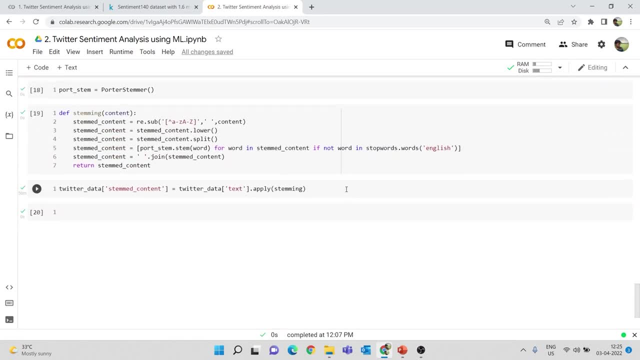 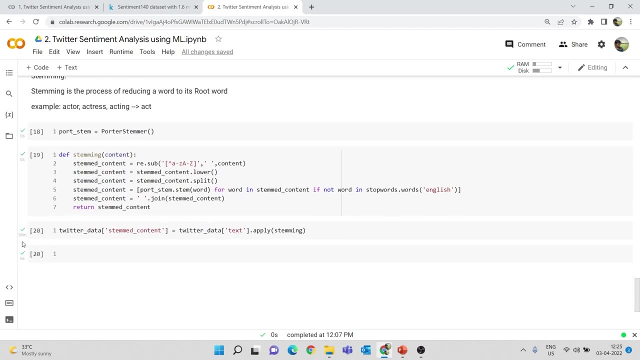 from pip install to kaggle, all the way up to this stemming. all the things are same, but it has been completed here you can see. so these cells took like zero seconds. so these cells like executed, whereas if you see this one, it is represented as 50m, which means like it took 50 minutes in order. 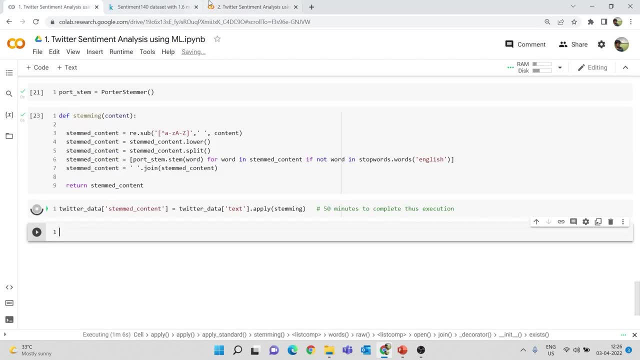 to complete this step. okay, so it will run for a long time. so i have created another file so we can quickly go through this. so if you are working on this on yourself, so you have to wait for 15, 50 minutes, so there is like no other options. now we can continue with our you know part. 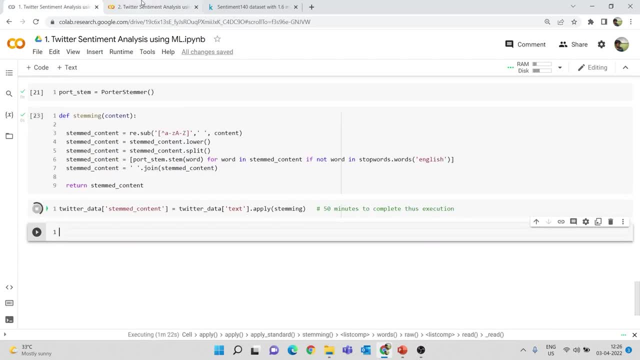 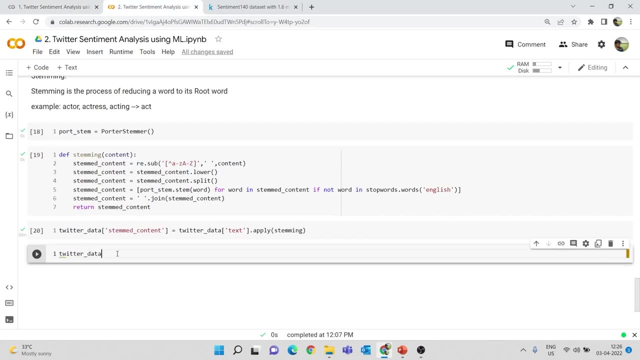 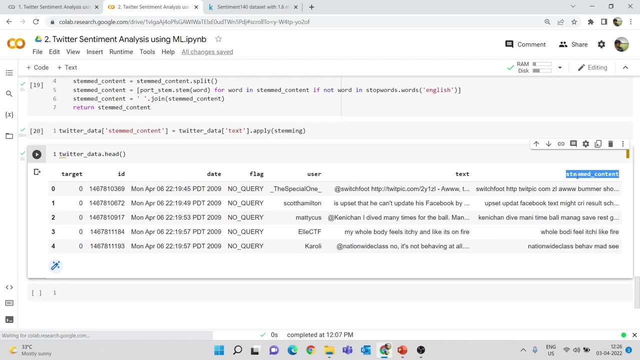 okay, so let that code runs. we are just continuing this code in this colab file, so there is like no change between this color file and this color file, so So I am going to print the first five rows of this data frame. So here you can see, we have another column called a stemmed content, whereas previously 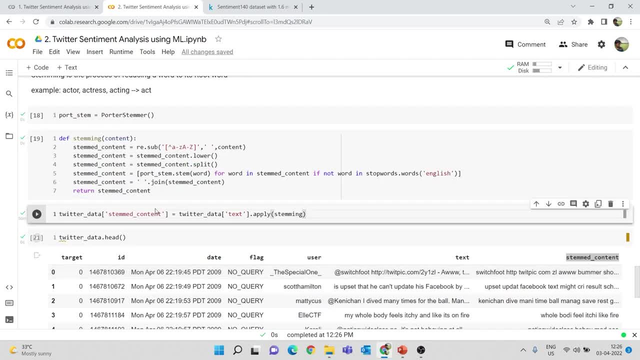 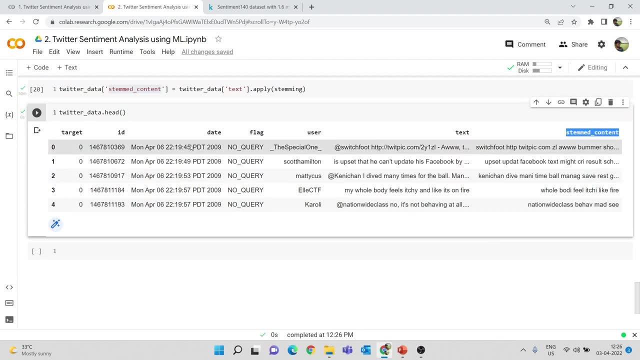 the stemmed content was not there, right? Because we are performing the stemming operation and storing the content to the stemmed content. So this is the final thing that we need. So we will be using the stemmed content and we will be using this target. So we will basically like ignore all the other columns because we do not need this. 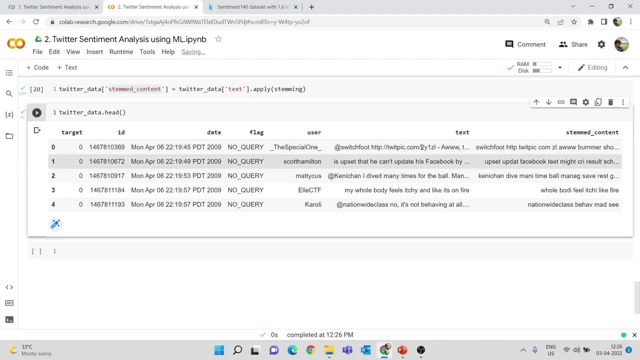 So we have, you know, this column has been made from this text, column right. So this is the raw data and this is the process data. So we will take this stemmed content and target for our, you know, training, our ML model. So this process is called a stemming, where we are doing all this processing of removing. 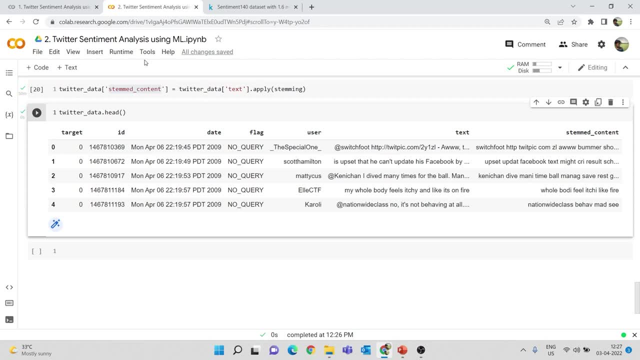 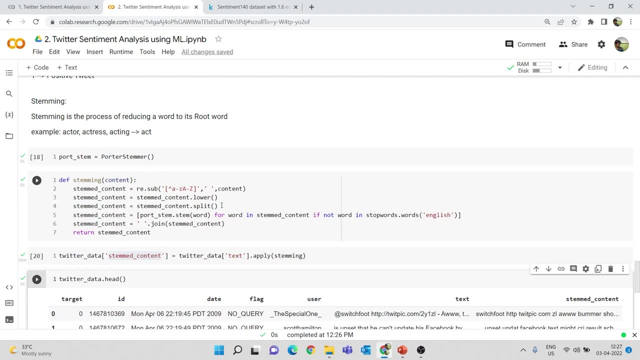 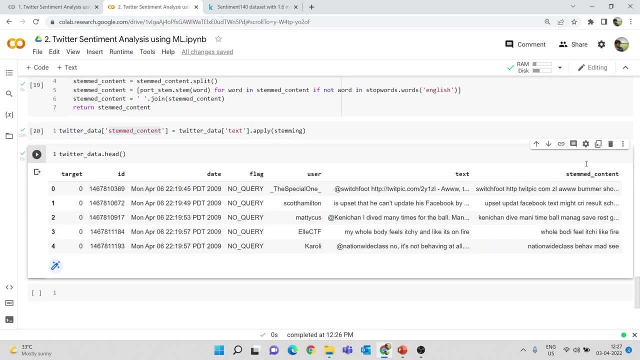 the stop words and removing the special characters, numbers and punctuations, and later converting the uppercase letters to lowercase letter, then splitting each word in a tweet to a list and then like performing the stemming operation and joining the words back together. So this is what we have done and we have like built this stemmed content column right and 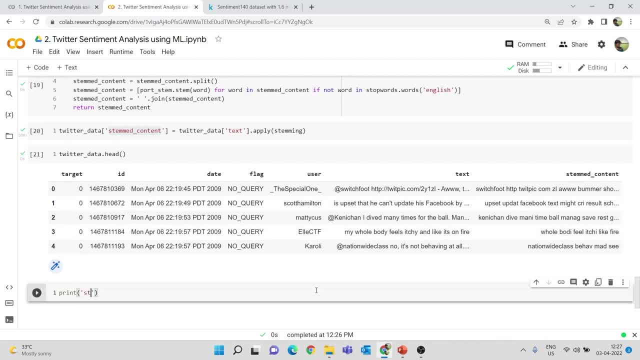 I can also print this column alone, So I can say print stemmed content. okay, so I have to say print twitter data. I have to mention the data of him, which is twitter data, stemmed content. So this is the tweet data that I am going to use. as you can see, there are like 16 million. 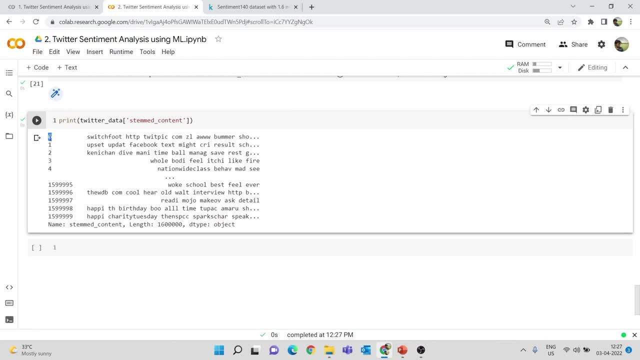 as I have told you before, the indexing starts from 0 in python. So 0, 1, 2, 3. so that is why we have like 1, less than 16, like 16 lakhs. So this is actually like 16 lakhs to each other, as the numbering starts from 0. this 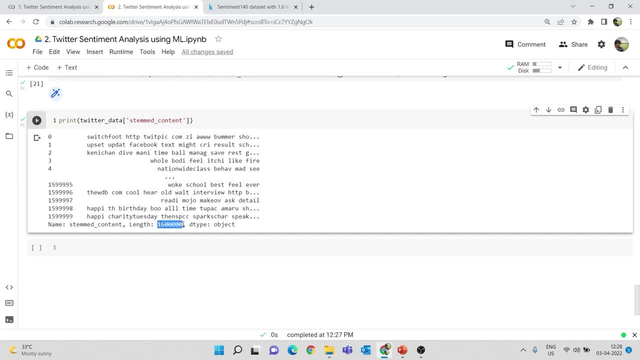 is the number we have, So you can see the length here, which is like 1.6 million or 16 lakhs. okay so, but the indexing starts from 0 and you know the 1 less than this 16 lakhs. so that is what we have here. 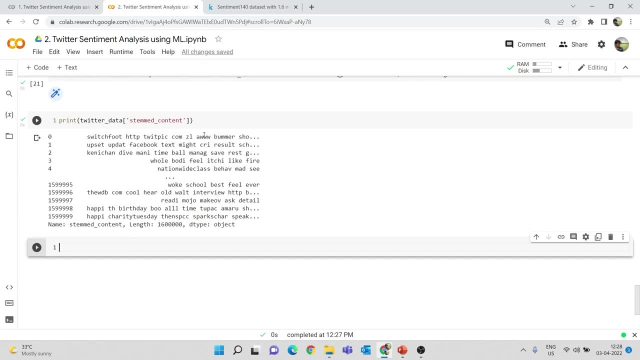 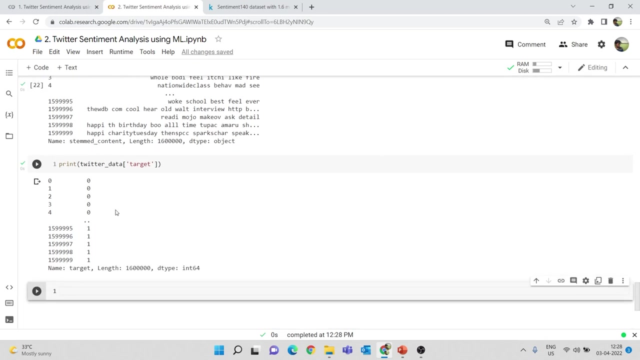 So this is the data that I want in order to train my ML model, and I will also print this target. Okay, instead of this template content, I will print target which contains the label either 0 or 1. okay, so 0 means negative tweet and 1 means positive tweet. 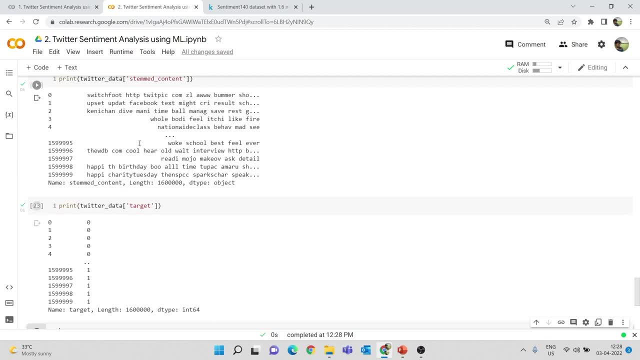 So these two things are the ones that we need. so we will pass this tweets and we will pass whether that tweet is a positive tweet or a negative tweet. Now the model will try to understand what is the relationship between this- positive tweets and 1 and negative tweets and 0. so it kind of understand if a particular word 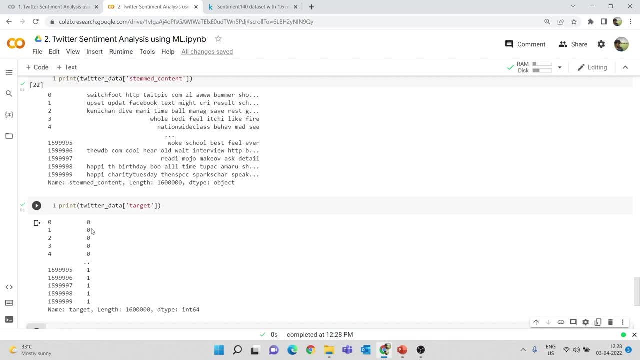 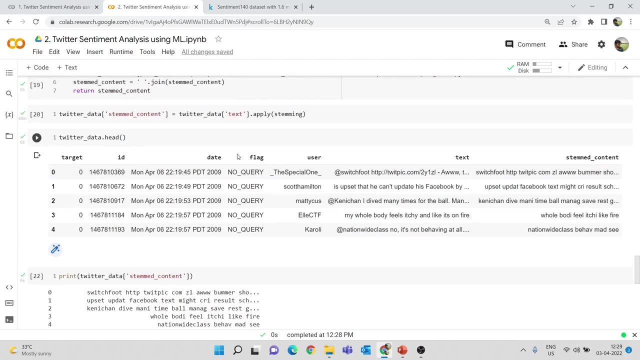 is there That it is a negative tweet. if a positive word is there, it will know that the intention is positive. So we want like these two things alone. we don't need this tweet of the id, date or flag in order to know whether it is a positive tweet or a negative tweet. so that's the reason. 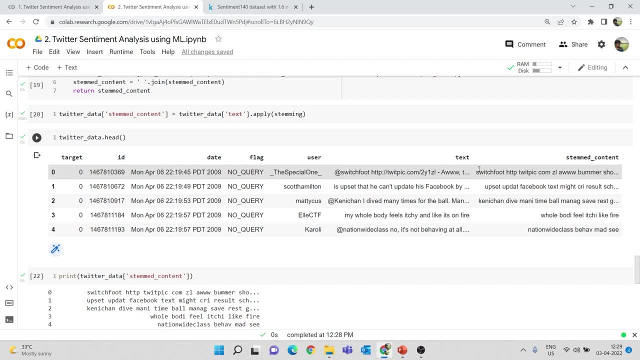 Say, for example, you don't need a person's username in order to understand whether they tweeted something positive or negative, or you don't need the date or time in order to understand whether a tweet is a positive or intention tweet, or it is a tweet with negative. 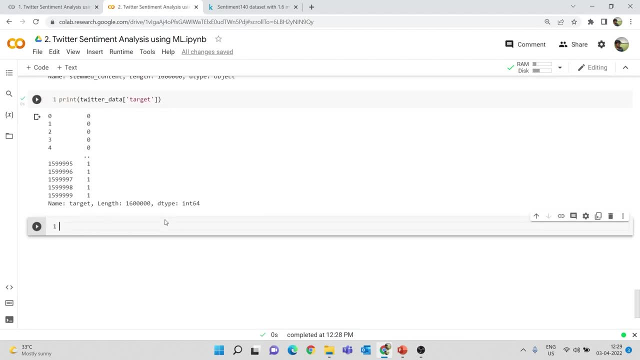 emotion. So that's the reason we don't need any other things except for this tweet and the data. So this part will be separating the data and label. so in this case, the data is the tweet and label is the target column- either 0 or 1.. 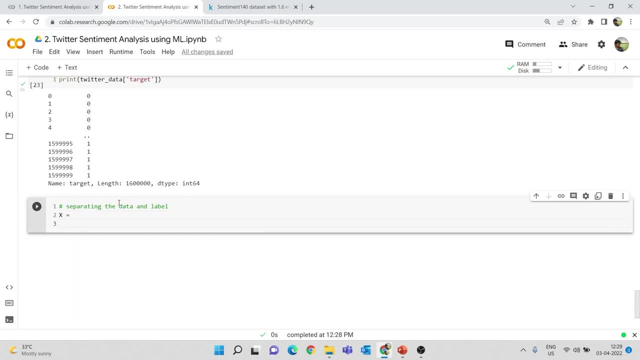 So I am going to create two variables: one is x and the another one is y. so in x, I am going to store all my tweets and in y, I am going to store all my target. I am going to say twitter data. Okay, so, as you can see, this cell is keeping, this keeps on running, so it will take as I. 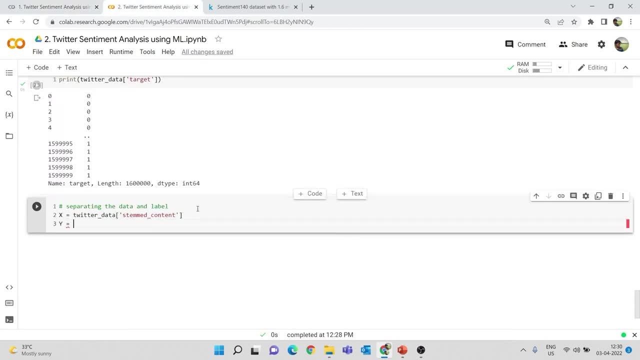 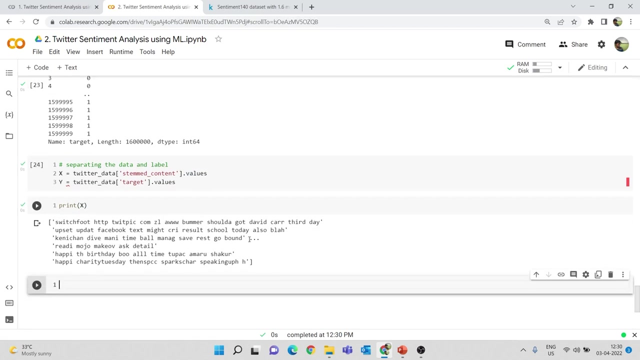 have told you 50 minutes to complete. we can continue with this one dot values, and for this I am going to say twitter data target dot values. okay, now I will print this six and y separately. so this is how you can split your data and labels. so this is my stemmed 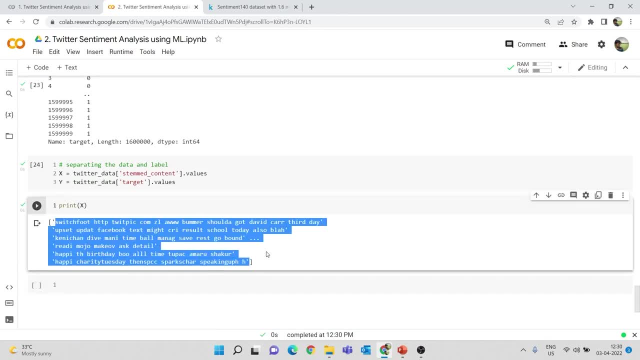 content. so this, this may seem low, but this actually contains like one point six million tweets. so like we are just seeing this like shortened ways, so like the first few tweets and the last few tweets, so that's why this is like looking like this: so this is the stemmed 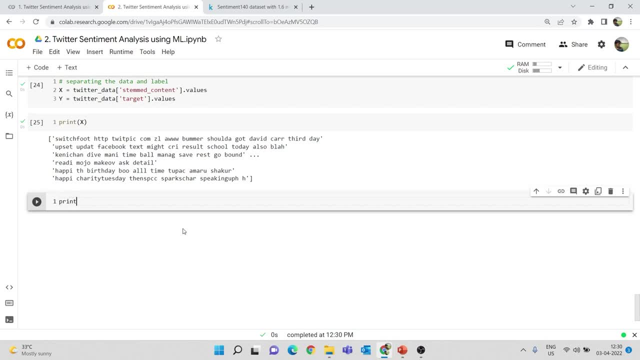 content that we have, and then you can also print this Y: Okay, So are seeing the first three target and the last three targets. Okay, so again there are, like totally you know, 1.6 million data points are there And the next thing that 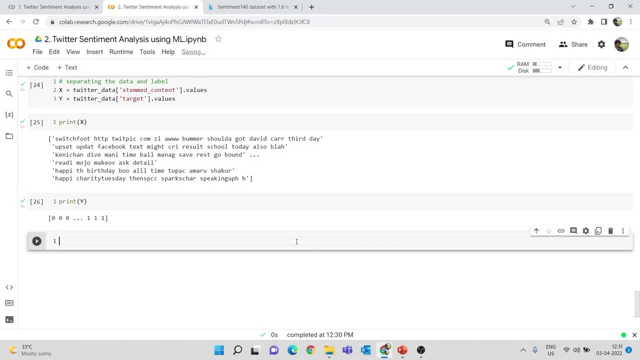 I have to do is split this data into training data and test data. As I told you, once we have a data set, we have to split this data set, and training data is used to train my model and test data is used to evaluate my model. right, So this part will be then put. 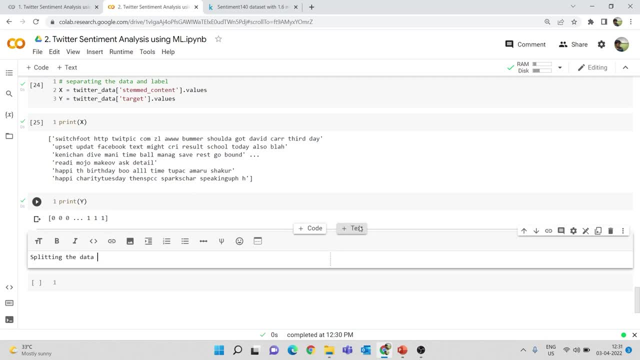 a text here as setting the data to training data and test data. Okay, For this we have to create four arrays: X train, X test, Y train and Y test. So these are the four arrays that we are creating And I'm going to use the train test split function, Train test. 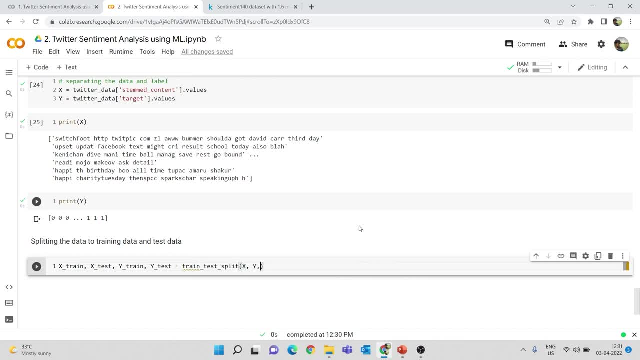 split, And within this we have to say X, comma, Y and test. the size is equal to 0.2 and stratify is equal to Y And finally, random state. I'll explain you what all these attributes mean. just wait for a moment. So random state is equal to two. So let's try to understand this. 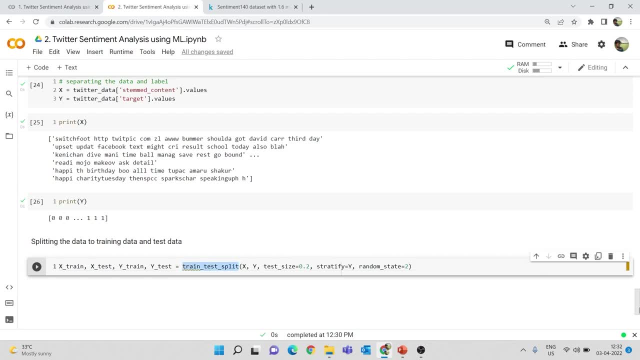 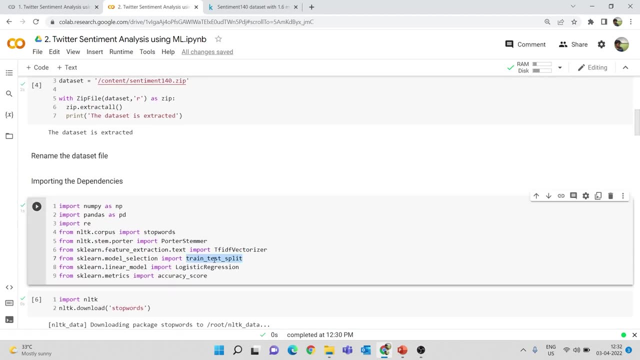 I'm using this train test split function, So we have already imported the test split function from here, as you can see. So this train split function function is used to split the data to training data and test data, right, And I'm creating like four arrays. 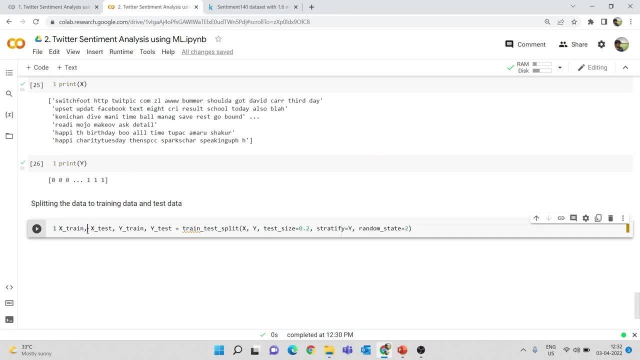 The first array is X train, X test, Y train and Y test. So X train will contain all my training data tweets. Okay, So this X train is split from this X. It will contain all the training data tweets and the corresponding label. this corresponding target are stored. 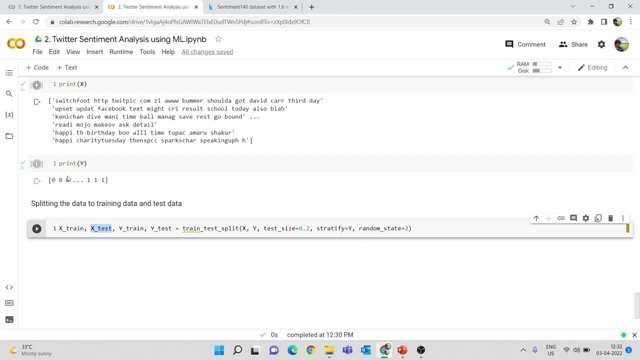 in this Y train And the X test contain my test data tweets and Y test contain my training data. So this X and Y test will be linked And I can say X train is going to contain whether it is a positive or negative for all the six tests. Okay, So this X train, Y train, 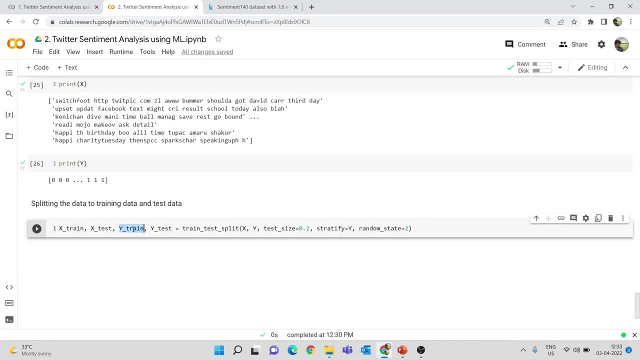 are linked. This X test and Y test are linked. Okay, So this is my tweet for training data. This is the target, the label for my training data. this is the test data tweet and this is the label for this data. Okay, And then we are doing this brain test split function. 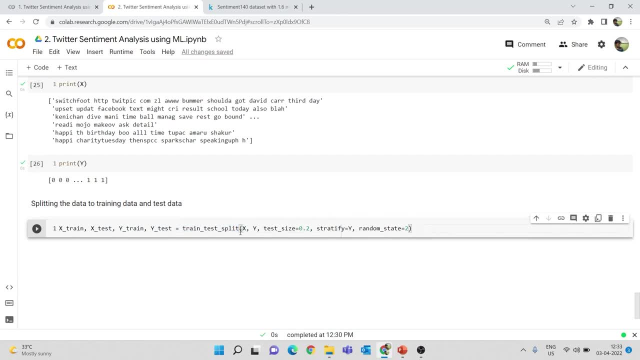 And we are splitting with this X and Y. so X is my tweet and Y is my label. So we have to mention X comma Y. And what is your tester size? Tester size means like how many data points you need test data point. so 0.2 means 20 percentage of my data will go to my test data and 80 percentage of 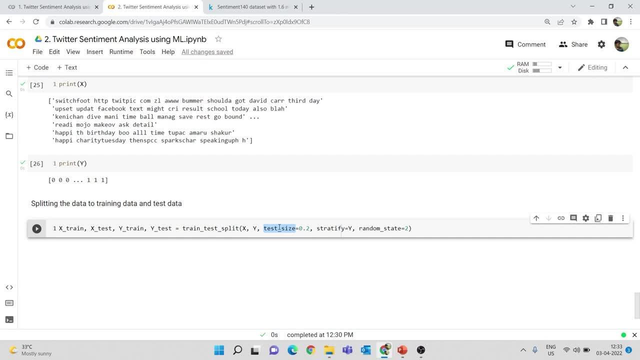 data will go to my training data, right? so out of 1.6 million, 80 percentage of this will be my training data and 20 percentage of 1.6 million will go to my x test data. so this is the general proportion that we use. you can, you know, consider either 20 percentage of the data as test data or 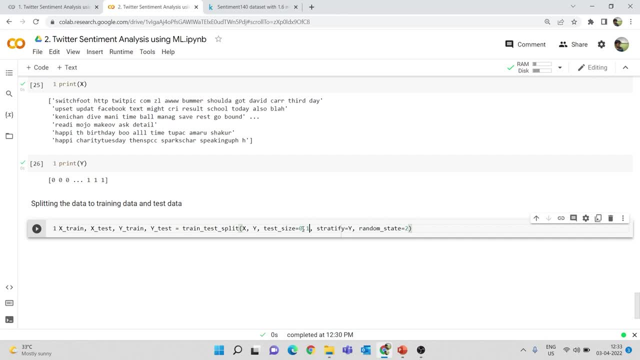 10 percentage of the data as test data. if you mention 0.1, that means like you want 10 percentage of data as your test data. okay, so i will just put this as 0.2 alone, and stratify is equal to y. so 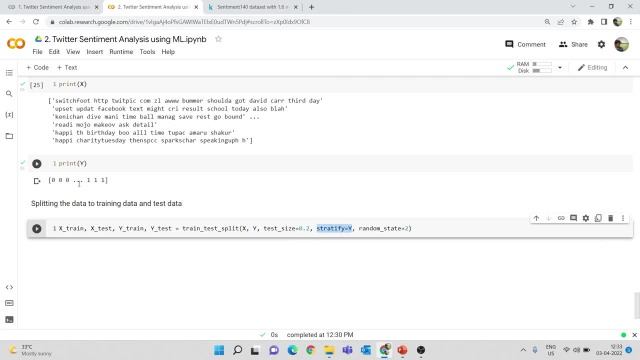 what this stratify means is: i want an almost an equal distribution of 0 and 1. so this is this means, like in the training data, if the proportion of uh positive and the negative to it is like 50 percent of each, it would be the same in test data as well. so if we do not do that, there is a chance. 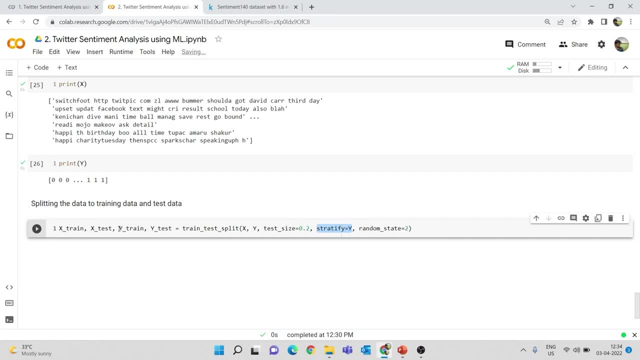 that all the- uh, you know, negative tweet may go to this test data instead of this training data. so we need to stratify: is equal to y in order to tell this train test rate down to this point, and then that I want equal proportion of the two classes, which are 0 and 1, both in my training data. 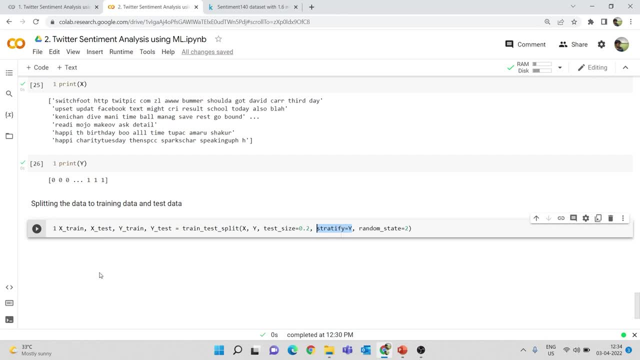 as well as test data. So that is the purpose. and finally, we have this random state, so if you run this train test without this random state, you can also run this without this random state. if you do that, each time you split your data, your data will be splitted. you know differently. 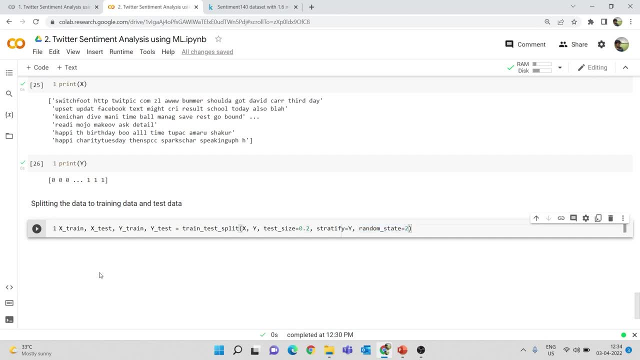 so it will be a random split. If you mention this random state is equal to 2, it will the you know, splitting will be replicated. let us say, for example, I am using this random state is equal to 2. let us say that you are practicing this code and instead of 2 you are using a value as 5. so your data. 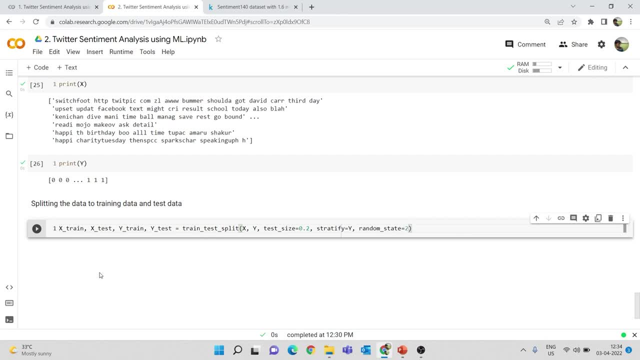 will be splitted differently and my data will be splitted separately. So if I use this random state is equal to 2, and let us say you are also using this random state is equal to 2, in that case your data and my data will be splitted in the same way. 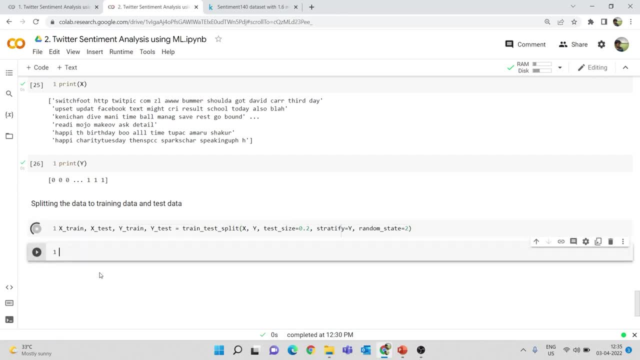 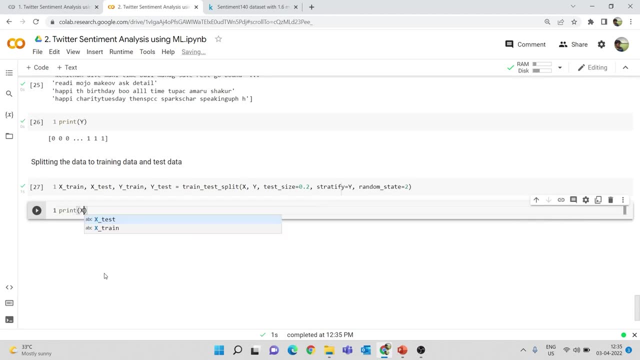 so that is the reason for this, using this random state. okay, And you can also Also print the x train. so let us print this: x dot shape, x train dot shape and x test dot shape. okay, so, as we can see, there are like 1.6 million data, so this is my original data. 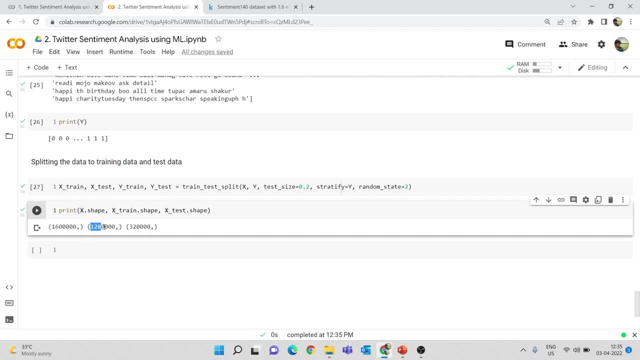 set. So 80 percentage of this 1.6 million is this, which is I think 1.2 million, okay, And the remaining data goes to my. so this is like 20 percentage of 1.6 million. go to my x test. 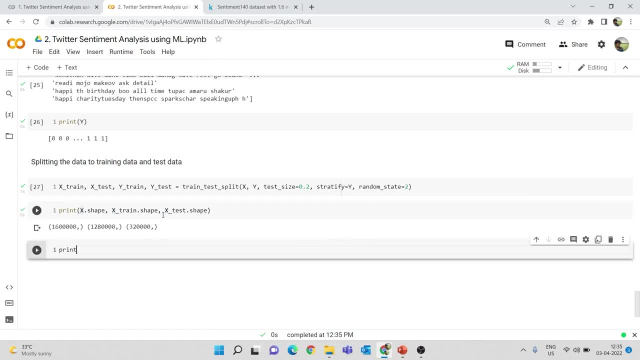 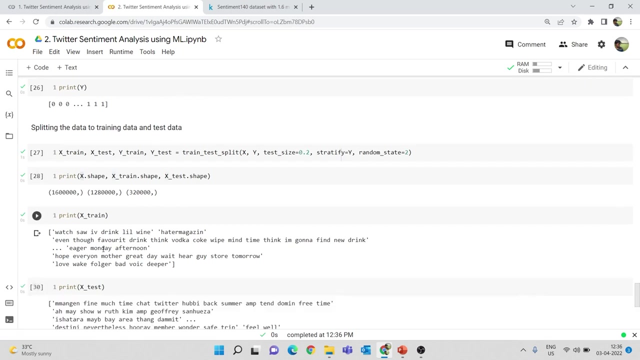 So this is how this train test split works. okay, so you can also try printing this x train and x test. So this is my x train, then print my x test. okay, so this is my training data, which contain like these many data points, and this is my test data, which contain these many data points. 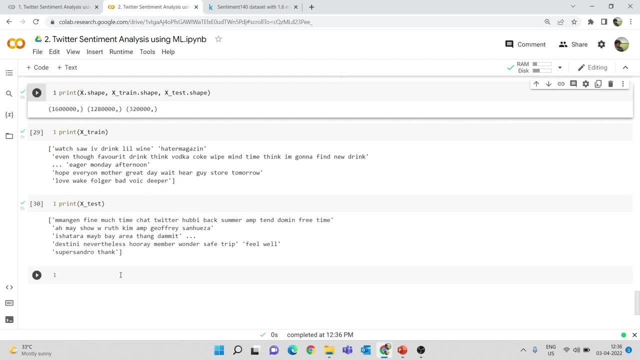 and now. So this is another important thing- that we have to do, so before training our ML model. as I have told you, ML model does not understand text right, so we have to convert this text into numerical values. so this is where we will use a process called as feature extraction. 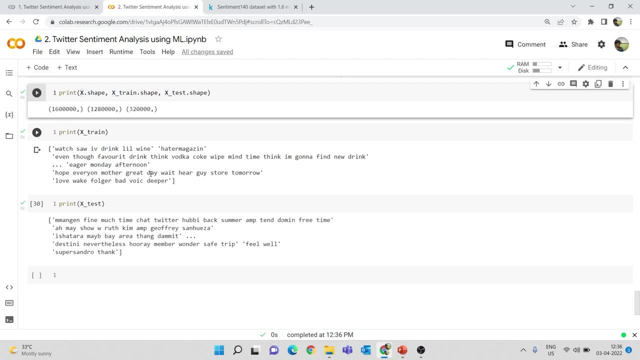 where we are going to extract the feature from this text, or you know, we are going to use a method called as vectorizer. okay, so this part of the code will be converting the textual data to numerical data. okay, and I am going to create a variable called as vectorizer. 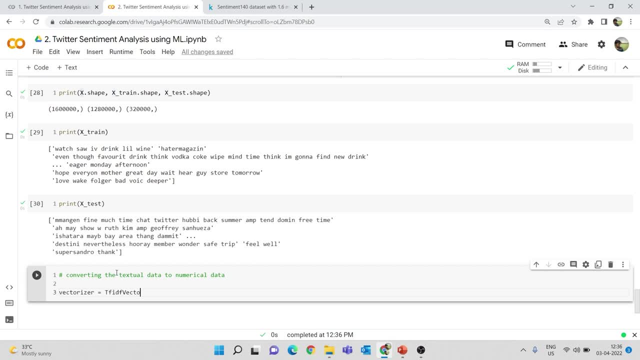 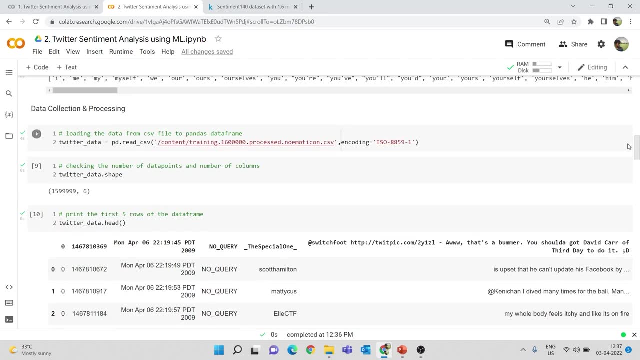 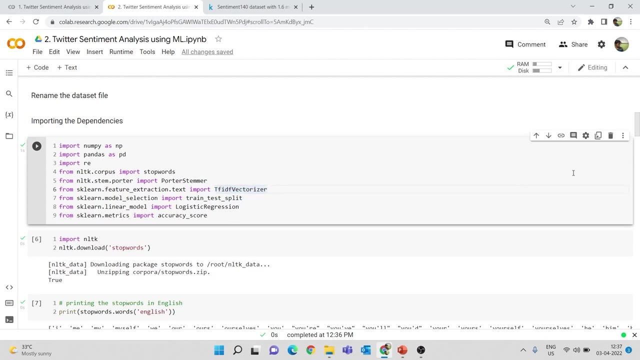 which is equal to tf idf vectorizer. okay, I have to mention parenthesis. if you remember, we have imported this tf idf vectorizer while importing the dependencies, so this one. so from your scale run dot feature extraction, dot text: I am importing my tf idf vectorizer. 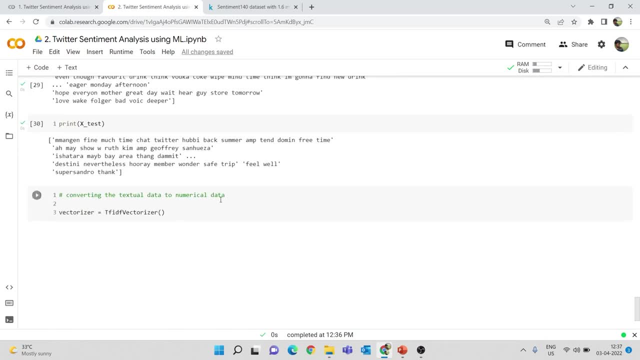 So this was so. this one will convert my textual value into numerical values so that my ML model can understand what is present in this particular data set. I am going to say: x train is equal to vectorizer dot fit. transform of x train and x test is equal to vectorizer dot fit. 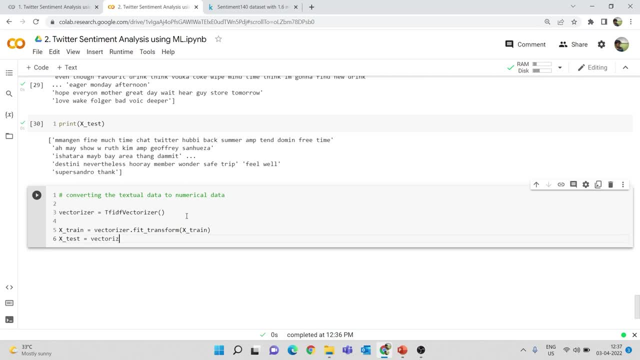 transform. So let us try to understand what we are doing here. so this function, as I told you, will convert all the words into some numerical values, and it is important that we have to understand how this works. so this vectorizer function will consider, like each word, and it will give: 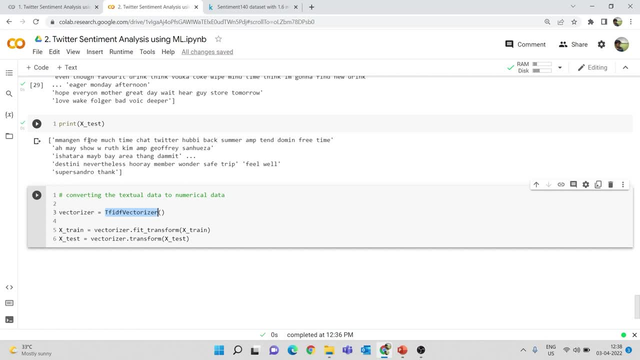 some importance to each word. so like there is some like, let us say that there is this word called as fine. So it will check how many times this fine has been repeated in my overall tweet. so in my overall data how many times fine has been repeated, so you know, so that, like this fine. 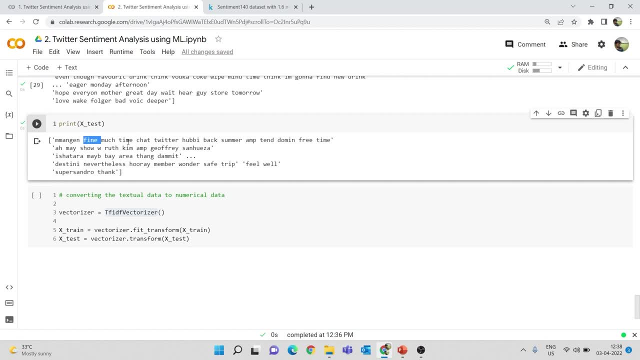 will get some, some importance. and there is like another word called as time and then chat. so based on that repetition it kind of get some, get some importance value. so we are like encoding all the textual data to some numerical values which kind of tells us importance, right? 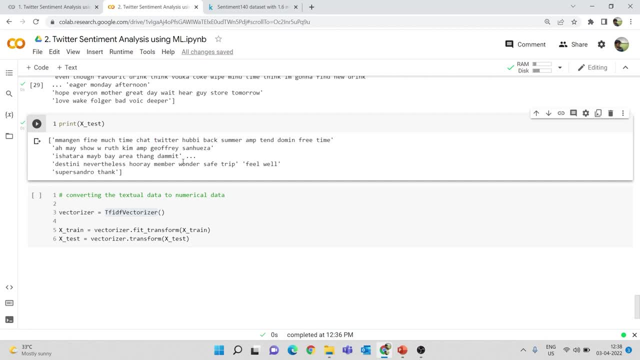 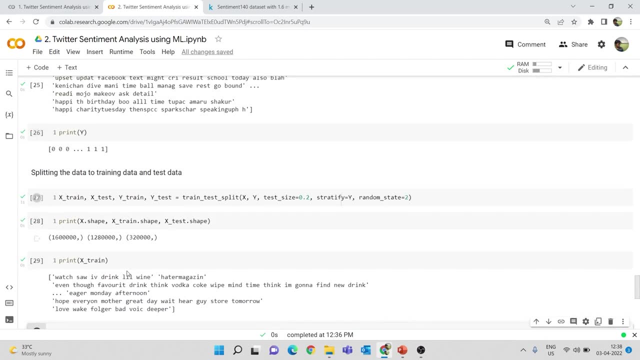 So we have one specific value, so each word will have one specific value. so once we do that, our machine learning model will try to correspond that numerical value, which is the importance value, to either 0 or 1.. So let us say that there is a world called as fine, or let us say that there is a world 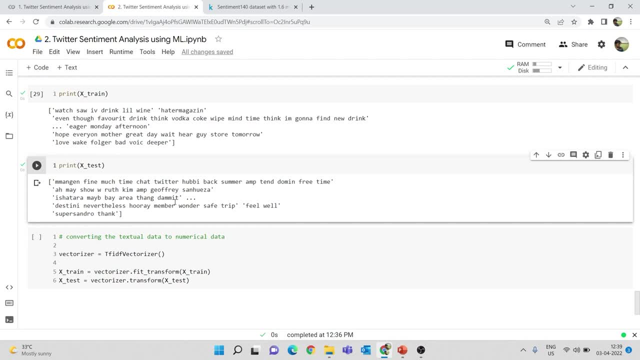 called as happy. so those are like positive words, right? so these words will get an importance score based on how many times these words has been repeated. so let us say that this happy word has been repeated for positive tweets, and let us say that no negative tweets as the. 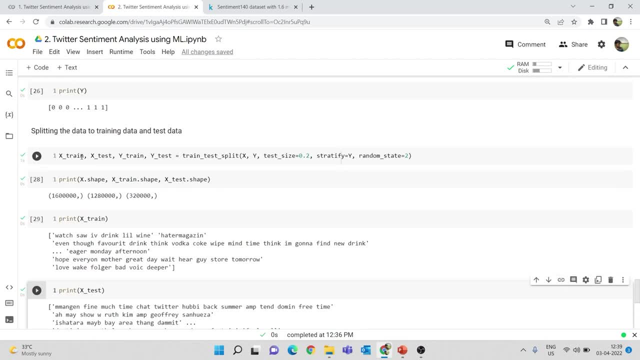 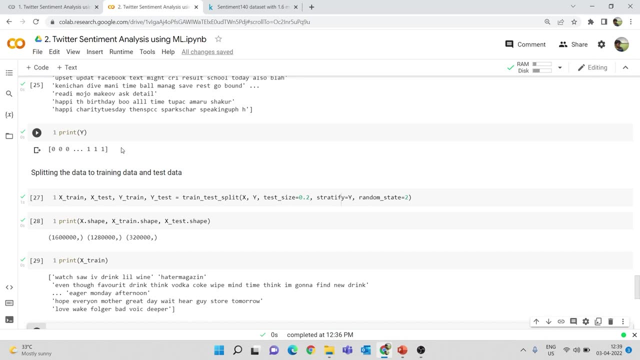 the you know text happy, in that case the model can understand that. okay, if a word happy is present, then in that case it is a positive tweet. if a word like you know, sad, or words like the present, we can say that it is negative between- i'm just giving you one example, but the ml model will like consider 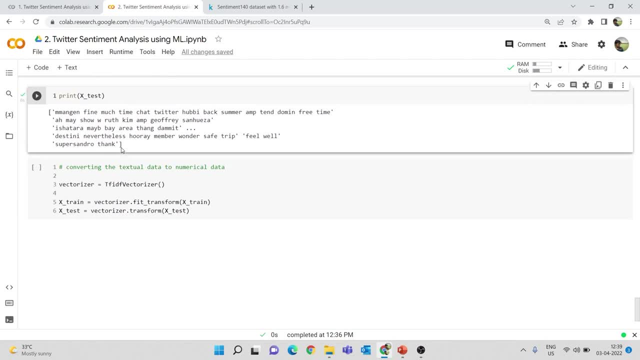 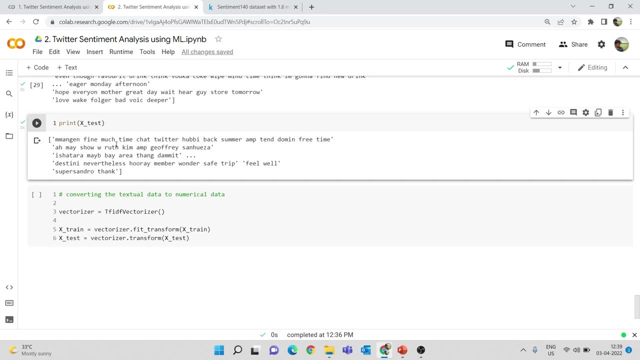 a lot of different words in a particular tweet, so we will take all the words in a in a tweet, so all the words has been converted to some importance, value and after that the ml model will try to understand what is very important and it will check whether, uh, it is a pos it that particular. 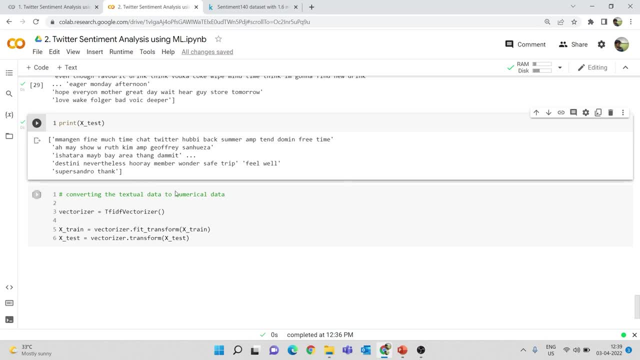 word corresponds to positive tweet or a negative tweet. so this is the process of this tf idf vectorizer, which is just to assign some importance to uh, each individual word. okay, so i'm like loading an instance of this tf idf vectorizer function to this vectorizer and i'm transforming 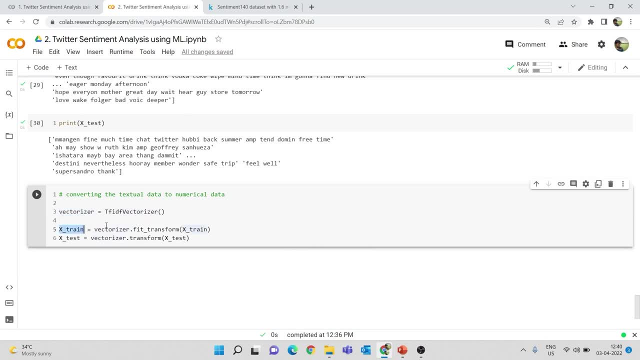 my training data and test data here. okay, so i have this x train and i'm using this vectorizer. so this vectorizer is nothing but this variable vectorizer i'm fitting and transforming. so i'm fitting my vectorizer to my training data and transforming this. so the result of this line of code, this fifth- 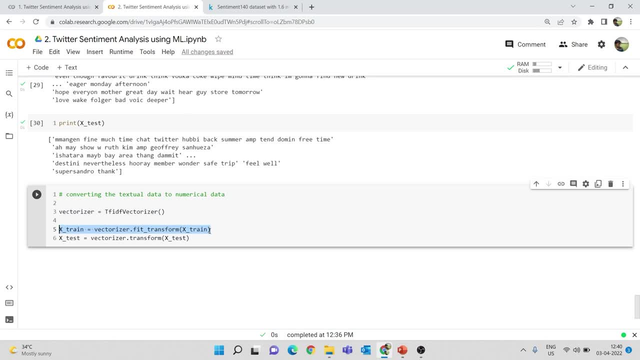 line of code is that all the training data will be taken and, based on this data, the uh vectorizing vectorizer will give uh score to all the individual words. okay, so there will be a particular transformation and, based on this transformation, we have to transform the test data as well, because 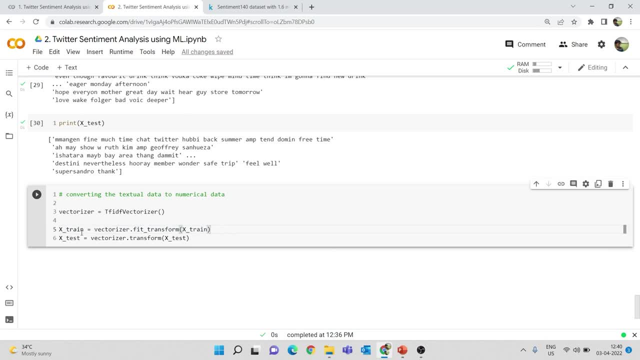 like you cannot have- you know words in training data, numbers in test data, so the data type should be the same. so we are transforming all the training data based on this transformation. we have to, you know, do this transformation in the test data as well. so, as you can see, i'm fitting. 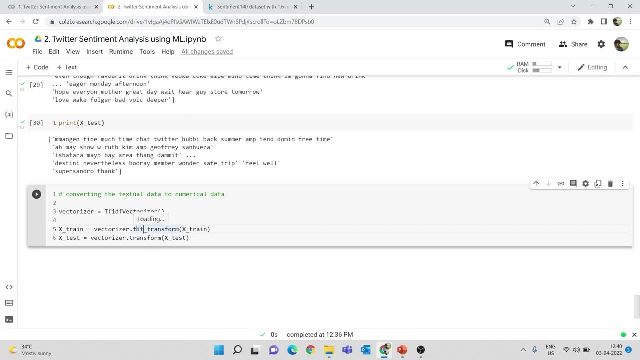 and transforming the extreme here. so there are like two process happening. so one is like fitting the vectorizer, for fitting means it tries to understand what is the nature of the data that is present here, and transforming is converting the data to this textual data to numerical values. 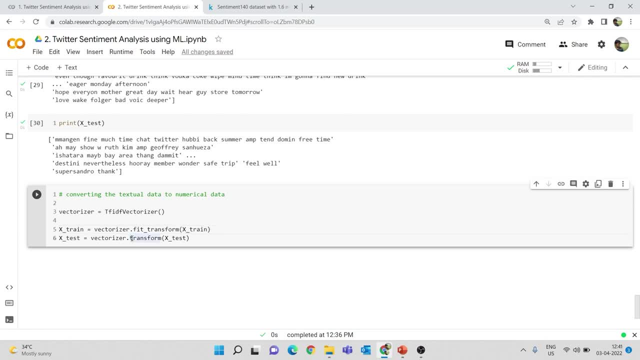 so in this x test i'm using this transform alone, so you shouldn't use like this, fit underscore transform. so it is a wrong procedure. you have to fit and transform only this training data, and the test data has to be transformed based on how this training data has been transformed. so this is very important, so you 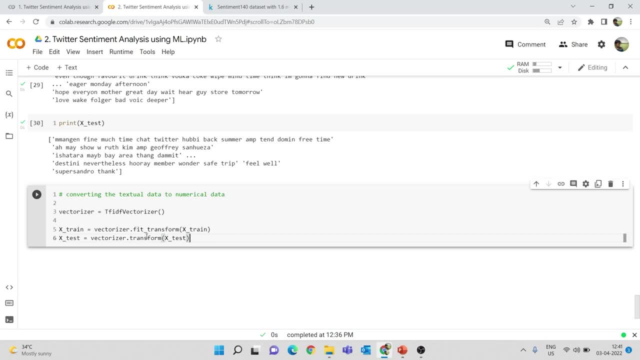 have to use fit underscore. transform this for this training data alone and only transform for this test data, right, so i'll run this one. so this will do all those processing. so let's wait for this to complete, and now i'll print my extreme and x test, my strain. 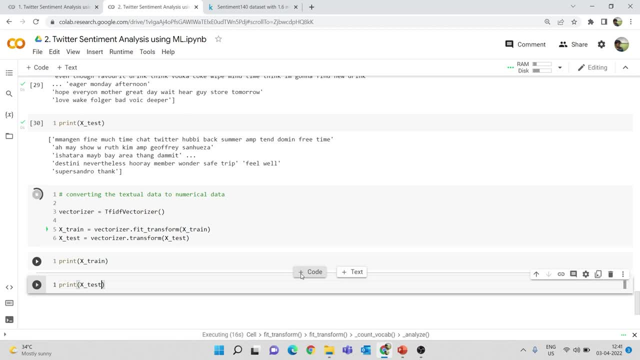 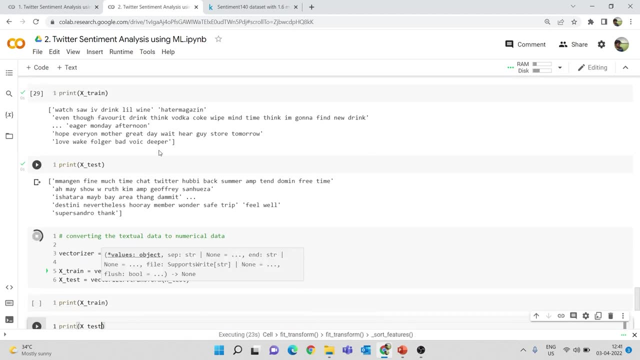 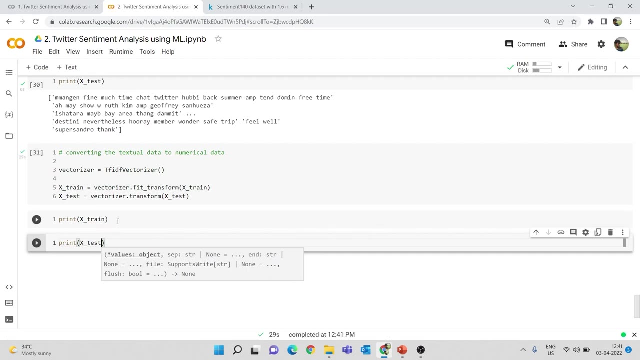 next test. so this may also take some time, but it won't take that much time. okay, so previously we have printed this extreme and x test right, so previously it is in the terms of words, and when i print this after this vectorizer it will convert all those values. 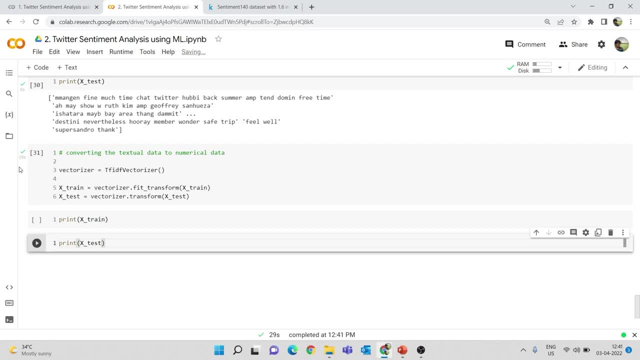 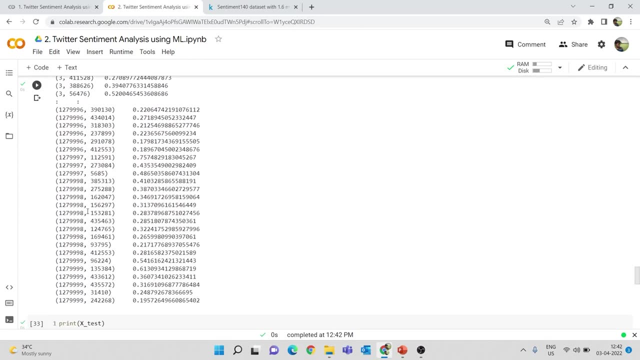 to numerical values. okay, so this is completed. so this took like 29 seconds. okay, now i'll print my extreme and x test. so this is how my- you know- extreme is kind of looking like and x test is looking like. previously it looked like this, which as words: so this is how victorizer will. 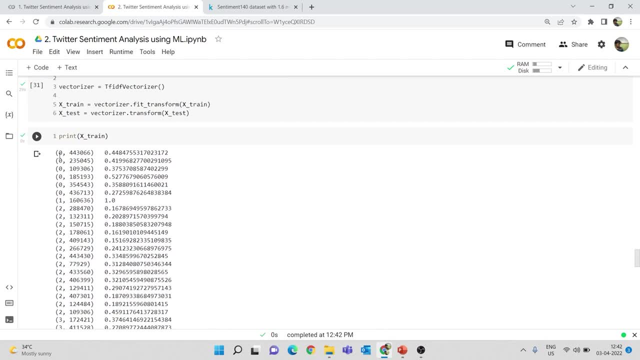 convert this numeric, this textual value, into numerical values. so zero means: uh, these are the like words in the first tweet, so those are mentioned like zero, these are like the words in the second tweet, and so on. so this is how like this works. okay, so all the words in all the tweets. 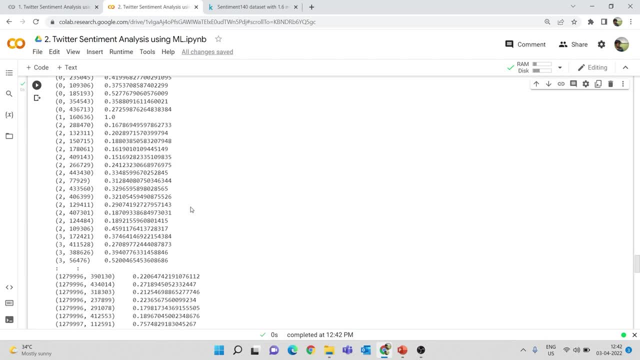 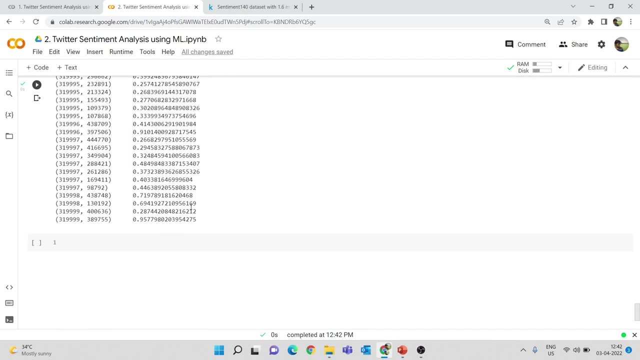 get some important value based on its repetition on, uh, that particular data set. okay, so this is how we can do this conversion, and all the processing are done, so we just have only one more thing, which is to train our machine learning model. okay, so all the data pre-processing and train test split has been completed, so this part is. 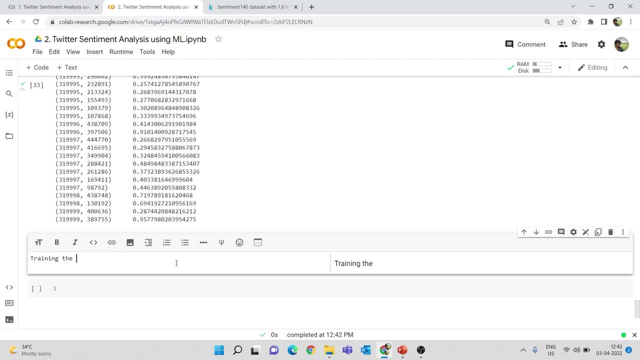 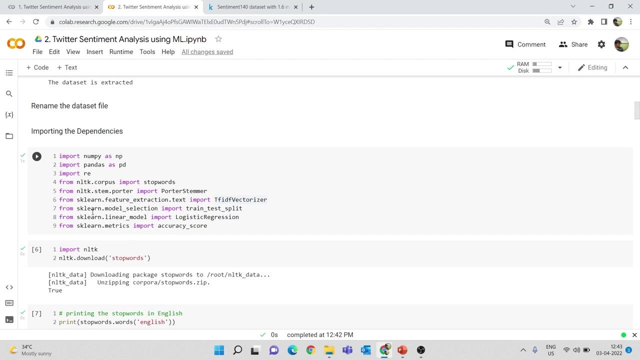 training the logistic regression model. so let me put this as training the machine learning model. machine learning model and the machine learning model that we are going to train in this case is logistic regression. okay, so we have already imported this logistic regression from sk learn dot linear model, as you can see. yeah, so sk learn dot linear models. i'm going to train this logistic. 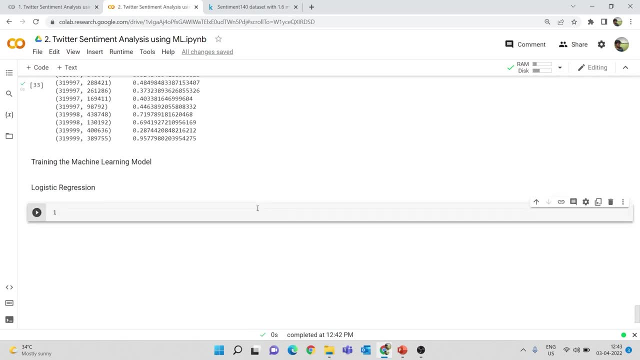 regression. again, logistic regression is a classification model. you can use it to classify the data points into different classes. in this case, the two classes that we have are positive tweet or negative tweet. right, i'm going to create a variable for this model, so model is equal to. 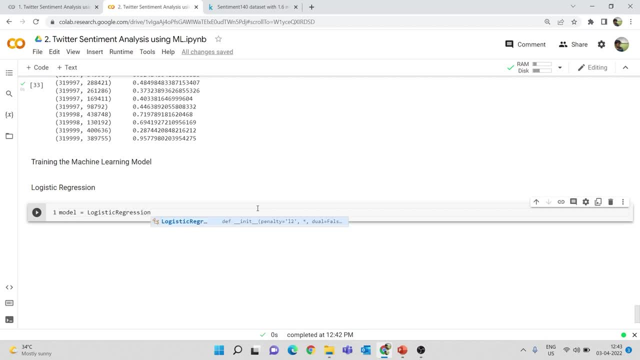 logistic regression. okay, i'm going to say max heater, so i'm specifying the maximum iteration, so the maximum number of times, the date the model has to go through the data. okay, so like it is not like only one step, so the model will go through the data again and again till it reaches a good 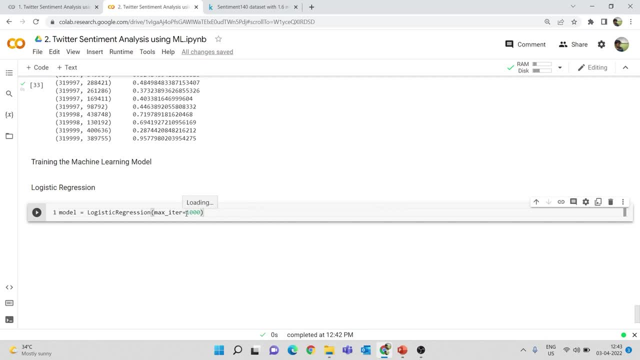 accuracy and this is the maximum number of times. maximum inter means maximum iterations, which means maximum number of times the model can go through the data. okay, so i'm loading this logistic regression to this instance, to this model, but i'm going to say model dot fit, model dot fit x train. 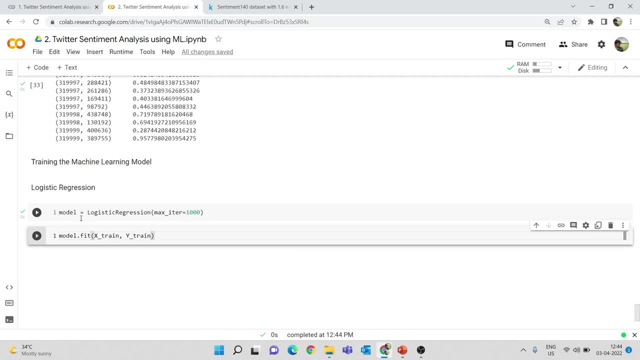 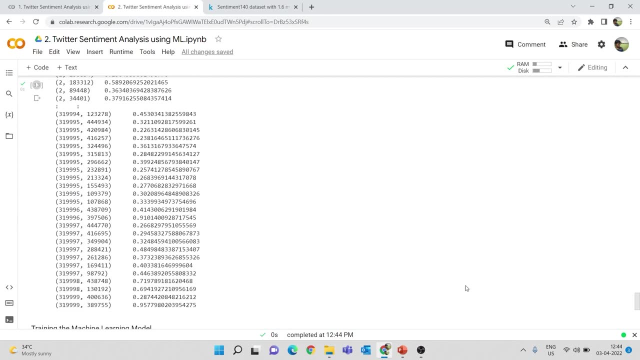 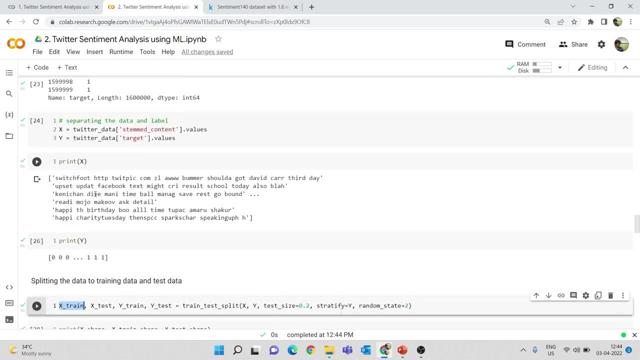 and okay. so y train is nothing but my training data tweet tweets, and y train is the target for this training data tweets. okay so, which we have seen on previously itself. so x train is my training data tweets from this. so this x will be splitted into two groups. one is training data. 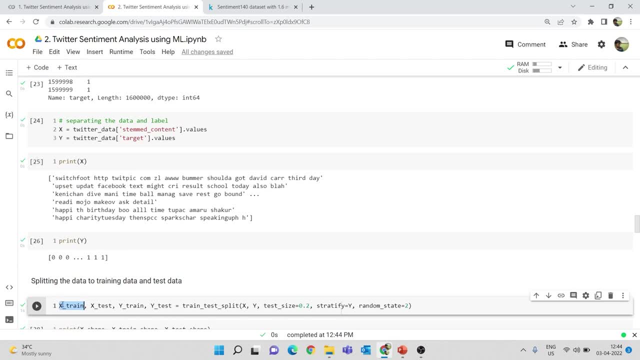 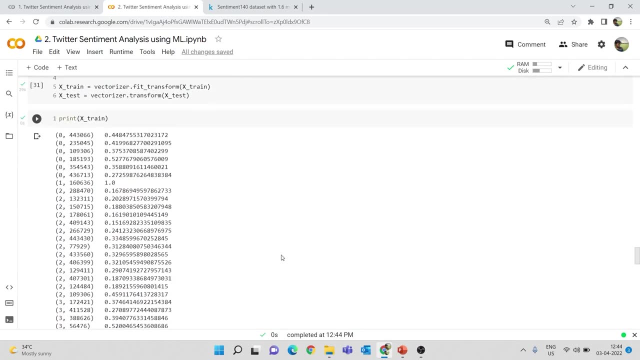 which is 80 percentage of the data and 20 percent test data. so this training data, the corresponding labels, are stored in this y train. so we have to feed this x train and y train to our machine learning model. so that's why i'm mentioning uh model dot fit. so this is the training data. 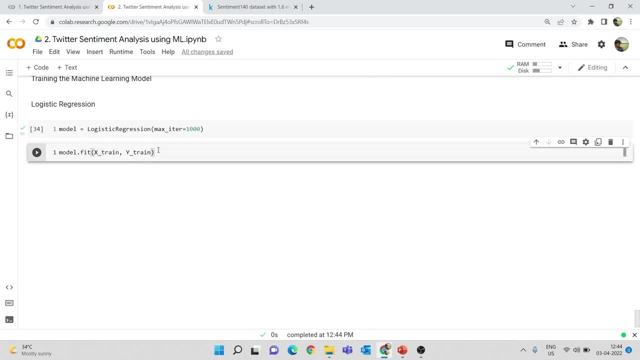 where the model will learn from the data. okay, so x train, comma, y train. so i will run this one. so this will also take uh some amount of time to train uh using this data because, like there are like almost 1.2 million data are there, which is like 80 percentage of the data. so in this, what happens in? 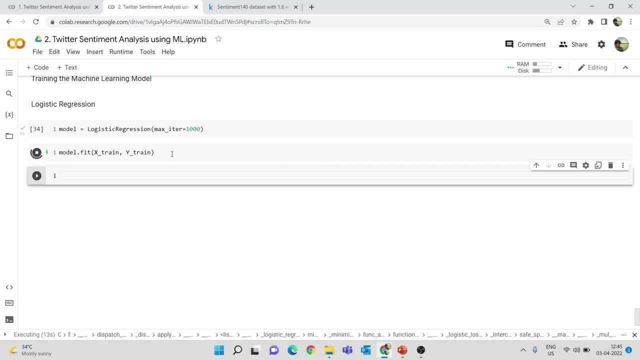 this is so the model will try to understand what are all the words that contributes to positive tweets and what are all the words that contributes to negative tweets. so i'm just telling this simply, but there are like a lot of complex procedures that is happening there, so it will try to kind of map, uh, the positive tweets to the label one and map the negative. 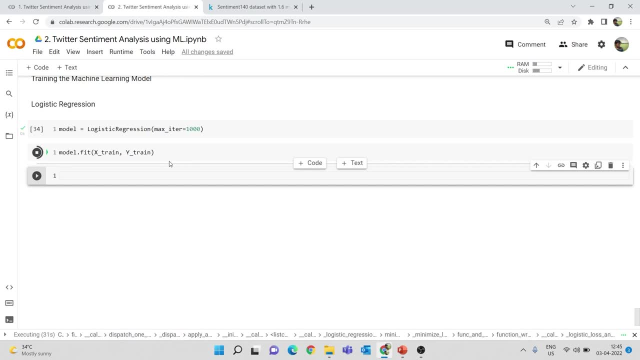 tweets to the label zero, so it will kind of try to find what is the relationship between this x and y. so that is what is happening here. so, once this training process is completed, we can evaluate our model in order to determine what is its accuracy. okay, let it run. let's complete the 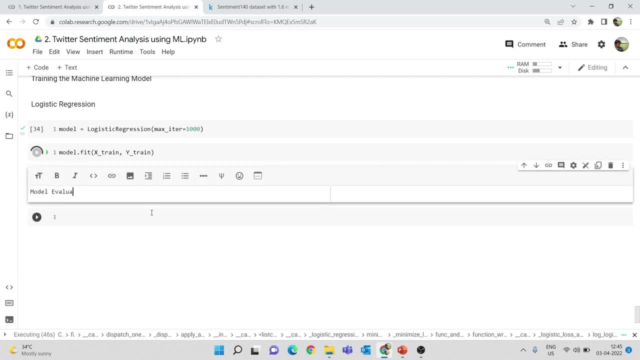 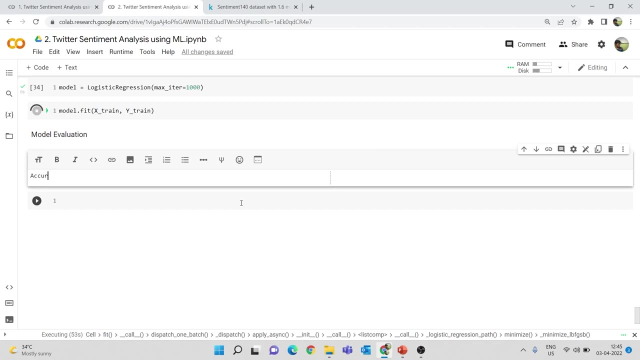 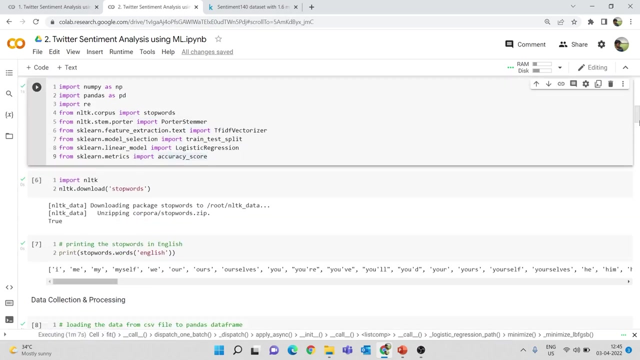 other part of the code, this model evaluation. okay, so for this model evaluation, we are going to use, uh, something called as accuracy score. this accuracy score, if you remember, we have imported this accuracy score function previously from this sklearn dot matrix, so it will calculate, uh, like how many correct predictions are being made by the model. 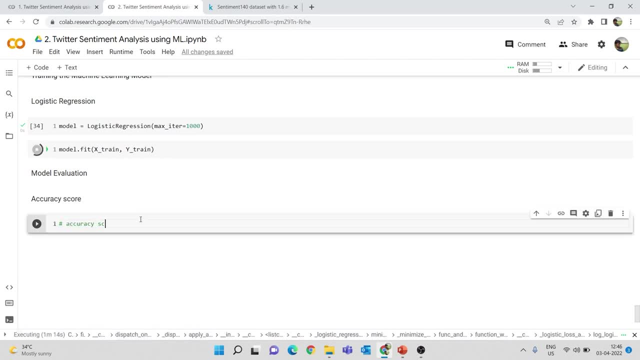 so let me put this as accuracy score on the training data, and i'm going to create a variable called as extreme prediction. okay, so this extreme prediction is equal to model dot predict extreme and this is my training data accuracy. training data accuracy is equal to accuracy score, so this is the function that we have imported. 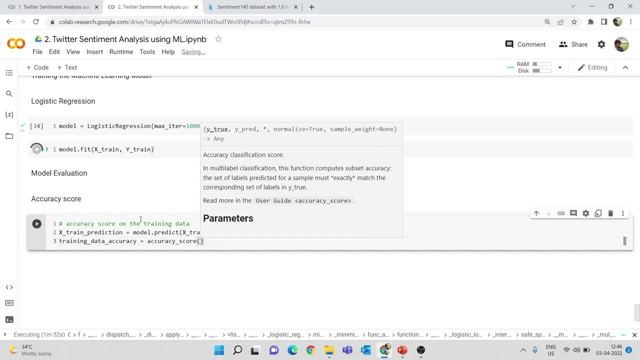 accuracy score. so within this, we have to give the current labels and then the labels predicted by our models- i'm going to say void, train and the extra prediction. okay, so what we are doing here is so, once this model has completed learning from this data, we will make predictions with this extreme itself. so in this case, as you can see previously, we have 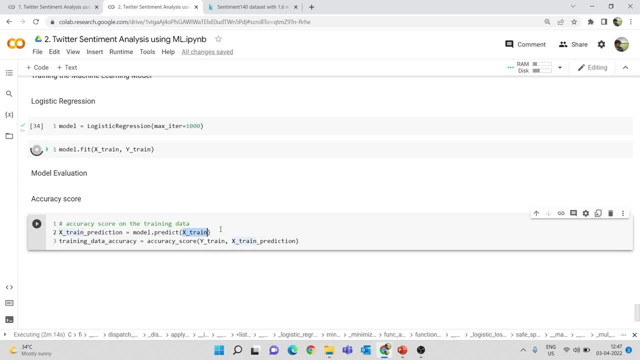 trained our model with the tweets as well as the labels. in this case, we are giving only the tweets. now the model has to find what is the target, whether you know whether the tweet is a positive tweet or a negative way. in kevin's case, we have given it a model that is based on x者. 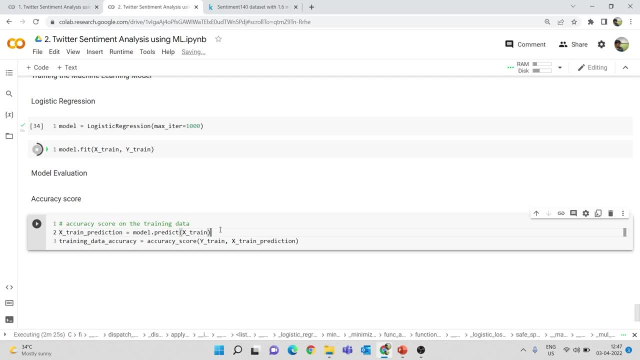 In other words, it will predict the values, a value as either 1 or 0. So these are the values predicted by our model and those are stored in this extreme prediction. Now we have to compare this extreme prediction with our true labels. the true labels are nothing. 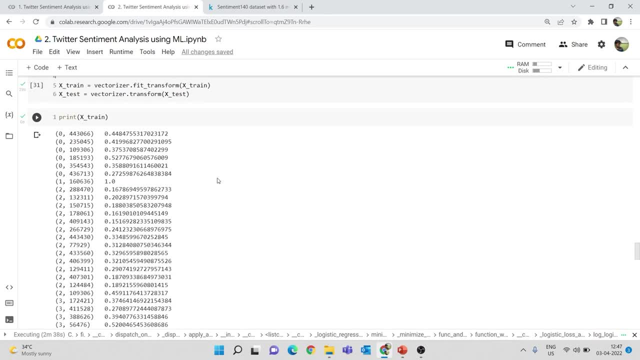 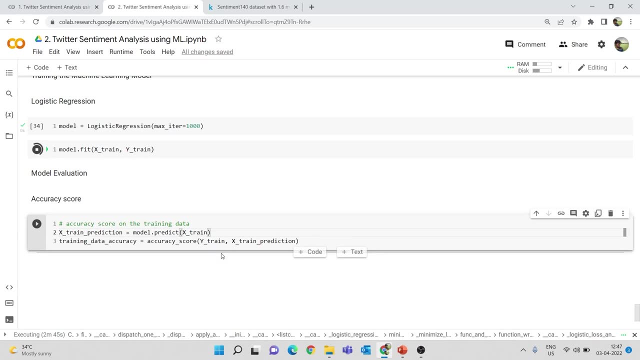 but my white train, that we are splitted here, that we are splitted using this train test split function here. Okay, So we are just comparing the true values and the values predicted by our model. So in this case, the true values, or you can consider this as the ground truth, with the 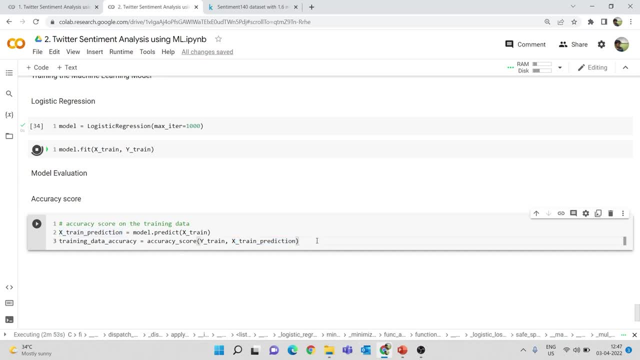 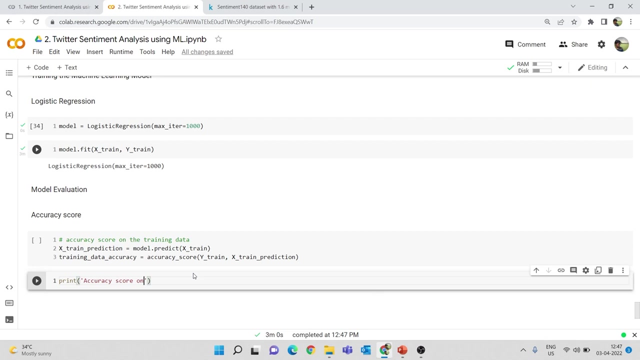 values predicted by our model. So these are the predicted values. when you run this one, you will get this accuracy score and once this is done, I will print this accuracy score as well. So let me put this as print accuracy score on the training data. okay, so accuracy on the 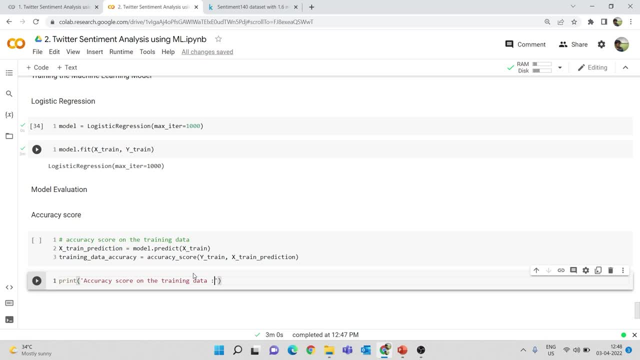 training data is equal to 0.. Training data accuracy: okay, so the model has completed training. so this took about 3 minutes. okay, So I will run this one. so this will predict the training data labels and this will tell me the accuracy score by comparing the true values and the predicted values. okay, and now? 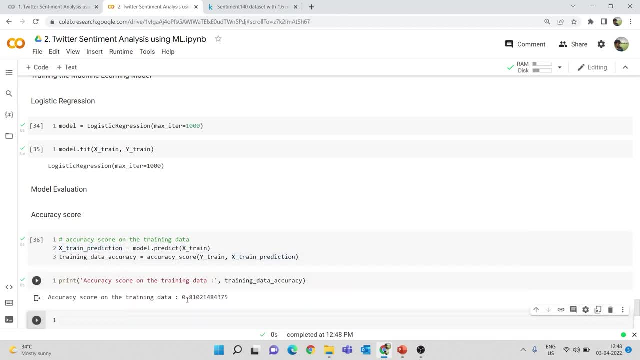 let us print this training data accuracy and let us see this. So the accuracy is 0.8102. so this means like the accuracy score of the model is 81 percent. Okay, So the value won't be represented in percentage, but will be represented between the value. 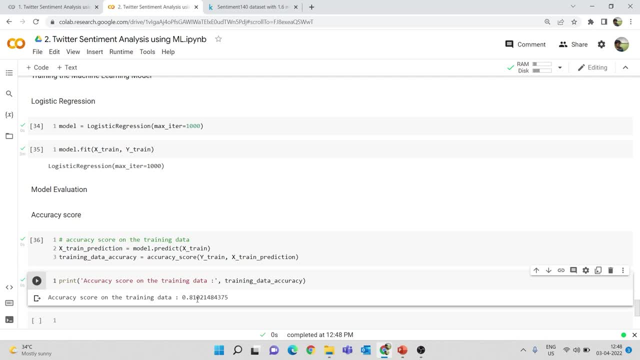 0 to 1.. So if the value is 0.90, that means the model is 90 percentage accurate. in this case, the model is 81 percentage accurate. So what is 81 percentage accuracy means, if let us say that we have trained our model? 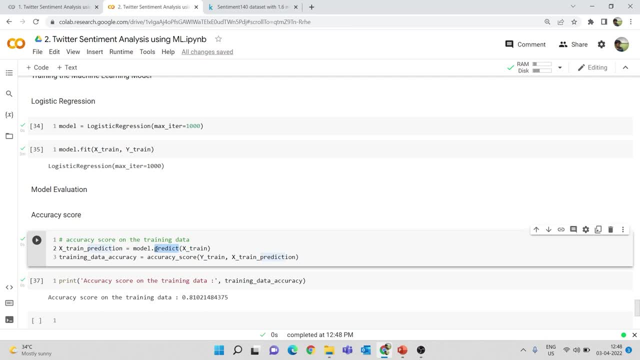 and if you use this model in order to predict new tweet, whether it is a positive tweet or negative tweet, in that case, out of 100 tweets, your model can make correct predictions for 81 tweets, So remaining 19 tweets it can predict wrongly. so that is what is meant by this accuracy. 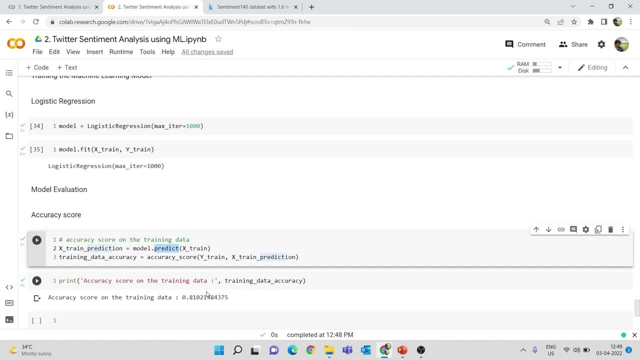 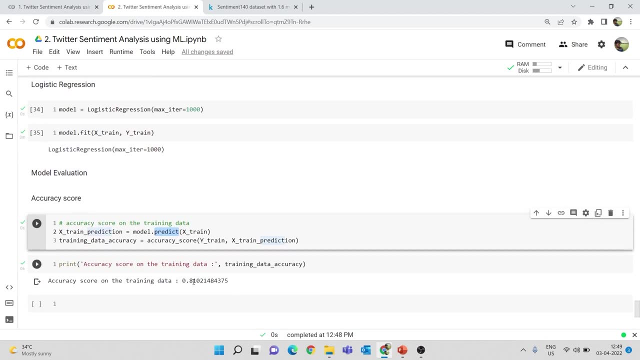 score. okay. So if the accuracy score is 95, that means like, out of 100 tweets, it can make correct predictions for 95 tweets. So this is what accuracy score means, okay, So this is like, instead of being in the range of 100, like you know, 80 percentage or 90 percentage. 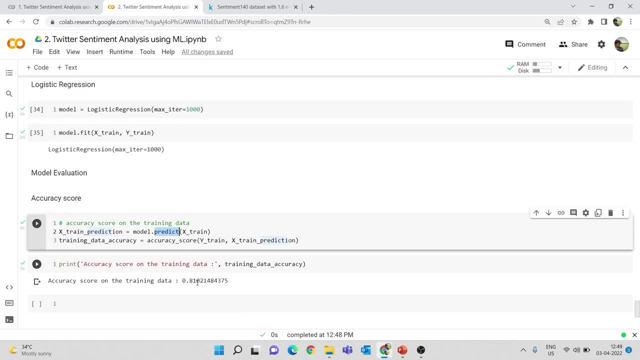 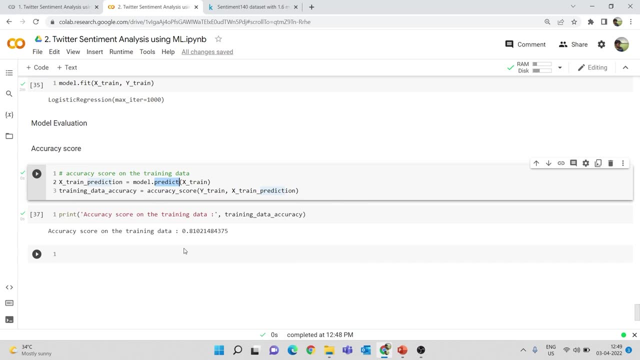 we are getting the values in values between 0 to 1.. So 81 means 0.81, means like 81 percentage, and so on. okay, So this is the accuracy score on training data, But this is not sufficient. we have to calculate the accuracy score on the test data. the reason: 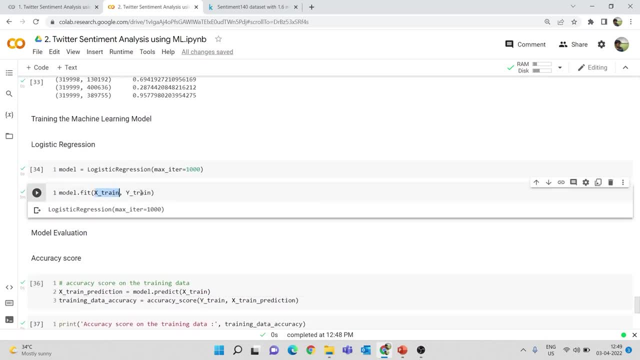 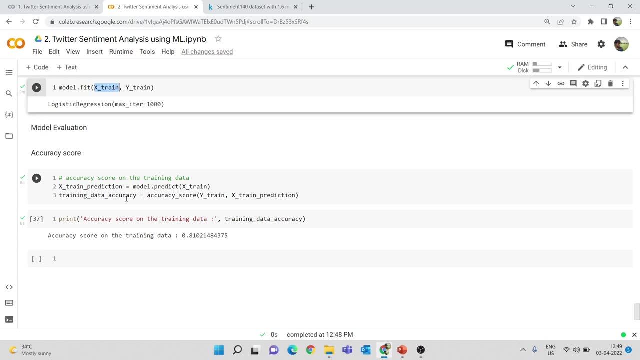 is, the model has been trained on this X-train itself, so it kind of knows how the training data looks like. but it does not see the you know test data before. so we have not shown the test data to the model right. so we have to check the accuracy score on test data, which 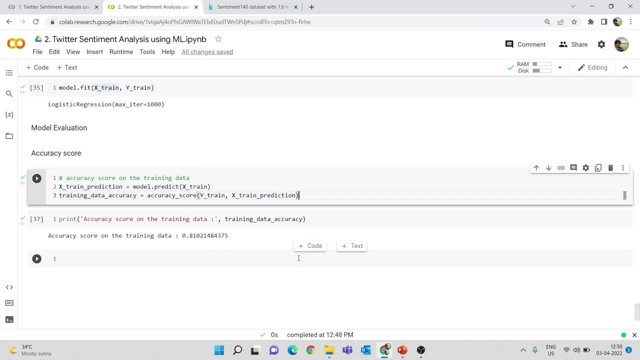 is very important, So I will copy this one and change this accuracy score on the training data to test data. So here I am going to change this X-train to X-test predictions. So here I am giving only the X-test and this will be my test data accuracy. so I am converting. 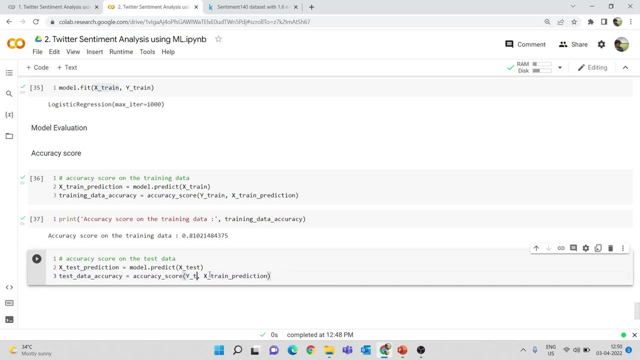 all this training to test. So this Y-train has to be replaced by Y-test. so this X-train should be replaced with X-test. okay, and then we will print this test data accuracy as well. let us see what is the accuracy of X data. okay, let us run this one. 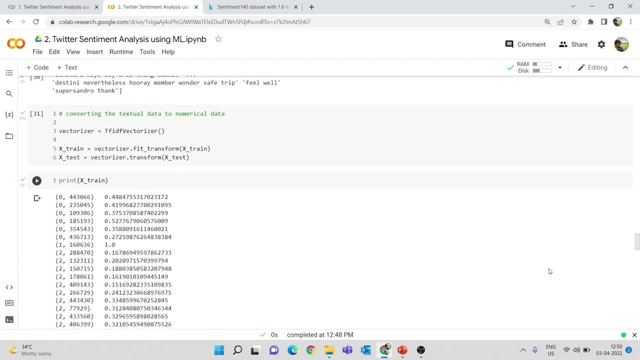 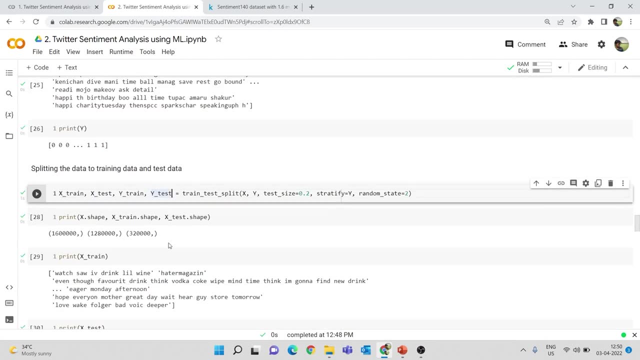 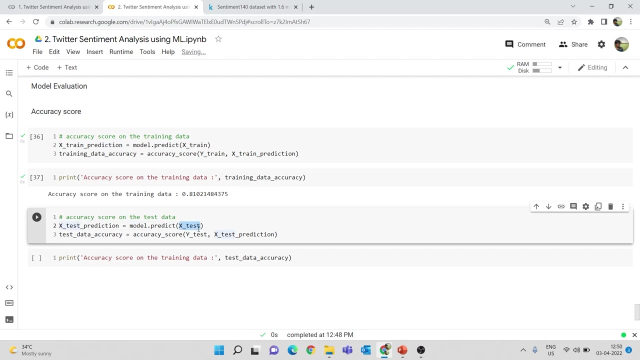 So X-test prediction model. So, as you can see, we have performed this X-test split, this train test split, and X-test is made test data and Y-test is the labels for it. in this case, if you see, here we are using the model to predict the labels for the test data and after that we are comparing this. 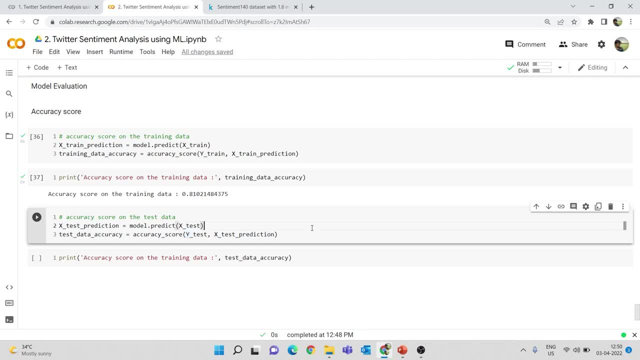 test data prediction with the true test labels, which is Y-test. okay, so I will run this one and let us print this accuracy score: and the test data accuracy is 0.778, which means the test data accuracy is 78.7.. Okay, As we can see, the training data accuracy and the test data accuracy is very close to each. 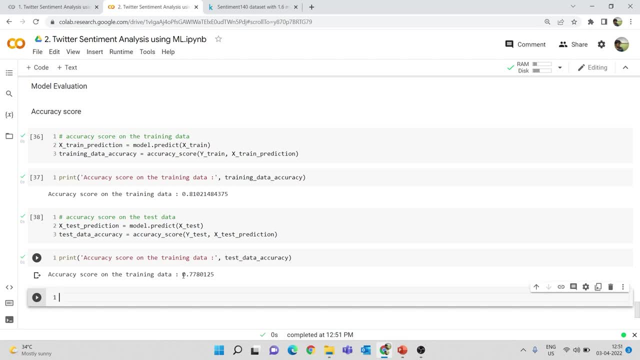 other. so in this case we can see that the model has performed well. so there are cases which we call as overfitting, when the training data accuracy will be more whereas the test data accuracy will be very less. say, for example, if the training data accuracy is 81%, the test 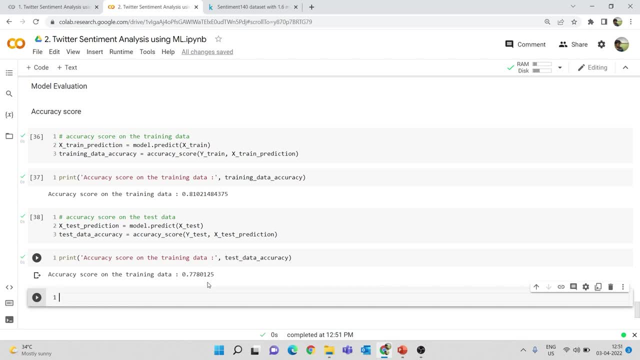 data accuracy will be like 40% or 50%. so that is what we call as overfitting. so overfitting means the model has not learned properly, okay, so this is why it is important to you know. check the accuracy for test data as well. so just convert this to test, okay. so the reason. 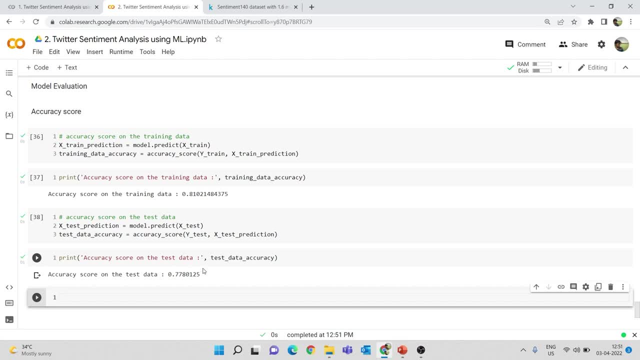 we are, you know, calculating this test. data accuracy as well is. so let us consider this example. let us say that you are studying for your max exam and you are practicing. let us say 100 questions or 100 mathematical problems, and you are just writing a test by yourself. 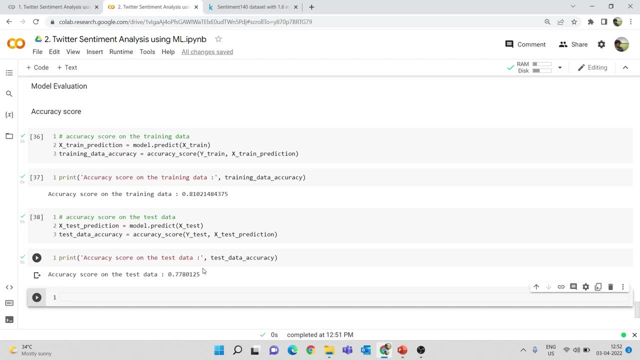 with this 100 problem. so you will get a score. as you have already seen this questions, you will get a good score. and let us say that there is an examination and in the examination they not only ask the question that you prepared, but they will ask different questions based 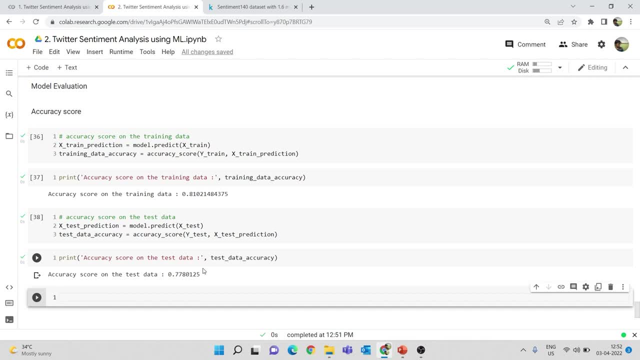 on that particular concepts. if you have prepared well, you should answer those questions correctly as well. right? so it is similar to it. so training data is like the data on which the model has studied, so it is like the questions that you have practiced, and test data is like the questions. 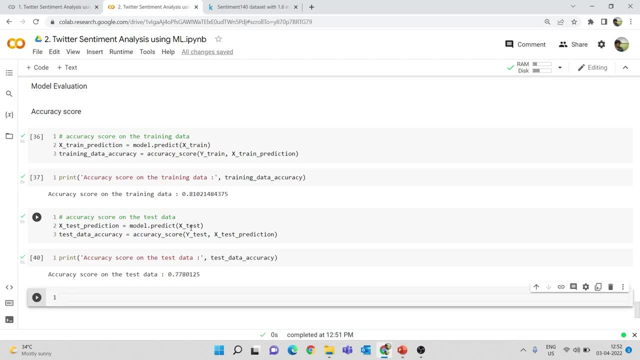 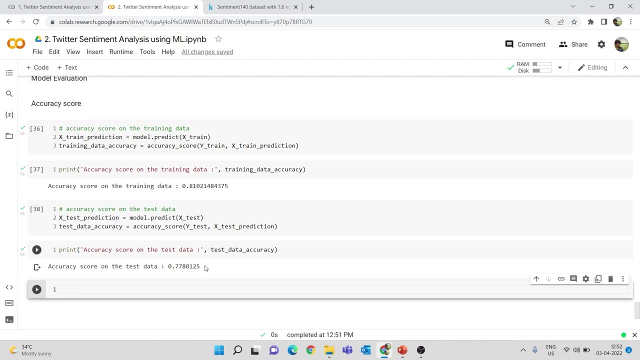 that you do not know. so those are like questions that are said by the questioner, but these are like the same concept. you know it is similar to the concept that you have prepared, so the this is why the accuracy score on the test data is important, the reason being the model. 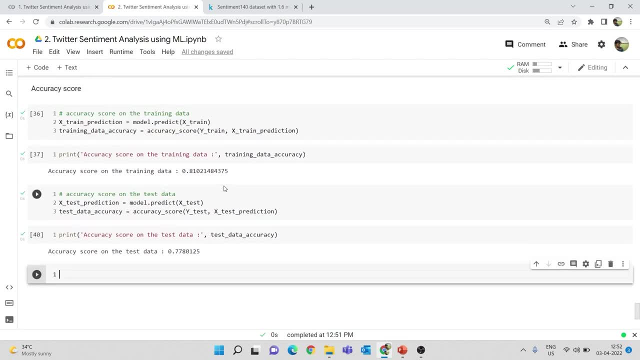 has already seen the training data. so that is why we, kind of you know, use this test data accuracy as the final one. so we do not consider this training data accuracy, but we have to calculate both of these things in order to see whether the model has over fitted where 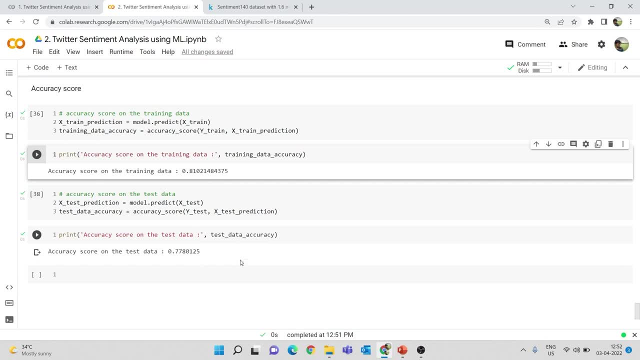 overfitting has happened. that means, like the training data accuracy will be very high and the test data accuracy will be very low. so let me put this as model accuracy. so this is like models. test data accuracy is equal to 77.8 percentage, so 77.8 is the accuracy. 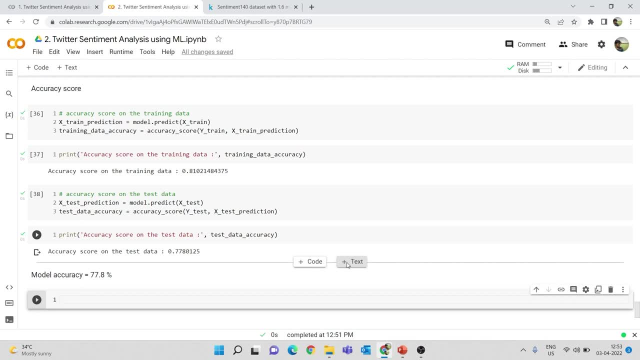 of the test data accuracy like 77, which is almost equal to 80 percentage, is actually a good accuracy score. if the accuracy is greater than 75 percentage, we say that it is a good model. and there are also like techniques, like grid search, cv and randomized cv, what we call as hyper parameter tuning. so if we get a 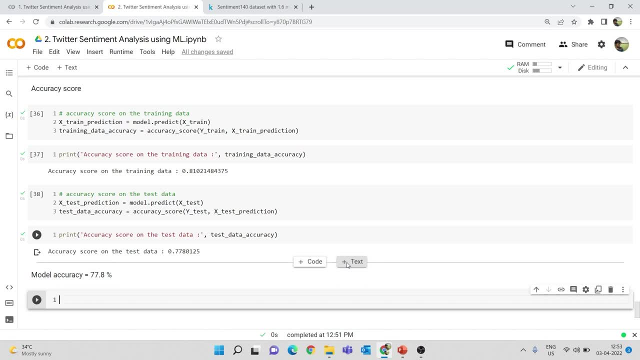 low accuracy. we kind of perform all those things in order to increase accuracy, but let's not go into that in today's video. so it's kind of like deviating from this concept of tweeters and tuned analysis. so we will discuss about this hyper parameter tuning in a later video, okay, so 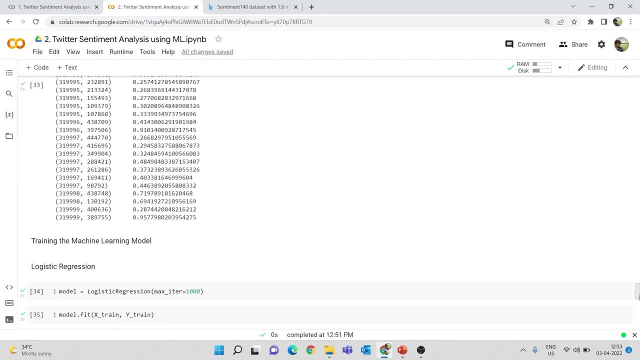 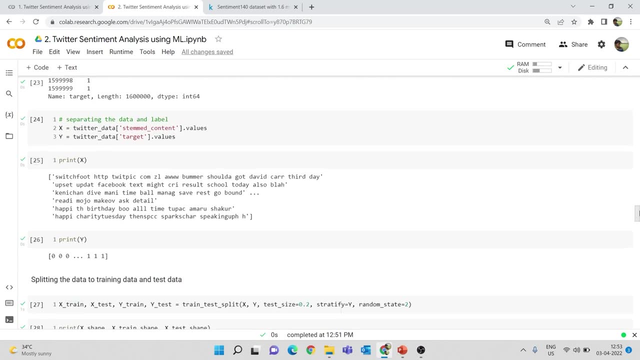 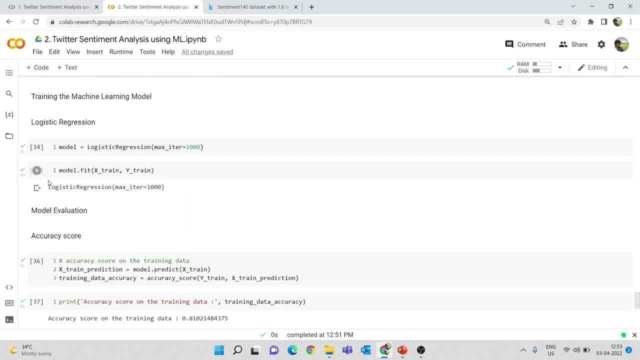 i'll just show you how you can save this model. so we have done all these processings right. so from like importing the data set, processing it and training the model and so on, which took a very long time, now i'll show you how you can save this trained model, which is my model, so modelfit, so 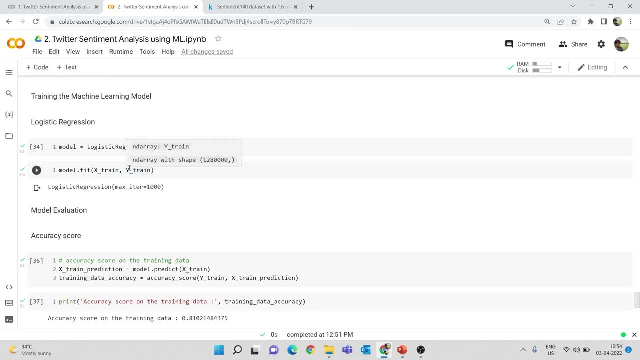 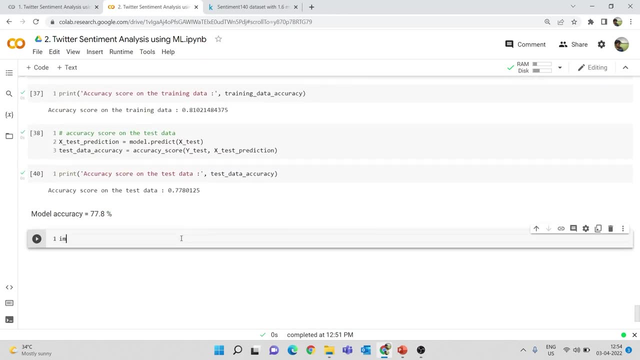 this model is not right, so i'll show you how you can save this model and how you can use this saved model afterwards without doing any of this training and data processing and all those things. okay, so for this i just going to import a library called as pickle. so pickle is the library which kind of 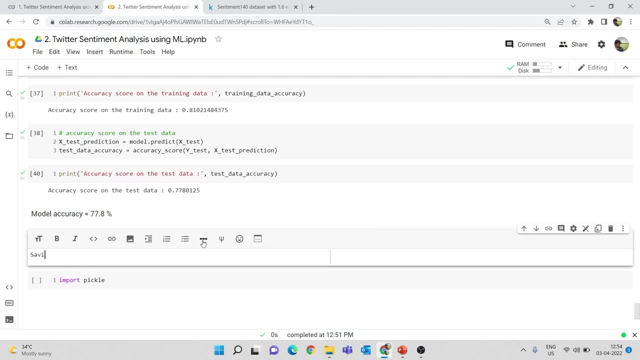 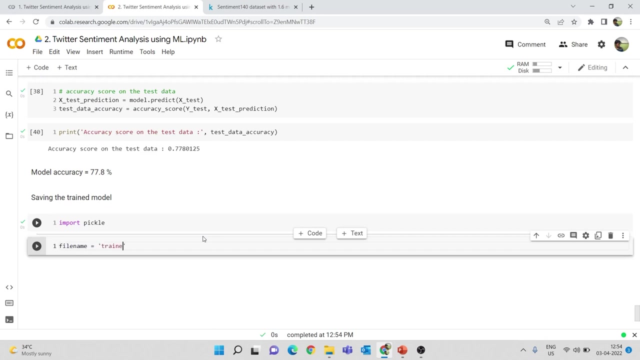 exists for this and i'll put a text here as saving the trained model. okay, yeah, so i'm importing this pickle library and i'm going to create the file name. so file name is equal to- let's call this as trained model dot sav. so i'm using the 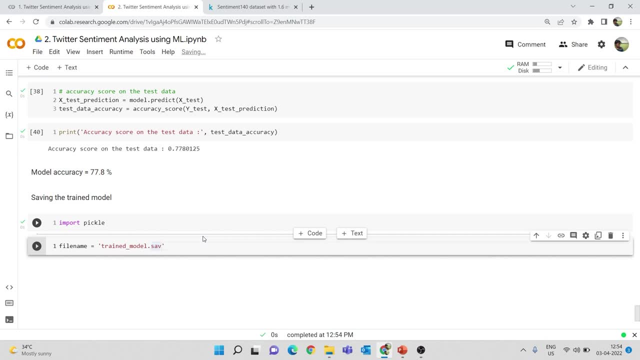 extension sav, which is like some saved file. you can also use the extension pkl, which means like avenue, pklfile. so like both are. you know, we can do any one of those things. so i'm going to say pickle, so pickle is nothing by the library that i imported dot dump. 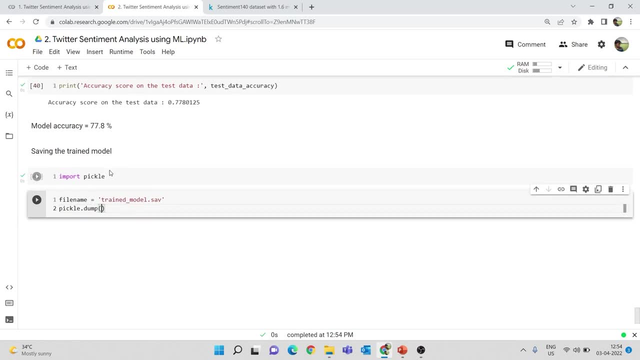 so when i say this, dump all the parameters, all the things that is learned by the model will be stored in this. i'm going to say model comma, open file name and file name from a wb. so what i'm doing here is using pickle and dumping it. so i'm dumping the model starting from pkl file name. so here i'm. 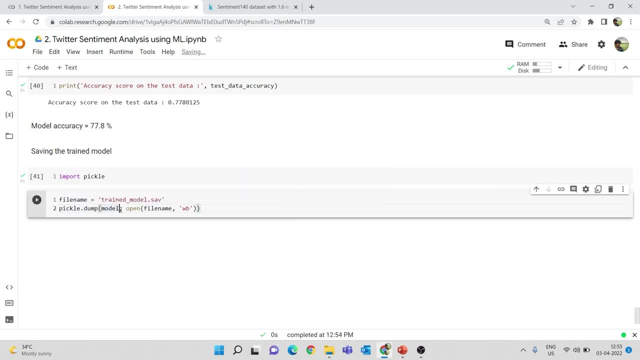 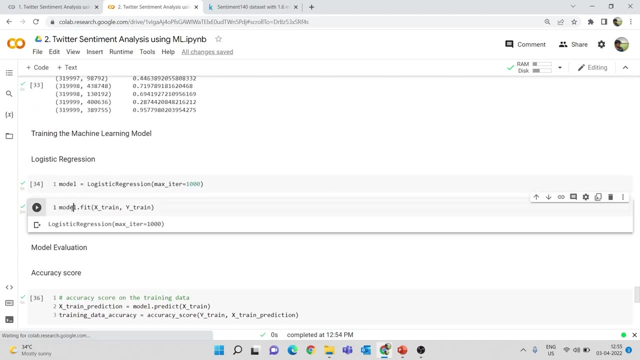 using pickle and dumping it. so I'm dumping the model, which means I'm storing all the parameters and the learnings of the model. so that is where I mentioned model. so this model is nothing but the model that we have created. so if you have used another variable called as classifier in that, 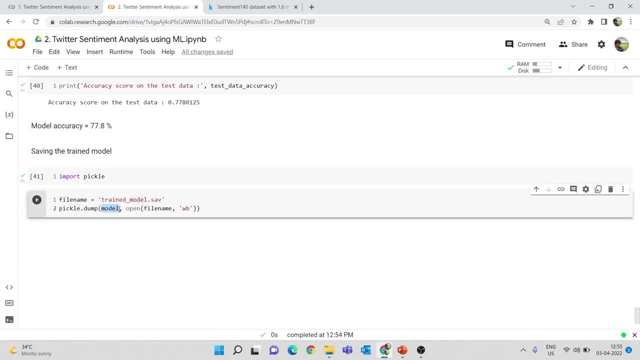 case, you will replace this model by classifier. so this is the name of the model that you are storing. and how we are storing is we are opening a file and open file name. so file name is nothing but the name of the file that we have created, which is train model dot SCAV. so WB means we are going to write a. 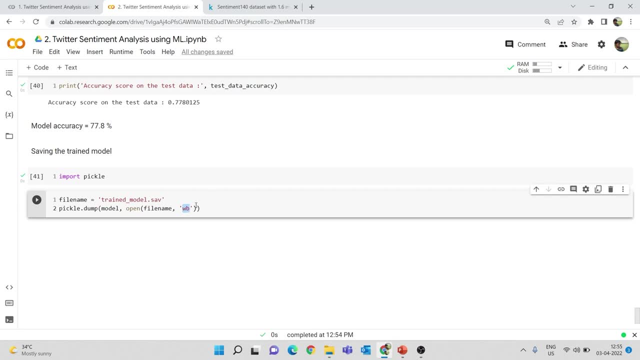 file. so we are going to create a new file and we are going to write something. so what we are going to write is this model, so the saved model. if you mentioned R, that means we are just going to read something. we are not going to edit it. so 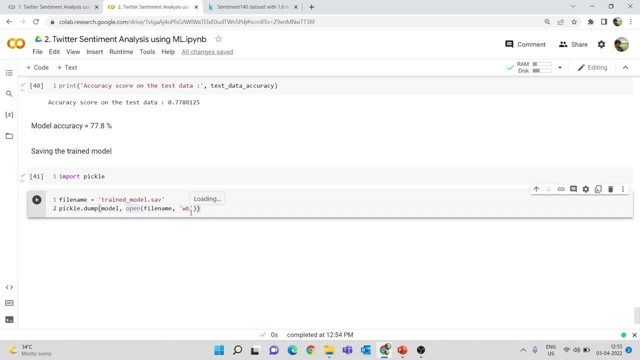 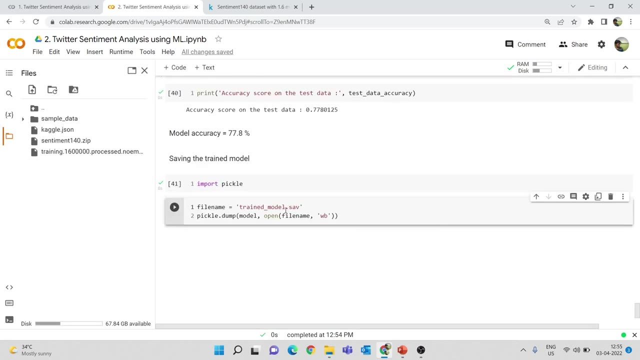 this is like editing or writing it. B means we are writing this in the form of binary format. okay, so this will save my model. so if you see this files, there is no files called as train underscore model dot SCAV here. right, so I'll reference this. there is no files like this. when I run this one, this model will. 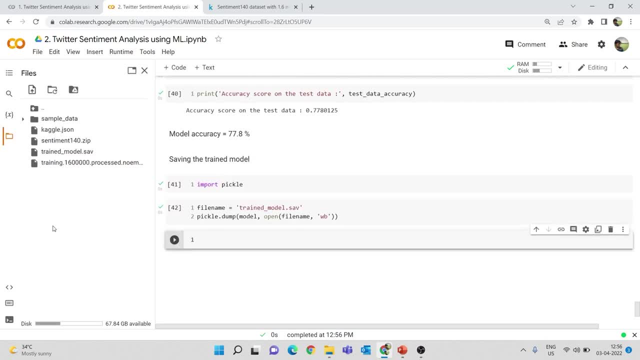 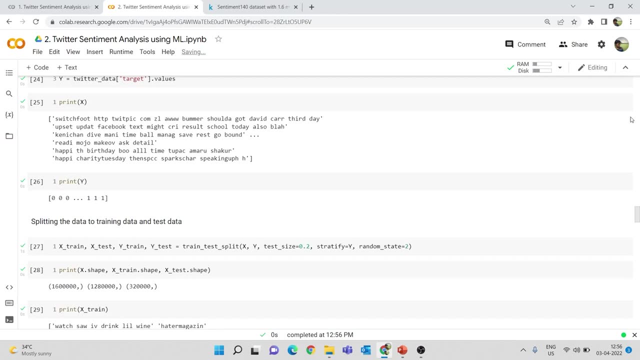 be stored. okay, so if you go here, okay, so if you go here, so this model has been stored and this model size is very small, which is like 3.5 to MB. so all the things that you have done, so you have, like, got the data. 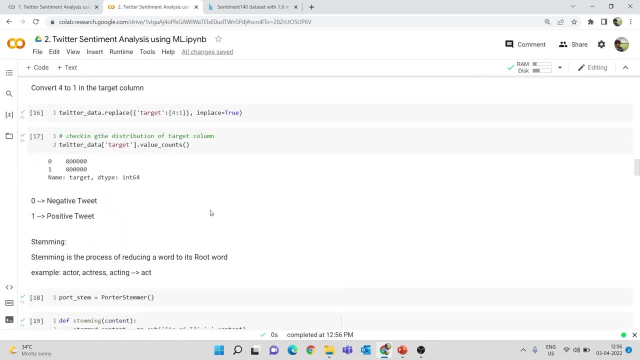 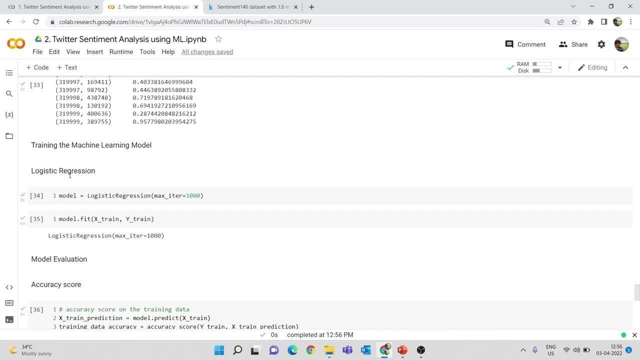 using the C API. you have done all this tough processing, all those things and you have trained your model right. so all this learning of this model- learning in the sense they are stored in the form of parameters of this logistic regression model. they have been stored in this file, so you don't need to train this model. 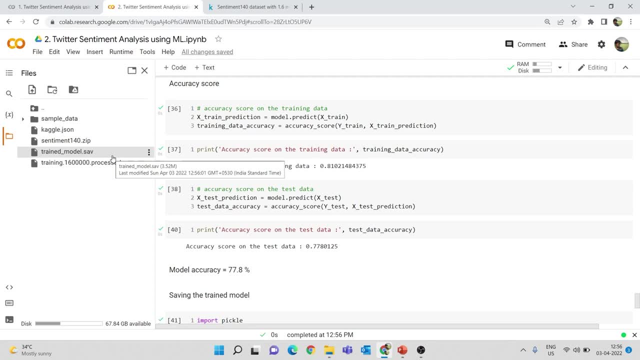 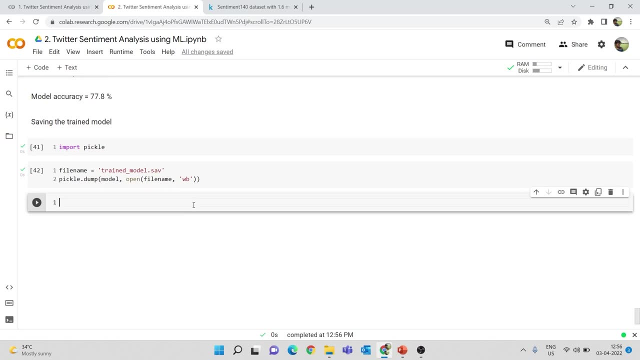 again in order to make this prediction. so you can use this trained model itself in order to make new predictions, okay, so this is how you kind of save a model that you have trained with some data set. now I'll show you how you can use this model for new predictions, okay, so first, as we have you know, return a file, right? 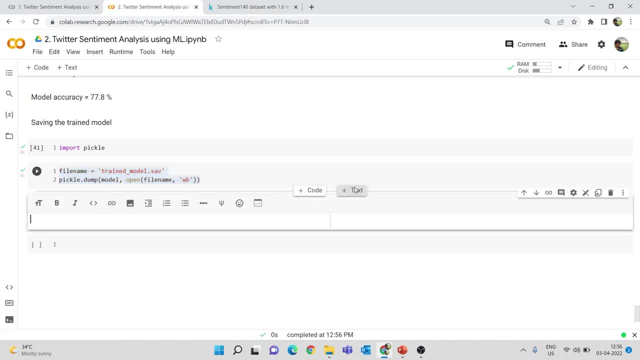 now we have to load this saved model. so this part is using for future predictions. So for this, first we have to load this model. so I am making a comment here as loading the saved model. okay, so loading the saved model. so I will create a variable as loaded model. 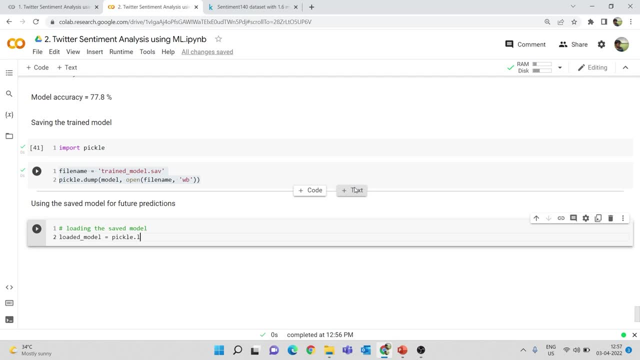 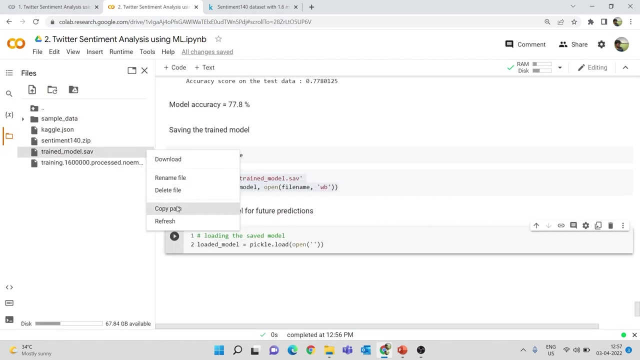 Loaded model is equal to pickle dot load. so for saving the model we have to use this pickle dot dump. for loading this saved model we have to use pickle dot load. so in this we have to say open trained model csv, or we have just have to copy the path of this model. 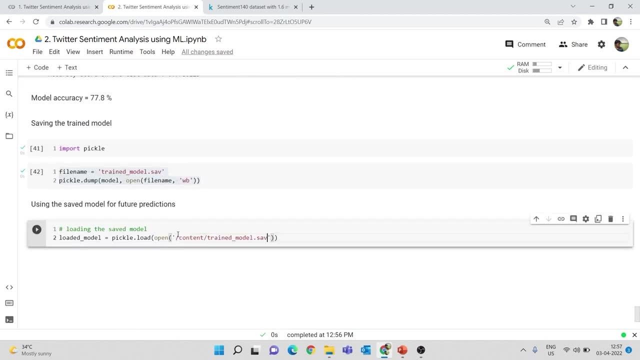 that we have created. So I will copy the trained model sav path. paste it here. and here we have to read this file, so you should not mention this as wb. you have to mention this as rb. rb means we are reading the file, whereas w means we are writing this file, so here we are not writing. 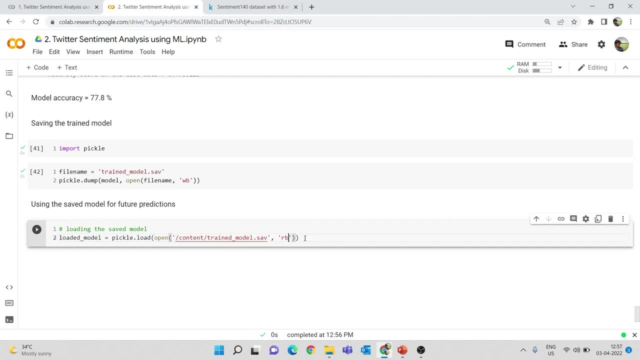 anything. we are reading the file, or we are just extracting this trained model, and again, we are reading this in the binary format. So I will run this one. So now the model that we have saved will be loaded to this variable called as loaded model, and now we can use this in order to make new predictions. 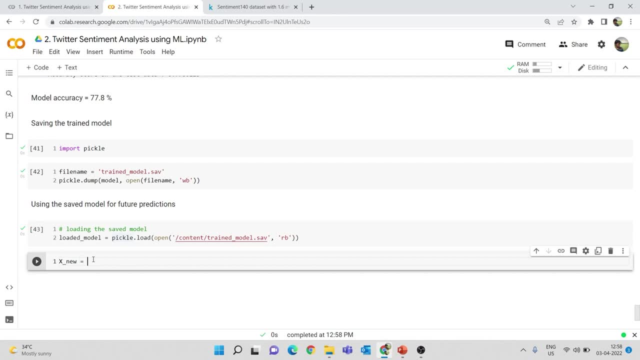 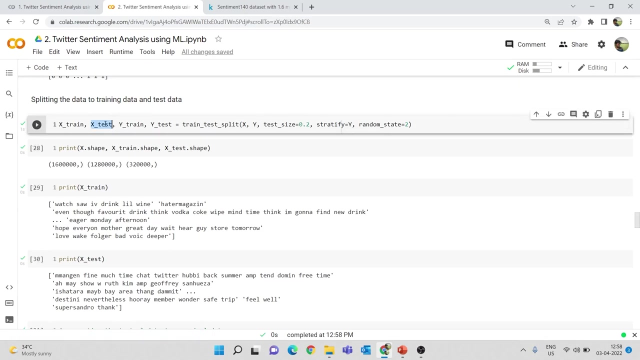 So I will say x new is equal to x test, x test of, let us say, 200, so x test of 200 is nothing. but so we have this trained test bit. so in this trained test bit we have this x test, which is my test data. so these are the data that the model has not seen before. 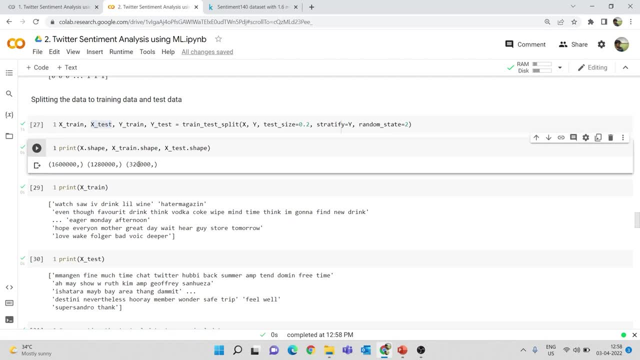 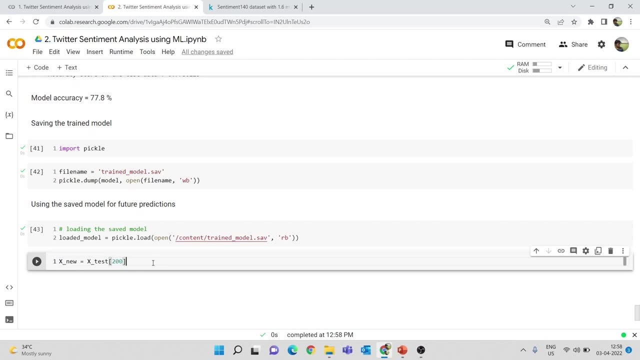 and this test data has about like 3,20,000 data points. Okay, From this I am going to print the you know 200th data point and the corresponding label has been stored in y test, right, yeah, so let me print this y test as well. y test of. 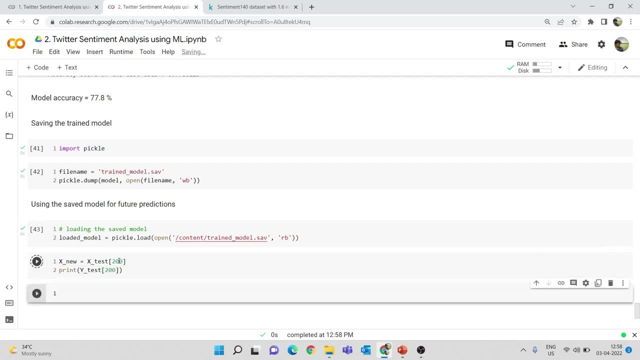 200,. okay, so this is my 200th tweet in my test data and the label is 1, so when I use my model for this x test, it should predict the same label as 1, let us see whether it is doing it okay. 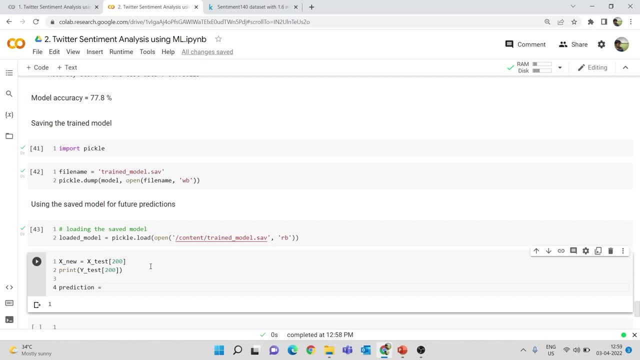 I am going to say prediction, so this is where I am going to save my new prediction. so prediction is equal to modelpredict x new. so x new is nothing but that one single data point for which we are going to do the prediction. 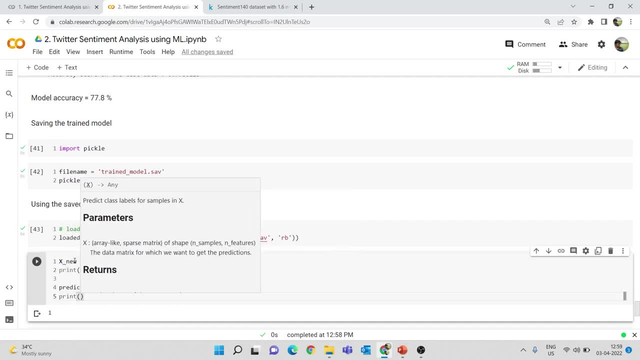 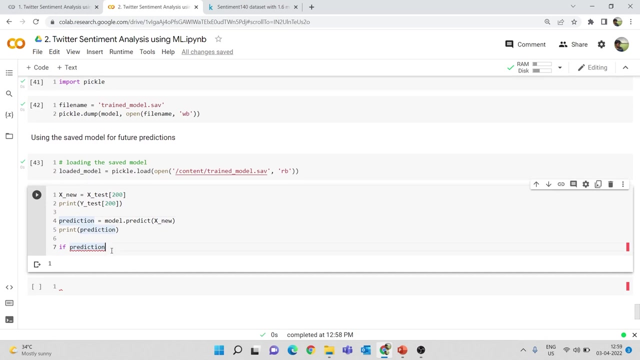 So x new, I am going to print the prediction so it will print whether the value is either 0 or 1, so print prediction and if this prediction, I am creating an if else condition here to print whether it is a positive tweet or a negative tweet. so I am going to say, if this: 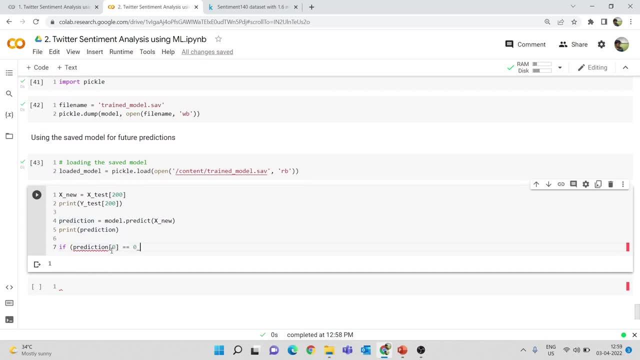 prediction of 0 is equal to 0, in that case, I have to say that I have to print: it is a negative tweet, so we know that if the label is 0, it means negative tweet, right? so negative tweet, okay. negative tweet, yes. 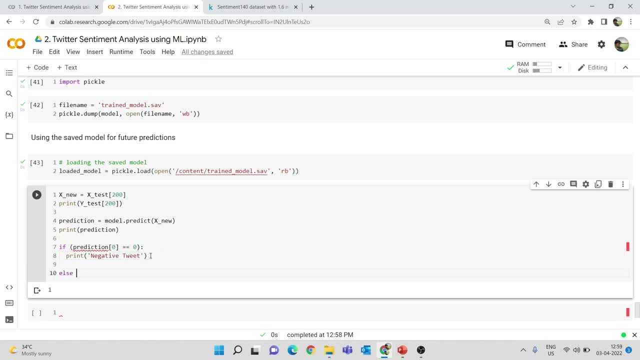 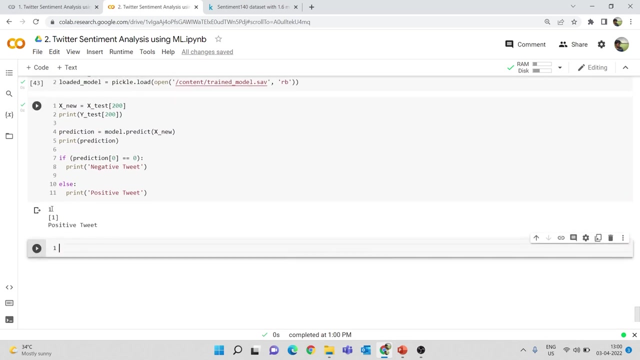 Okay, Yes, Yes. So the prediction is kind of, you know, if the value is 1, in that case we have to print that it is a positive tweet. okay, let us run this one okay here. the first one is: 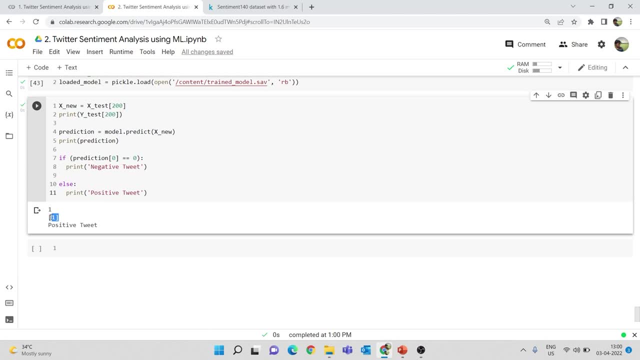 the true label. so, as you can see, y test of 200, this one which is in the square bracket is the value predicted by our model, which we have stored in this prediction. so this print prediction will give you the result like this, and if the value is 1, we have to. 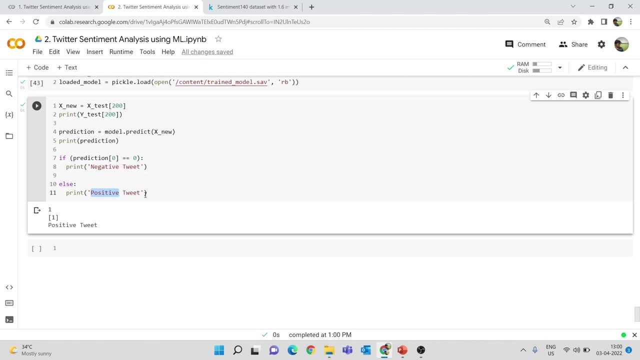 say it is a positive tweet, Because we know that if 0, it means a negative tweet. if 1, it means positive tweet. right, so that is what we are doing here. the reason we are mentioning the square bracket here is the result of this prediction, the result of this modelpredict, or I can also use this: 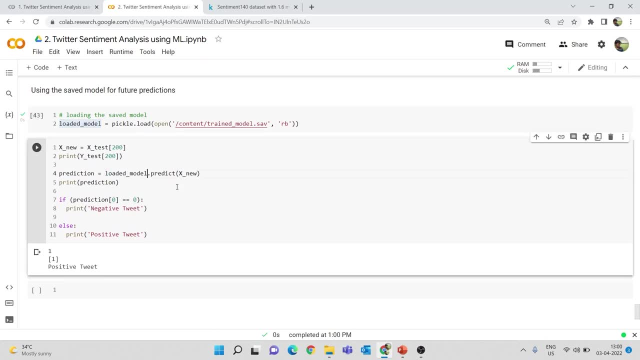 loaded model. so, instead of you know, using the model that we have trained. so this is the saved model. so they are actually the same thing, because we are just loading the same model here. so the result of this model, or this prediction, will be stored in a list. 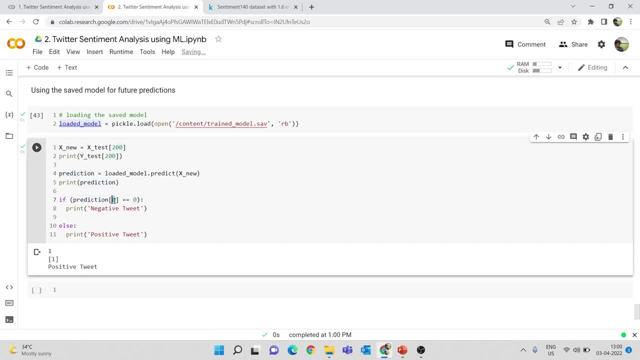 so this is a list with one value. so when I say prediction of 0,, that means it is the first value within this prediction. So when I say when the first value of this prediction is 0,, I have to say negative tweet. 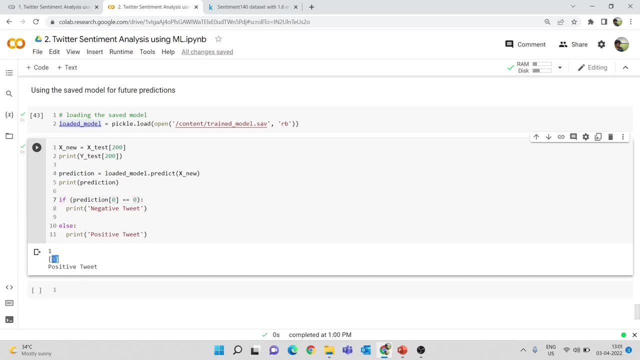 if not, I have to say it is a positive tweet. so in this case the value is not equal to 0, right, if it is 0, it would have shown it as negative tweet if the value is 1, it. 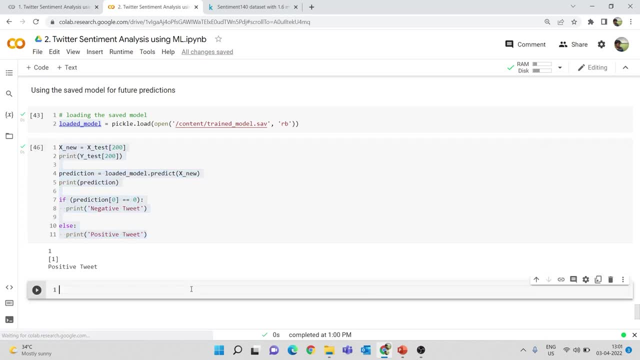 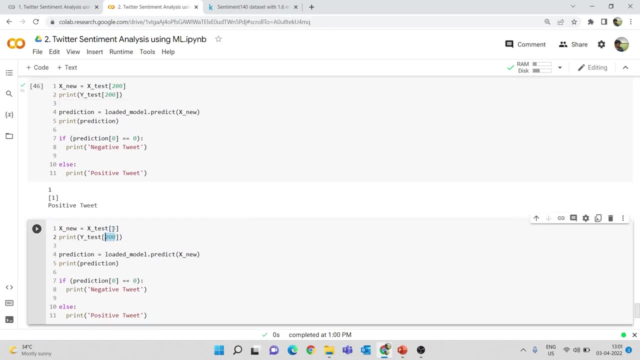 is showing this as positive tweet, so I will copy this one. I will just paste it here, but now I will use a different value, so I am going to say a different index, which is 3,. let us see what is the index and like whether it is a positive tweet or a negative tweet. 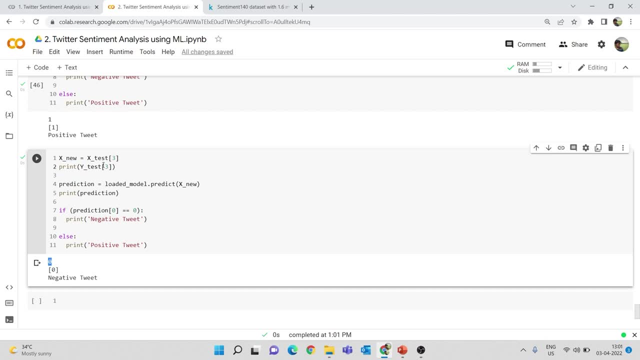 so this is my true value, which is 0.. Which I have printed using this ytest of 3 and I am comparing it with the value predicted by my model. so my model, I have predicted the value as 0, so it has predicted correctly. 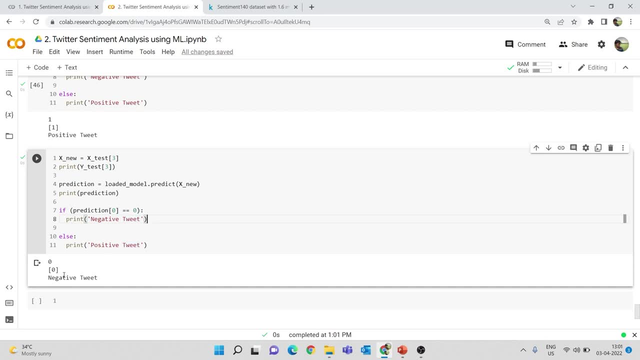 and if the value is 0, we have to say it is a negative tweet. so here: what we are doing here is like we are checking whether the model is predicting correctly. so you do not have to print this, but I am printing this to check whether the model is predicting correctly. 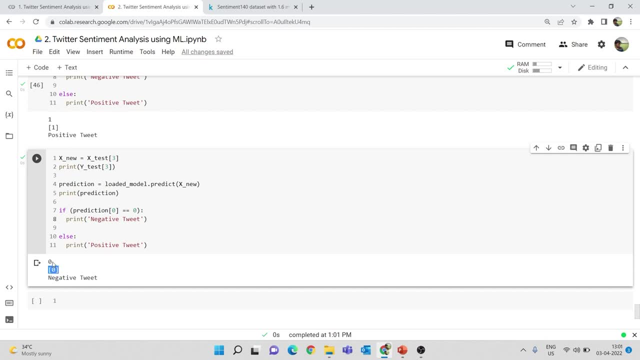 if the model has predicted 1 in this case, then it is a wrong prediction, because the true value is 0, but the model is predicting 1, whereas in this case it is predicting both the values as the same. So it means like the model is making a prediction. 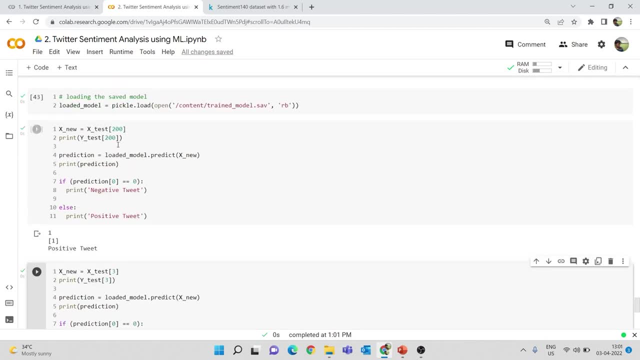 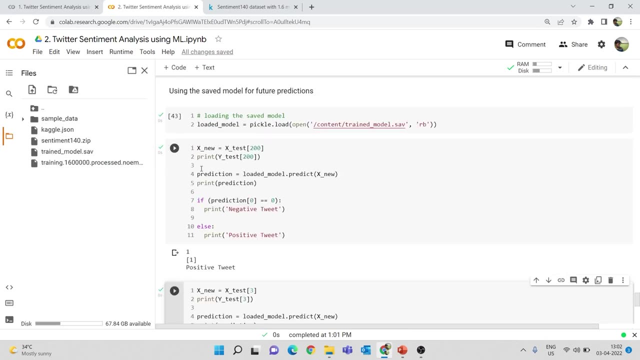 So this is how you can use the saved model. so, instead of doing all those processing, so once you complete this, once you do not have to do this again, so you can save this model, you can download this and you can also run this in your spider or Python and you. 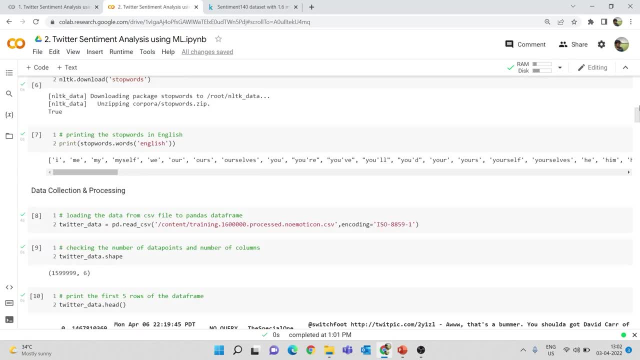 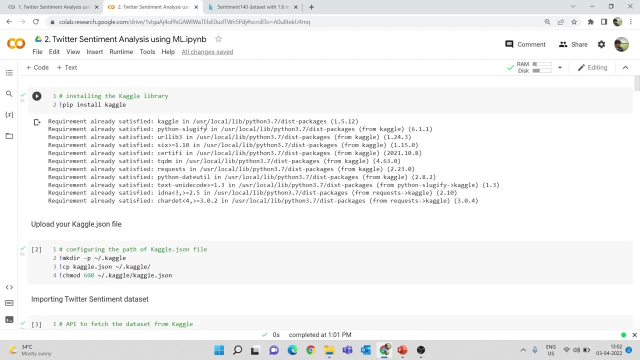 can make these predictions like this, and this is how we kind of do this. So I hope you have understood all the things covered in this one. so I will just give you a quick recap of all the things that we have done here so that you understand what are. 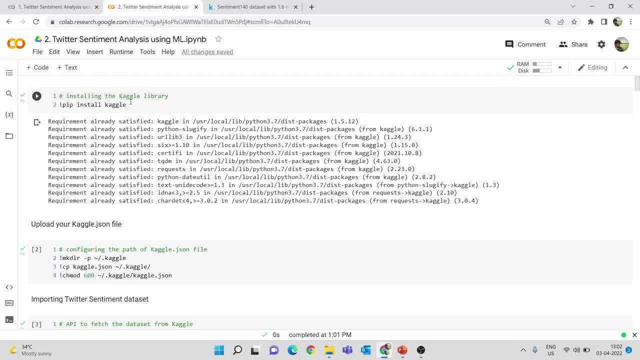 all the processes that happens here. The first thing is installing the Kaggle library. the purpose of this is to use the API- the API- in order to extract the data directly from this Kaggle site. so we have like installed this Kaggle library. so we have seen that it is already pre-installed. so this is like. 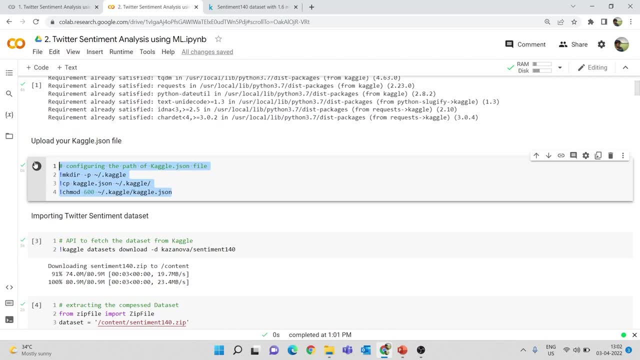 a standard code that we have to use, so you do not have to change anything. so after, like, installing Kaggle library, we have to upload this Kagglejson which we have got from this Kaggle account, which I have shown you, where we create this new API token and so on. 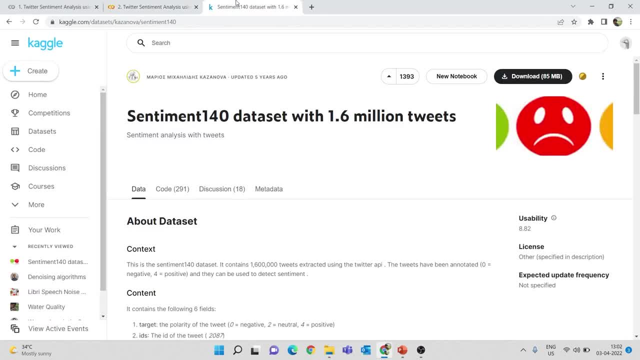 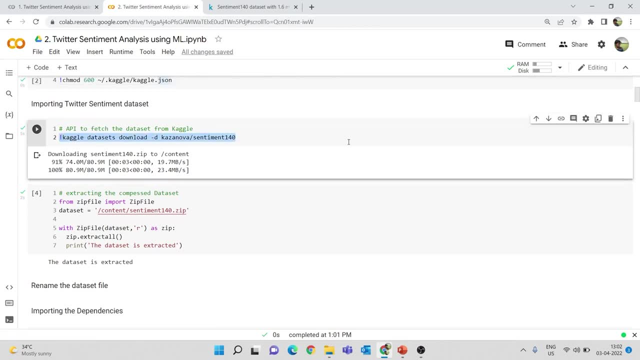 After that we have to configure the path. later we have to copy this API command and the API command is present in this option. copy API command and it will copy this API. so this is my API command. it will load the data directly from the Kaggle to this Collab. 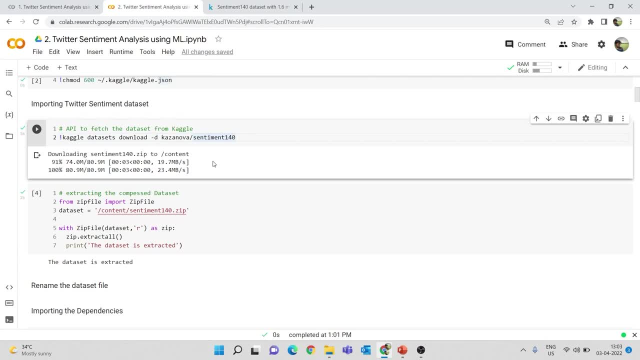 environment. so if the dataset file is small, like 10 MB or 20 MB, in that case we can download. if it is like large, like you know, 1 GB or 2 GB or 10 GB, in that case it is always advisable. 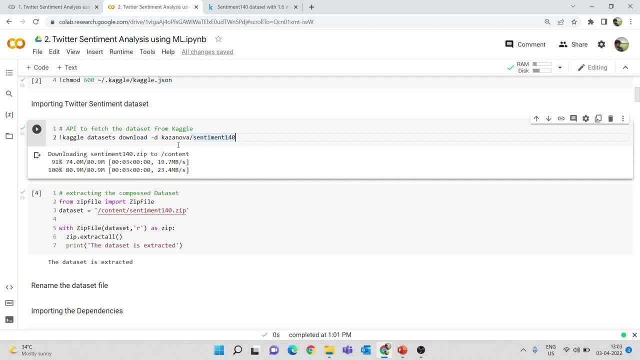 in order to use this API instead of downloading it, so that it kind of happens quickly and no expenses- like no data expenses- will be from our end, so this will happens automatically through this API. so like this 20 MB or this 1 GB, whatever the size of this data is, so 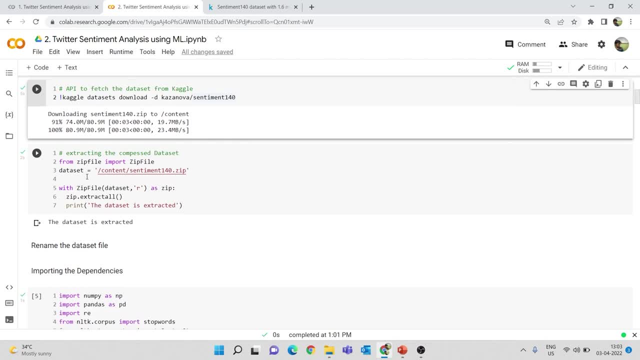 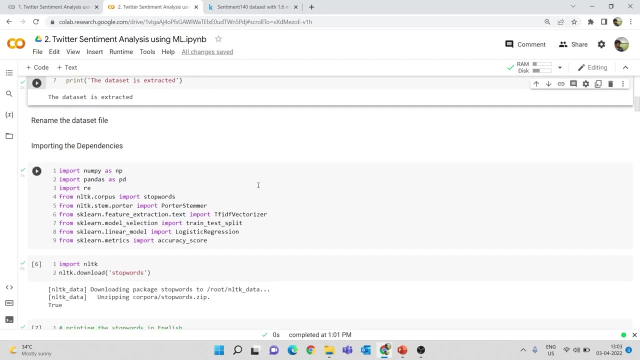 this is not detected from your particular data package, so that is other advantage. and then we know that this is stored in the form of a zip file. so we are extracting the sentiment 140.zip and after that we are importing the dependencies. so we have various libraries. 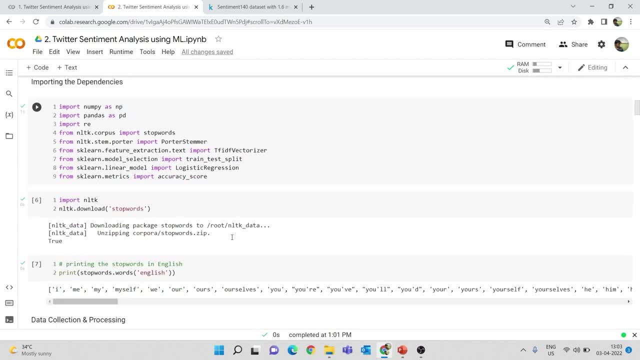 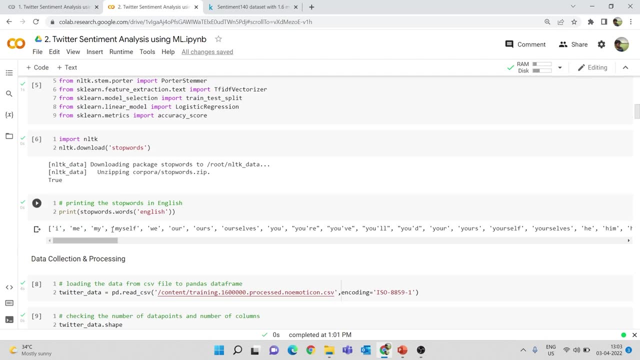 like NumPy Pandas, regular expression etc. So once we have imported all these things, we are downloading this stop words. so stop words are those things that does not have that much contextual importance to the tweets. after that we are loading the data from the CSV file to a Pandas data frame and we have 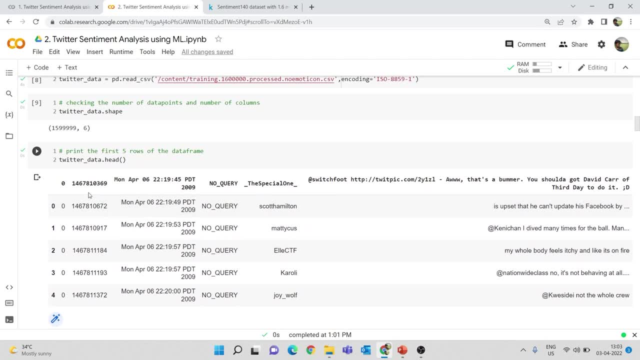 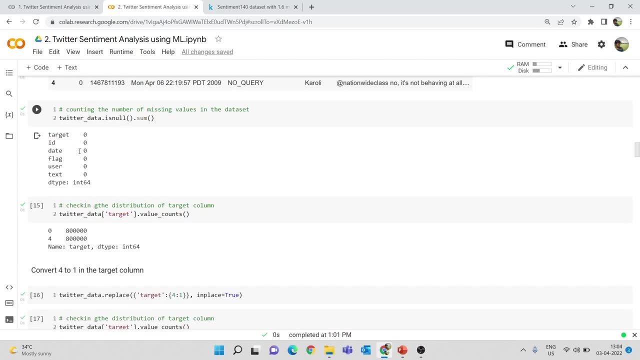 seen like there are totally 1.6 million tweet. but the problem is it is not reading the column name. so we are creating the column names and then we are loading the data frame again, and then we are checking the shape, and then we are checking whether there are any missing values using the seasonal.